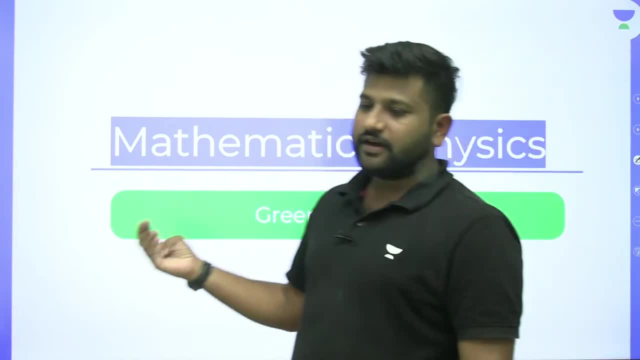 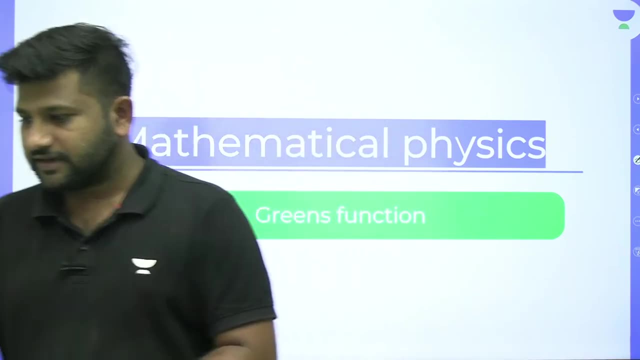 Okay, Let's go. So tomorrow also, two sessions are going to happen In which I am going to discuss CSIR's practice precautions. Good evening, Mr Malaya. Good evening All of you shared it, etc. 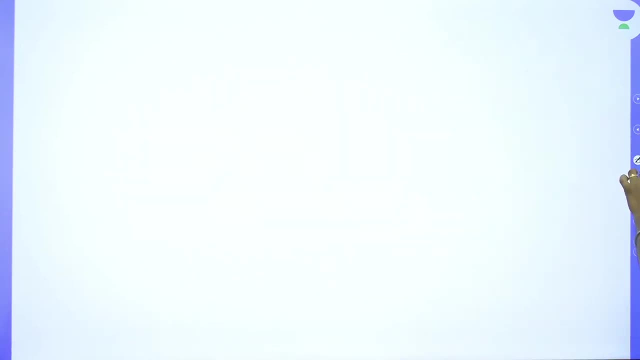 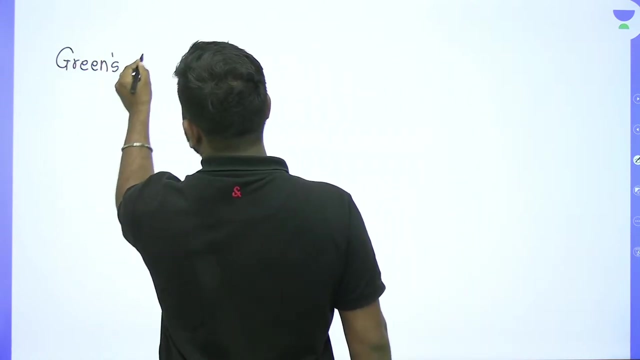 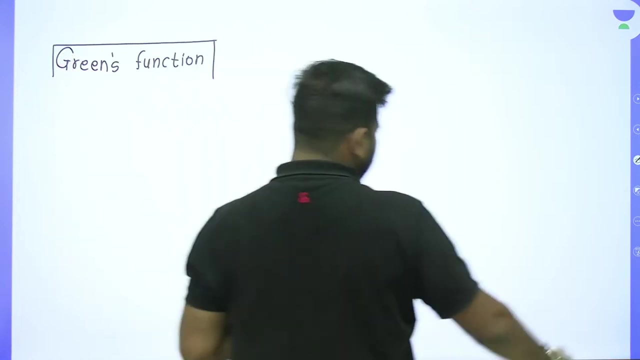 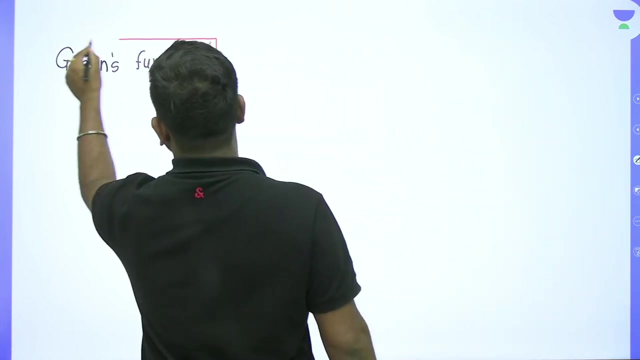 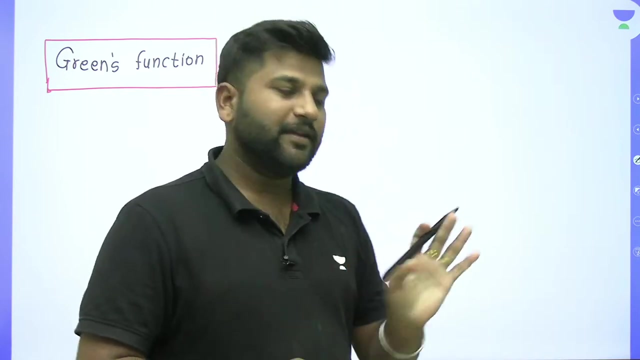 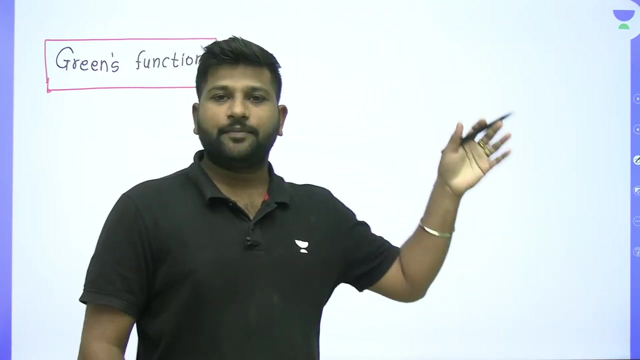 Let's start. So today we are going to discuss. So we are going to discuss about the greens function and this topic is an easy topic. see this: greens function. there are many ways to find out the greens function and their method method is also a long procedure method, but I will tell you how you can find out the answer. 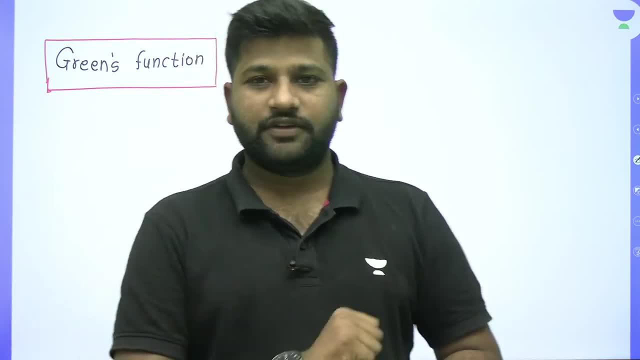 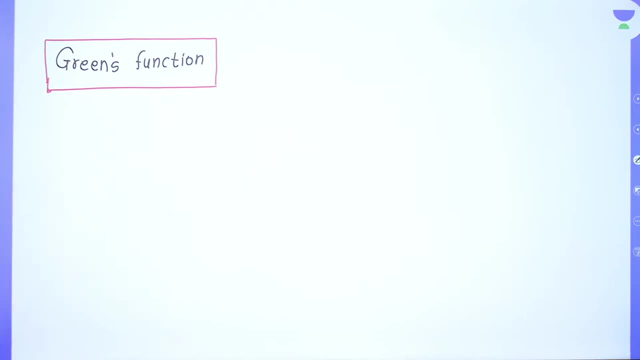 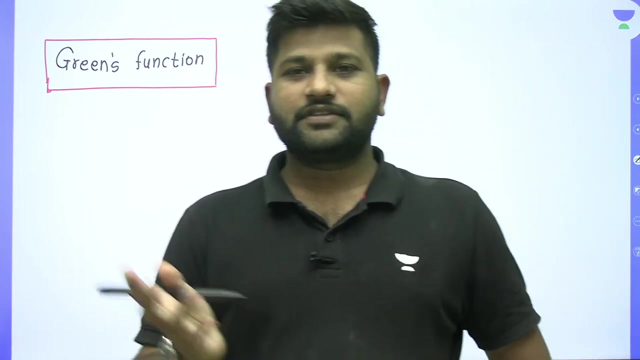 by looking at the question option, without doing these calculations. so we are going to discuss all these things good evening, good evening, good evening. first, let's discuss that this greens function. what is this greens function means why we use this greens function. what? 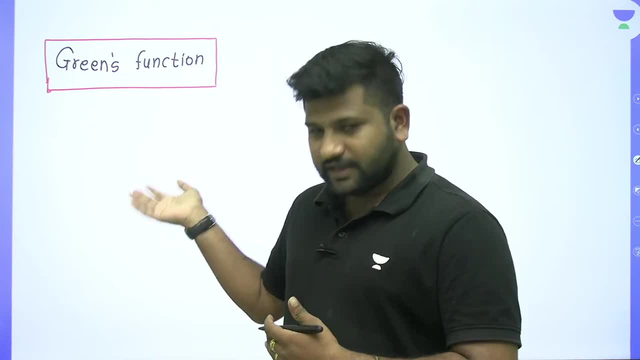 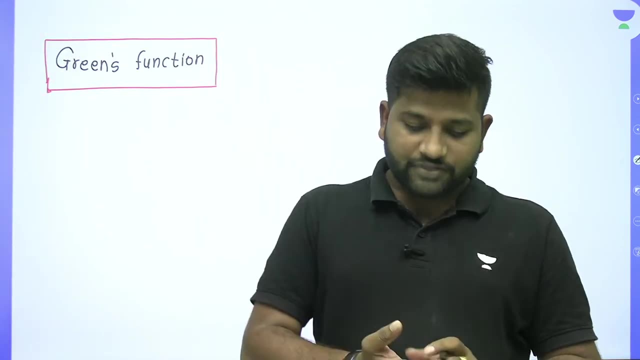 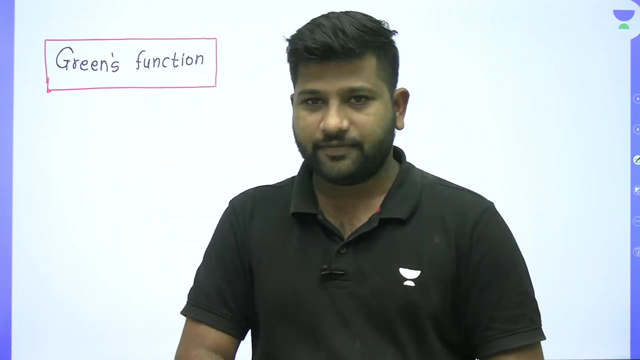 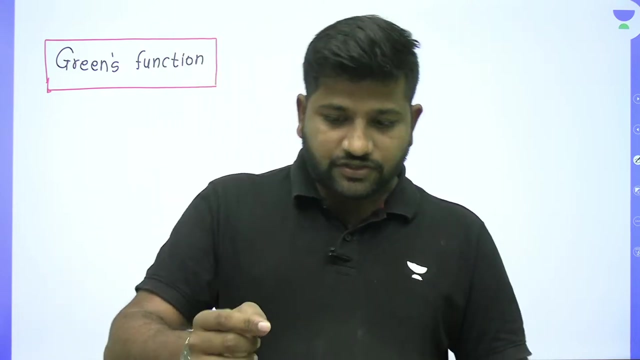 does it mean? we know the topic is the greens function, but how this means. what happens? it means that we have a differential equation and there are eight or nine ways to solve different equations, to solve the differential equation, but some differential equations are there. what we know? that the differential equation is homogeneous. differential equation- how? 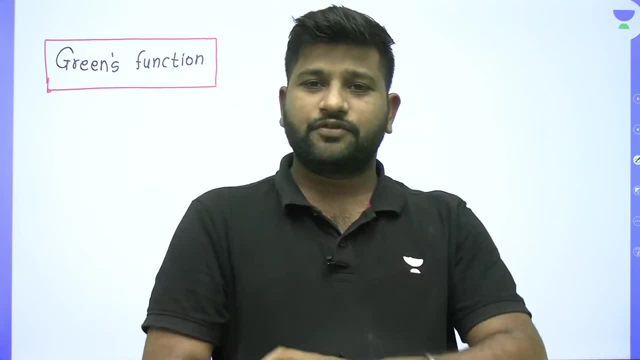 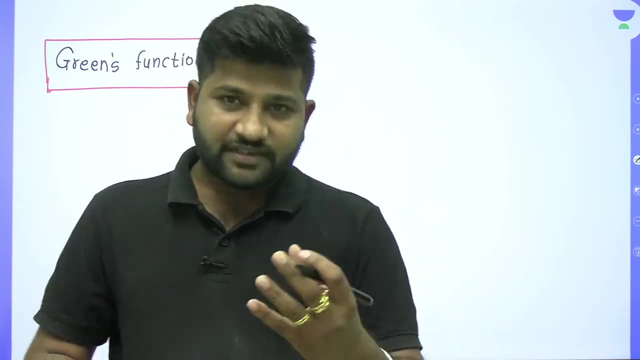 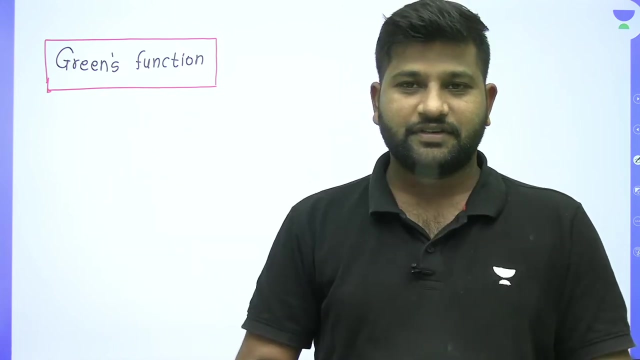 it is not homogeneous. there are our style of activating the differential equation. There are many types of differential equations, but some differential equations are such that the method we discuss in the differential equation cannot be solved by that method. That is why they are solved by a different method and that is called Green's function. 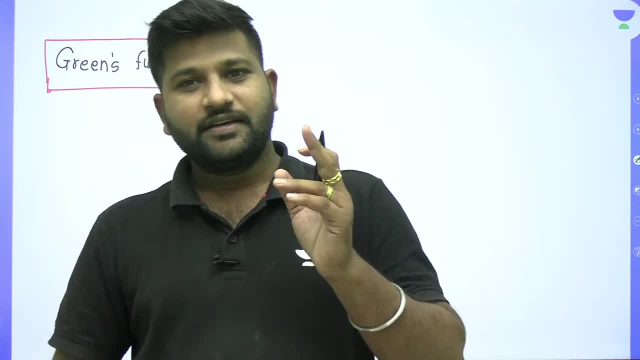 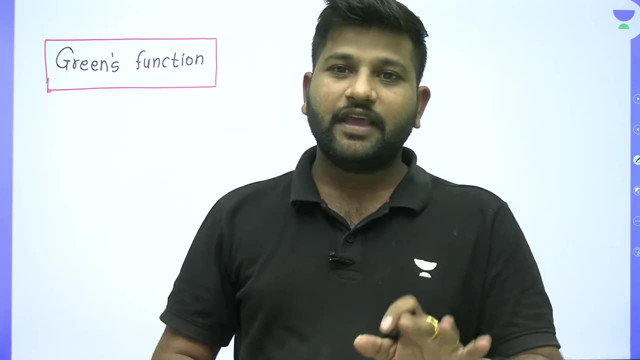 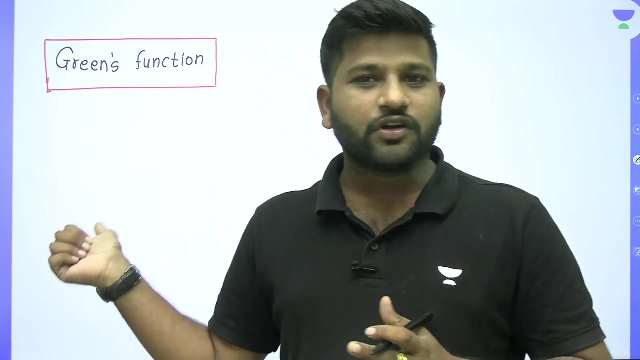 So Green's function is not a separate topic. this is the topic of the differential equation. What do we find out from them? By using this Green's function, we solve the differential equation. So Green's function is not a separate topic. this Green's function is nothing but the differential equation. 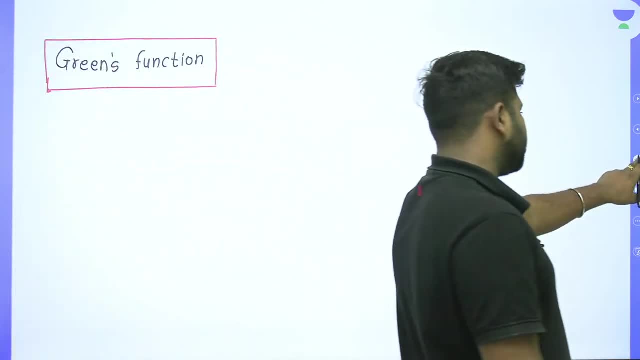 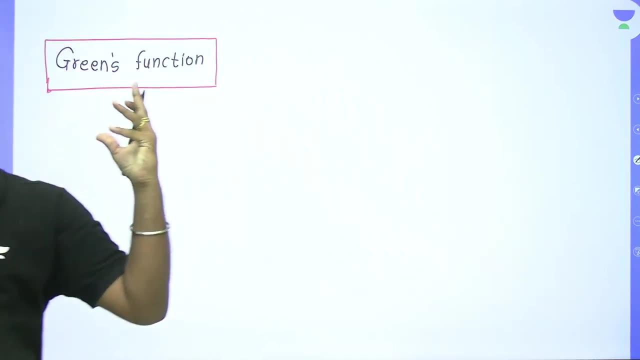 Solving of differential equations, the differential equations that cannot be solved by the methods we have. by using the Green's function we find them out. Sakshya ji good evening. Pujya puja ji, good evening. Did everyone understand? 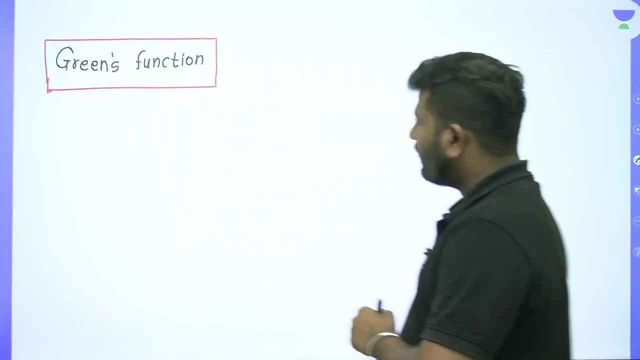 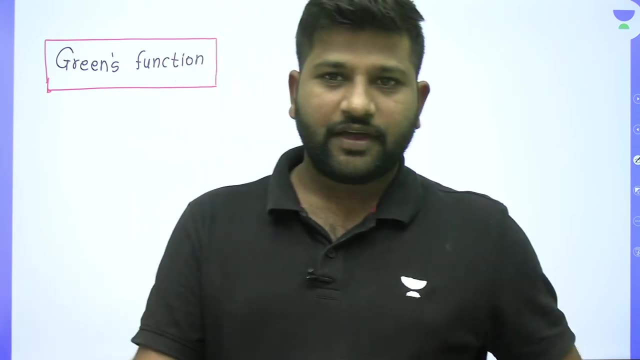 What is the meaning of it? Now see, we will directly enter the idea of Green's function on the topic, because now the exam is the day after tomorrow, it is the 16th, so the rest will not do much because you have to give the exam. 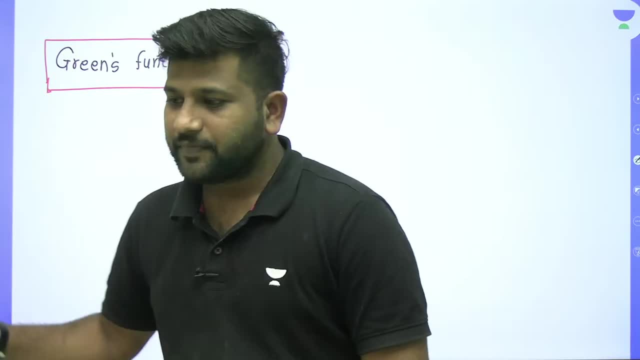 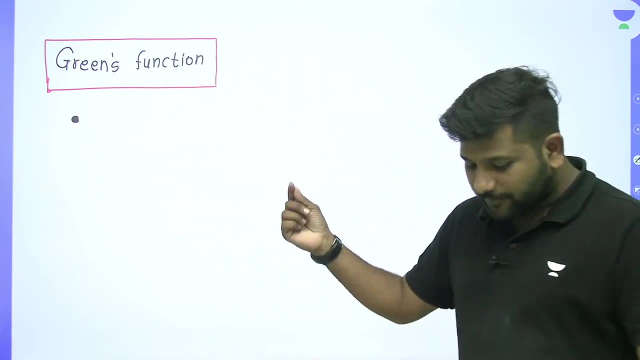 So we will talk directly point to point. Now, what is the basic idea in this? In this session, I will tell you how to find the Green's function. The Green's function is found out. I am going to tell you all the things right now. 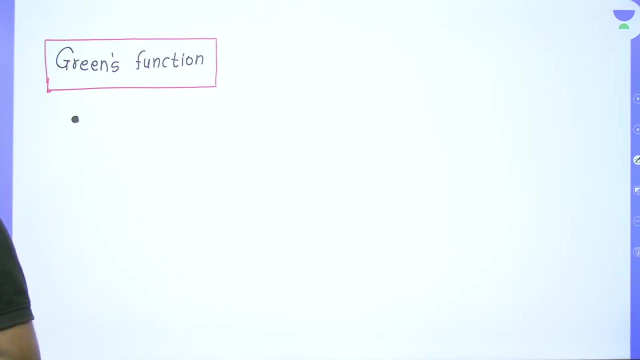 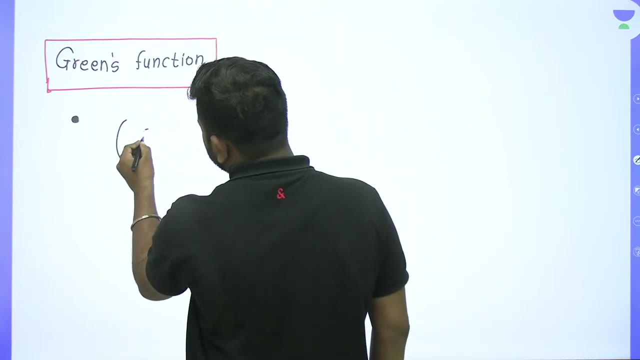 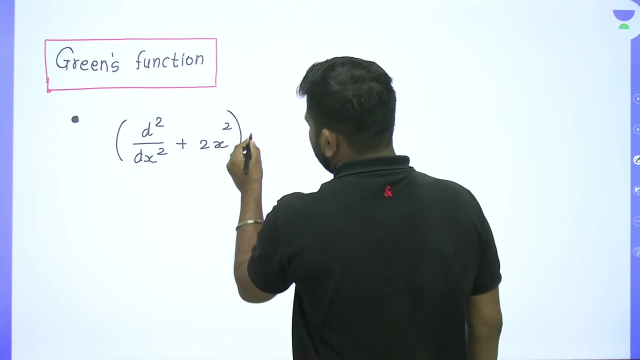 Good evening, Sanjay ji, Good evening, good evening, good evening. Let's say I have a function. I am just defining the function. Let's say d square by dx square plus 2x square. Let's say this y of x is equal to. let's say you have f of x. this is the function. 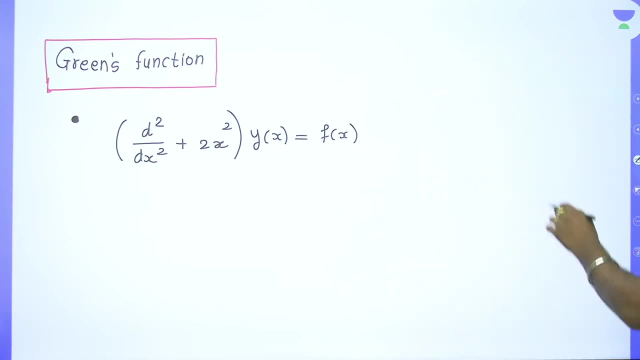 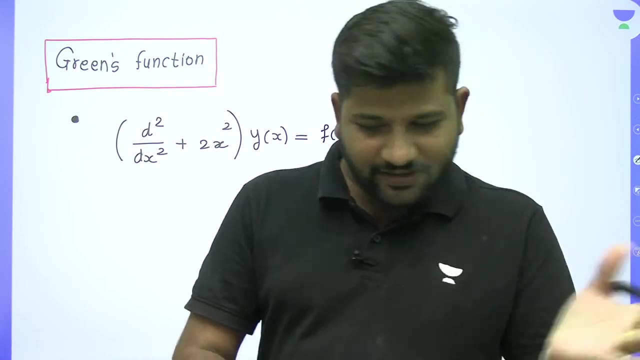 Let's say, we have this differential equation, This differential equation, you have a differential equation. See, if you have to assume all the things a little bit here, just see, everything will be clear in the future. Maybe it can happen earlier. sir, in 15 minutes, what are you doing? I don't understand anything. it can happen like this. 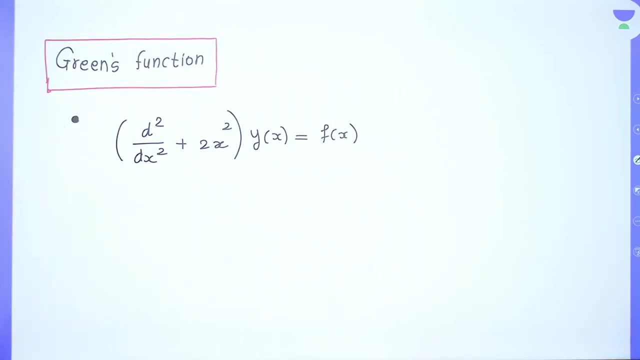 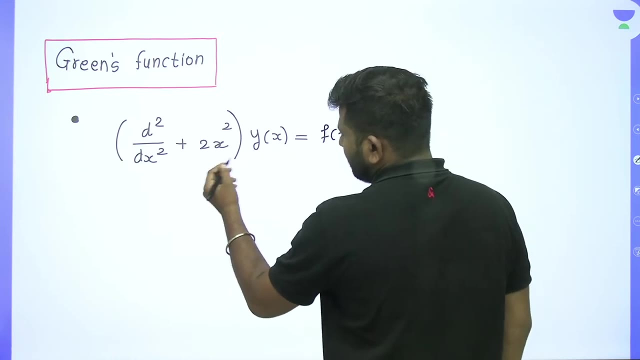 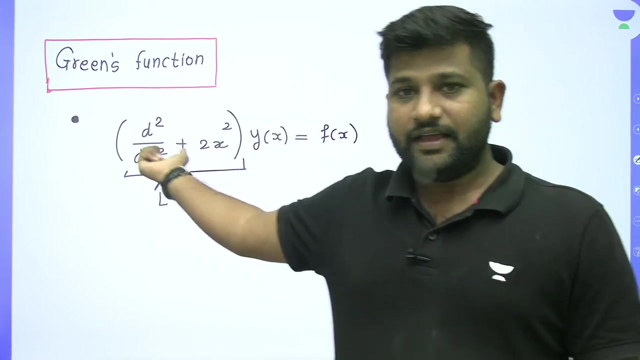 Isn't it? But its link will come to you in the future. Just believe: Okay, Now this one, what you are seeing, we give it a name. let's say: this is L, Because this is an operator. this is an operator, we gave it a name. 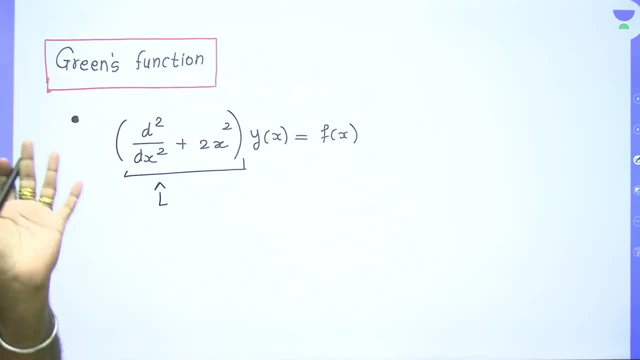 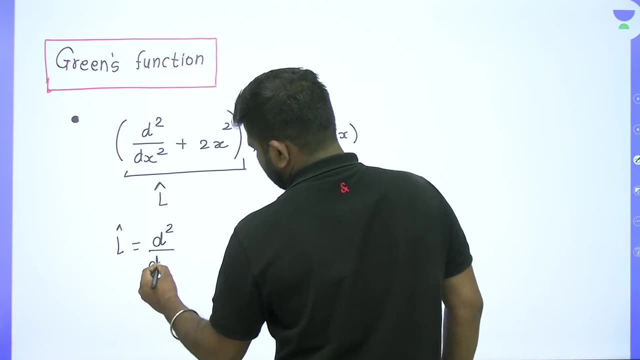 We gave it a name. let's say we have given. we gave them a name. let's say: L Means here this L. what is this L? Your L is nothing but d square upon dx square plus 2x square Means this is in your differential equation: d square plus this: 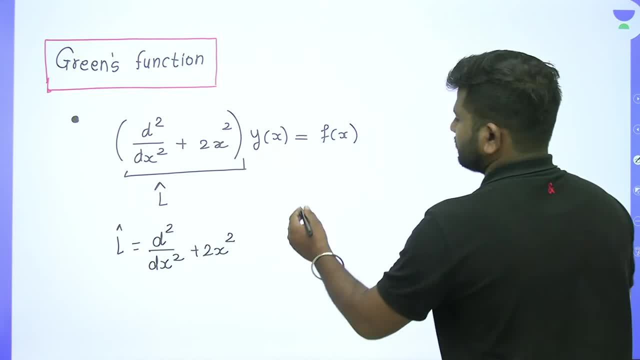 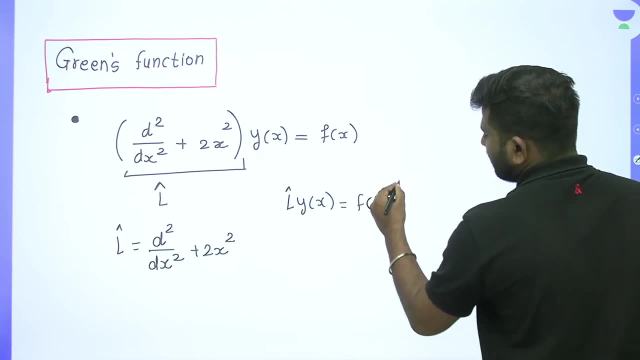 So we gave them a name. what is this? This is L. that means we can write it like this: that L y of x is equal to f of x Means we can write them like this: Okay, We can write them like this: 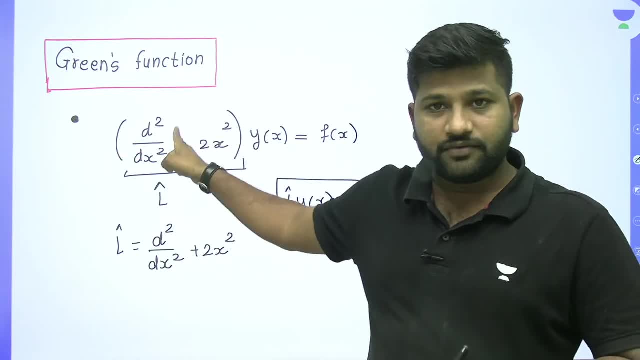 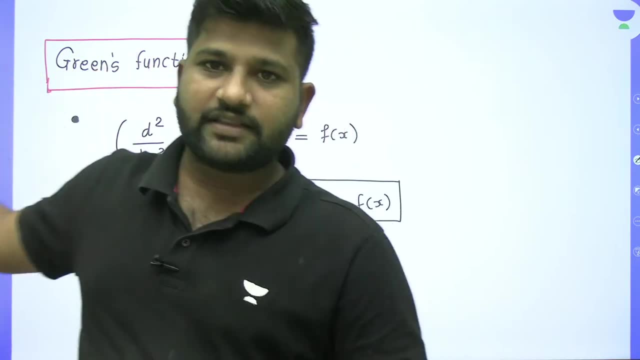 Now, this is a differential equation of this type. Assume that this is a differential equation of this type, That we have a lot of methods to solve differential equations, But this differential equation cannot be solved by that method. This is a differential equation of this type. 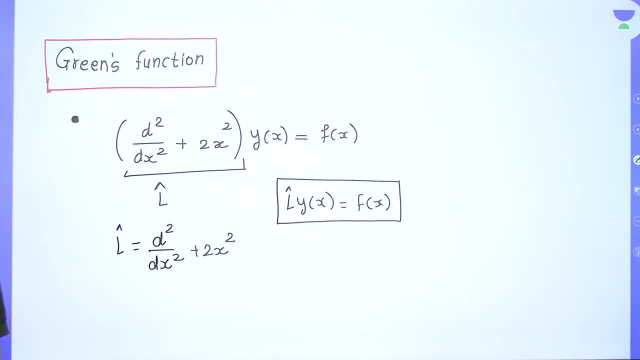 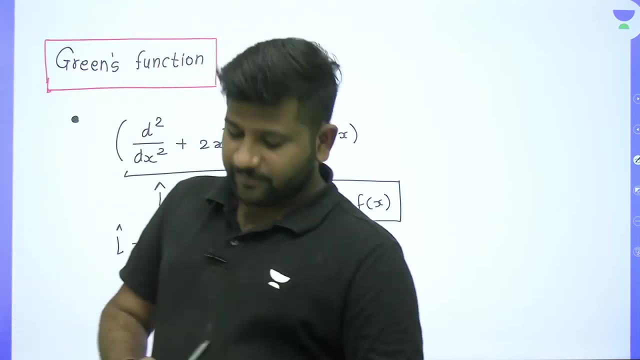 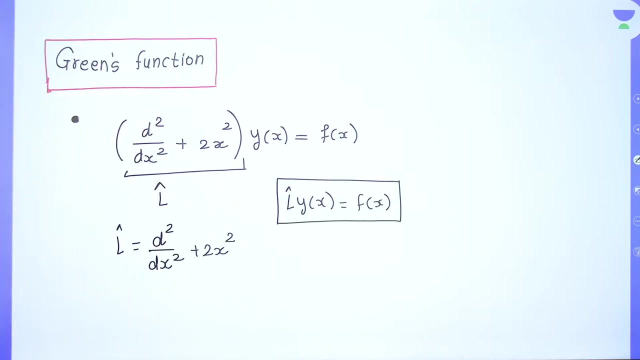 Let's assume it like this. Okay, Mr Devraj, I have taken branch cut and branch point in full detail in the special class. See once in the special class. I have taken it in full detail. I have taken 3-4 lectures, I think. 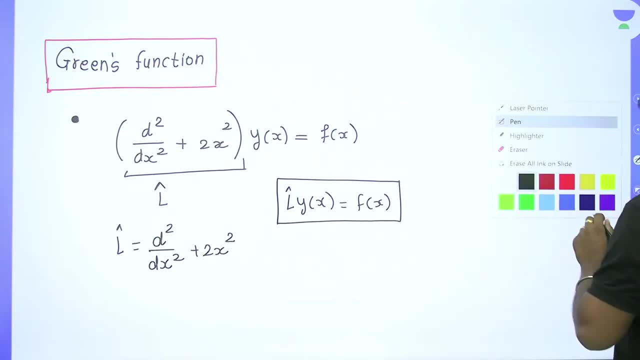 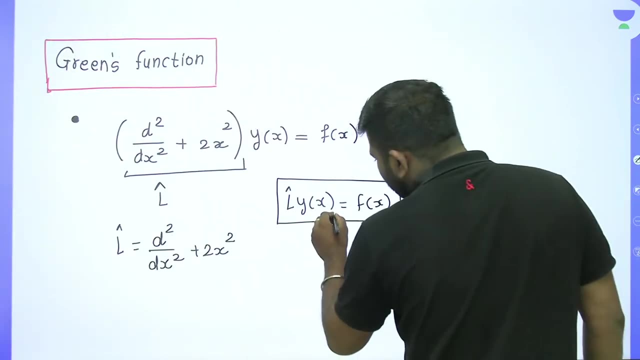 Isn't it Okay? So this is: this is not an angular momentum operator. I just gave it a name: L. Okay, Now, by solving them from here, what do you have to find? What is your aim? What is your aim in the differential equation? 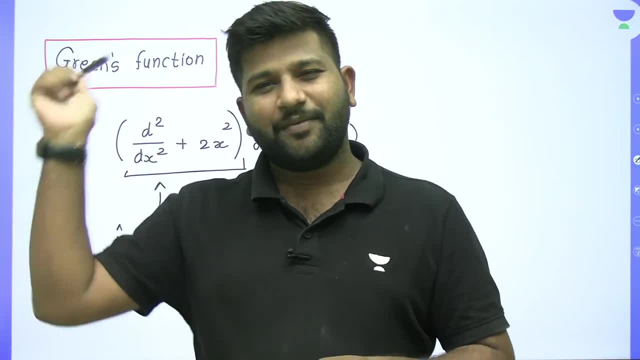 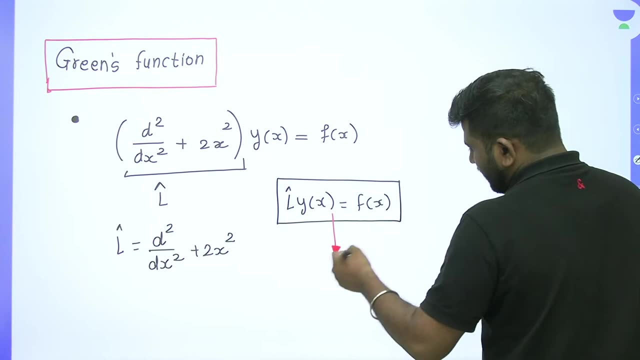 Your aim is that you have to find out the solution. The aim of the differential equation is to find out the solution. So you have to find out the solution. That means your ultimate aim here is the same: That you have to find out this y of x from this equation. 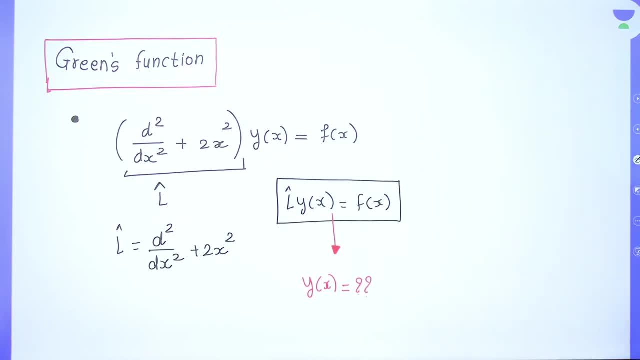 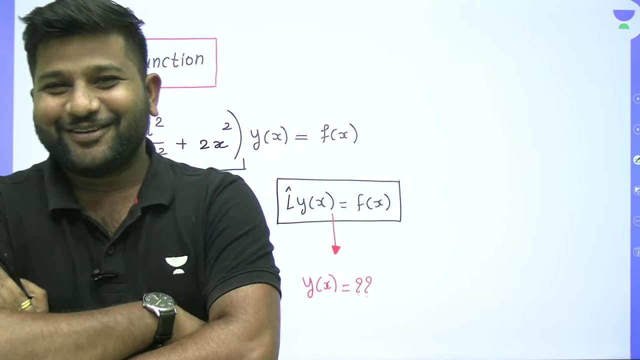 Okay, Okay, Hey, not an angular momentum operator, man. I wrote it like this, Isn't it? Okay, Now solve them here. Okay, Now solve them here. Okay, Now solve them here. Okay, Okay, Now solve them here. 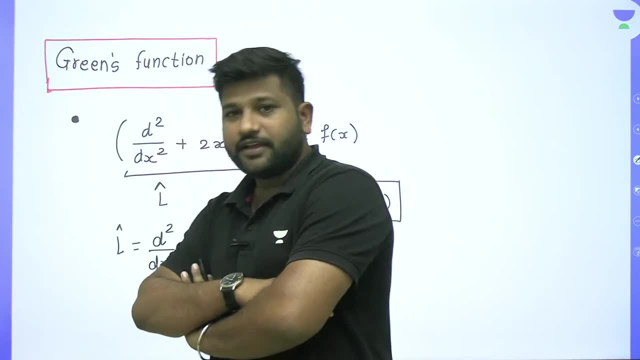 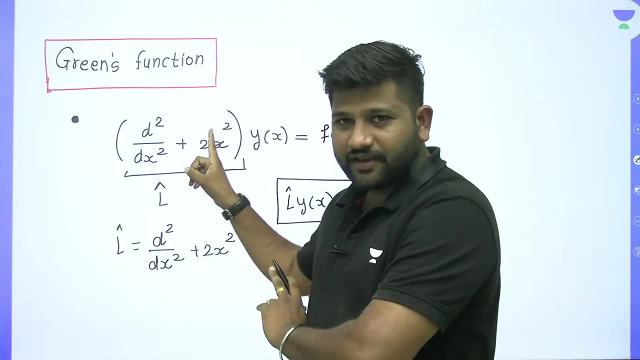 Okay, Now here, how will we solve them? So here we will define a function. Okay, What does the function mean? This is the differential equation. Look carefully, This is the differential equation. Yes, Do you know the solution of this differential equation? 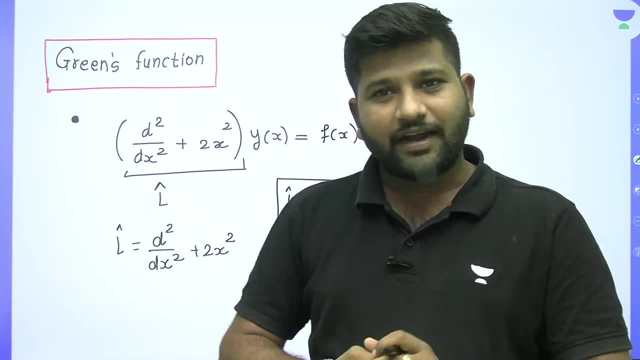 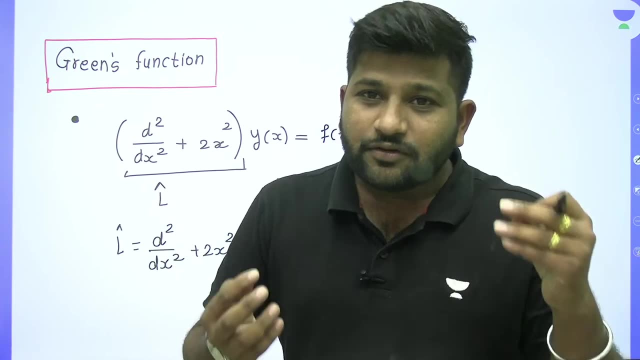 I don't know. Do we try to find out from the greens function? Yes, But here we don't even know the solution of the Greens function. But here we don't even know the solution of the Greens function. we have to assume that. what is the meaning of the solution? 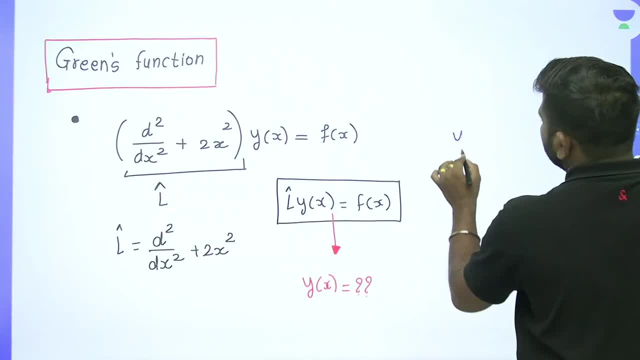 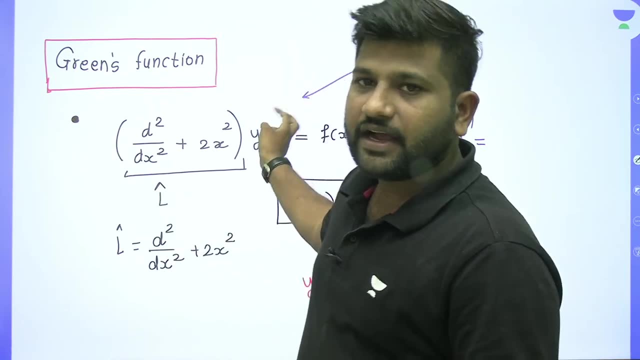 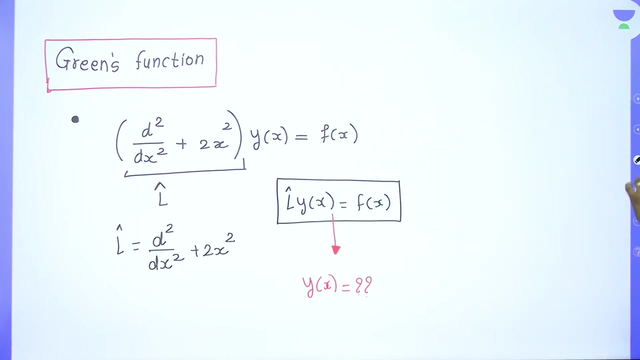 what is the solution? solution means that if we substitute the value of y in this equation, then LHS is equal to RHS. that is called as solution. that is called as solution. so we have to find out that. so for that we have to define a function. 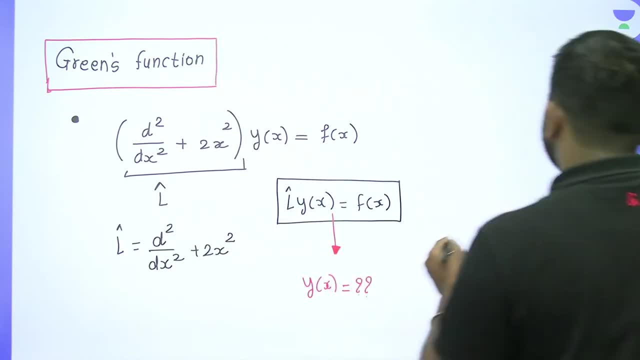 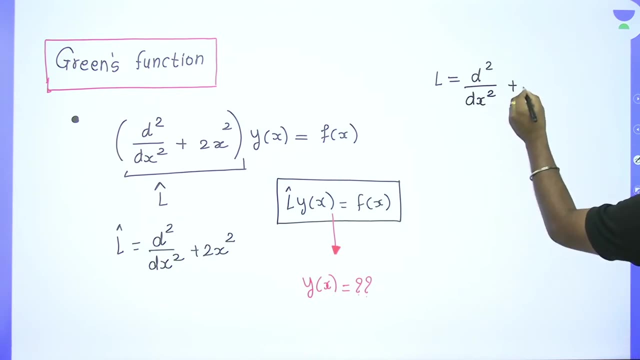 and that function is called as Green's function. so here we have taken what is our L. so our L is d square divided by dx square plus 2x square. so this is our L, so this is our L. then we will define a function. now, what does this function mean? 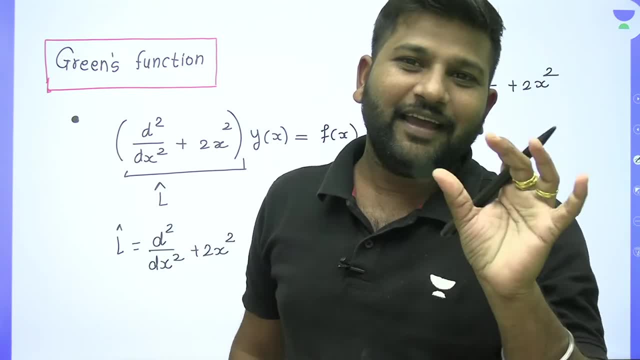 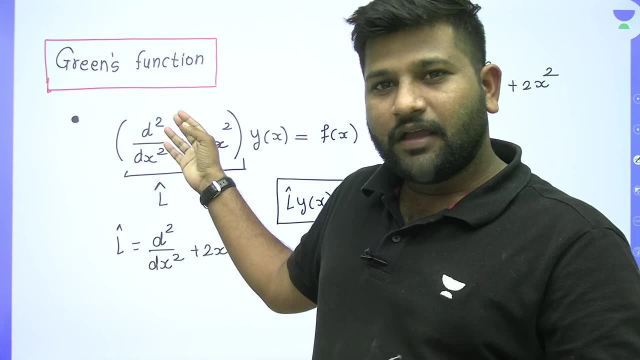 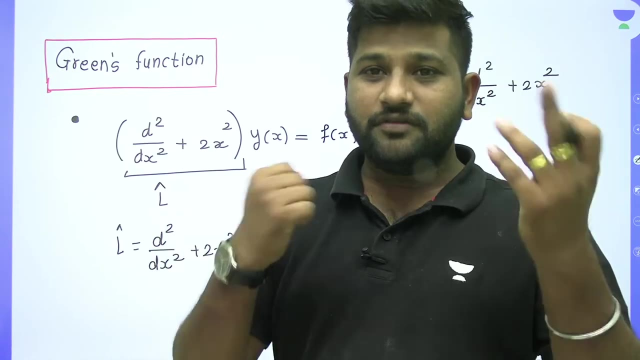 this function means that this differential equation- we don't even know the solution- those who have done this method, they also didn't know the solution. so what they have to think? that they have assumed that this is the solution, just assumed, like this, that this is there, this is the solution. 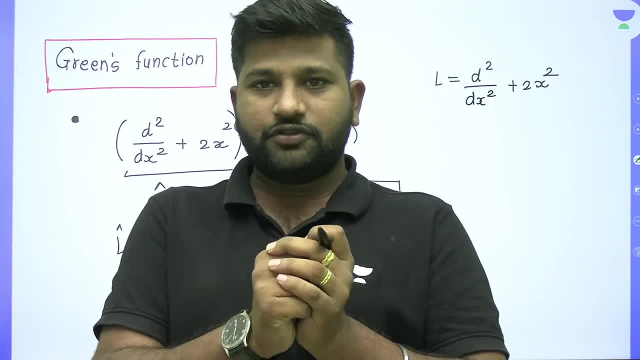 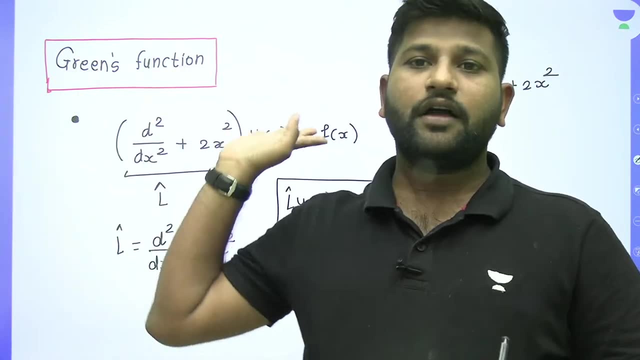 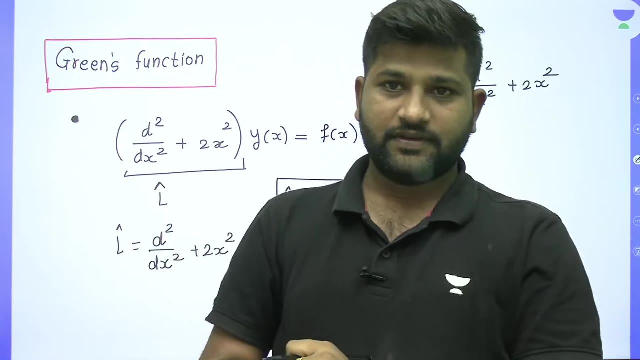 assumed like this: if we have assumed like this that this is the solution, so we put it in differential equation and if differential equation is satisfying, then what will be your solution? as simple as that. whatever we are doing here, that is all about the assumptions. we are assuming that. 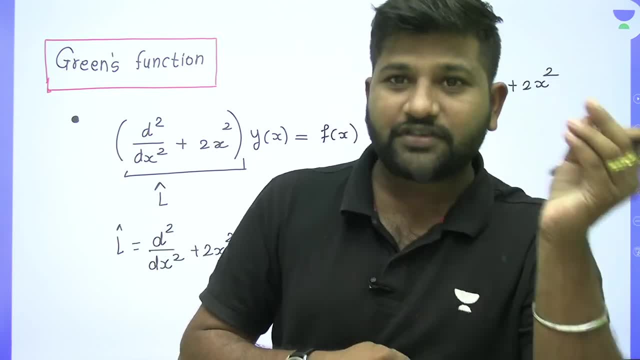 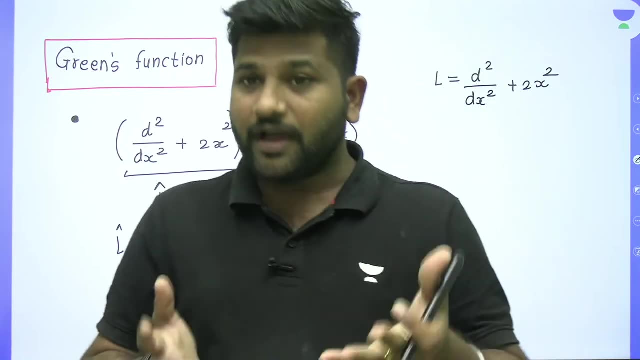 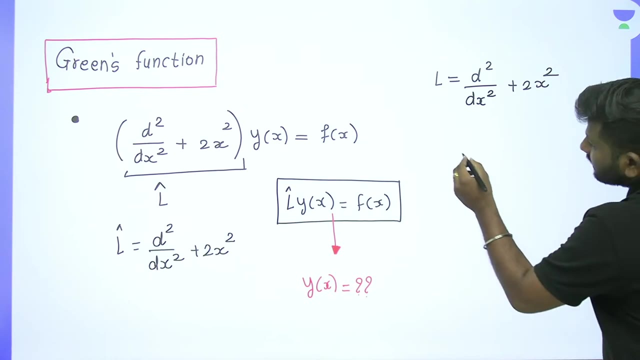 this should be like this, then this will be the solution of differential equation. we have to prove that the assumption we have taken is right or wrong. we have to see that too. you are understanding what I am saying right? so here we have taken L, so they have assumed that. 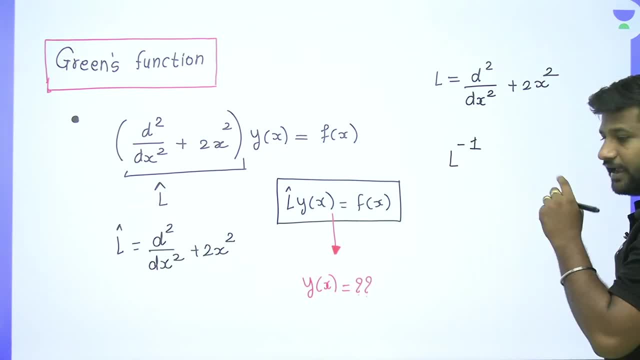 here this L inverse, what they have taken. this is L inverse, which is equal to G of. so here see this function. this function is defined, that L inverse is equal to G of and this function is called Green's function. that means we can write from here: 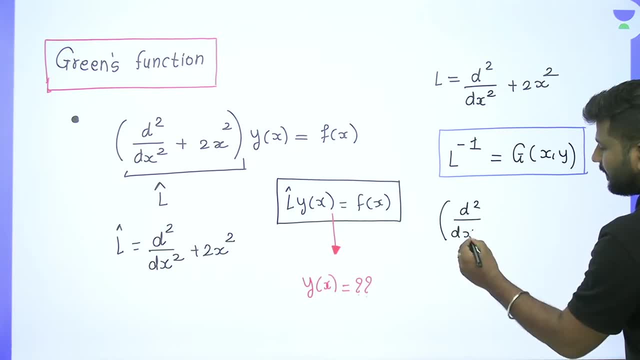 that d square upon dx square. don't worry, this topic is very simple. this will be your- let's say this, so its inverse, and this is nothing. but what is your Green's function G of? we have just assumed them like this: now, with them, we will do all the things. 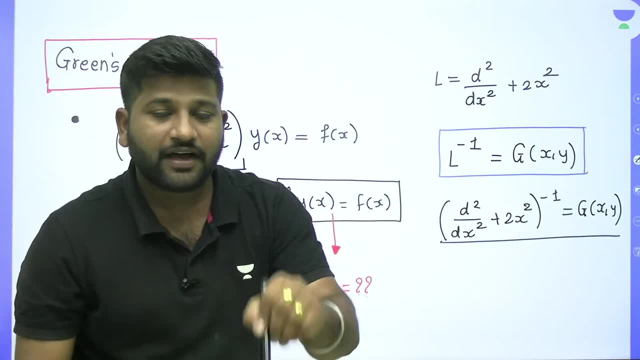 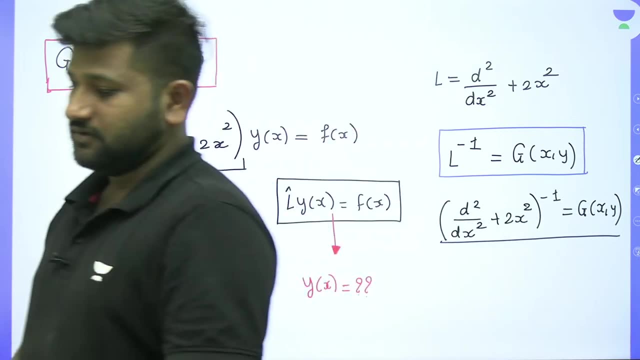 and then we will see that, by using them, the solution which we take out. so that, does your differential equation satisfy or not? you are understanding what I am saying, right, what I am trying to say, right, isn't it ok? I hope you understood this. 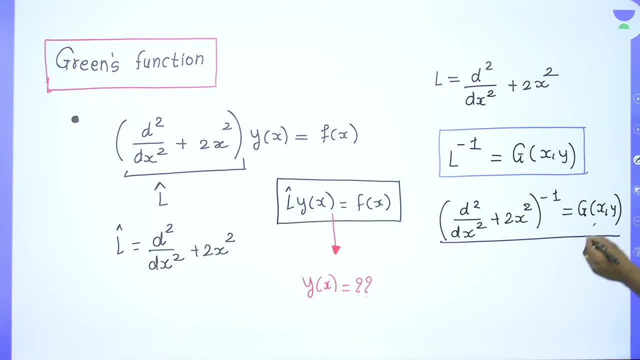 all of you. so this, this is called Green's function. this function, this function is called Green's function. this is nothing but the Green's function. definitely here you in CSIR, 5 marks question you get on this. there will be 3 sessions. just attend 3 sessions. 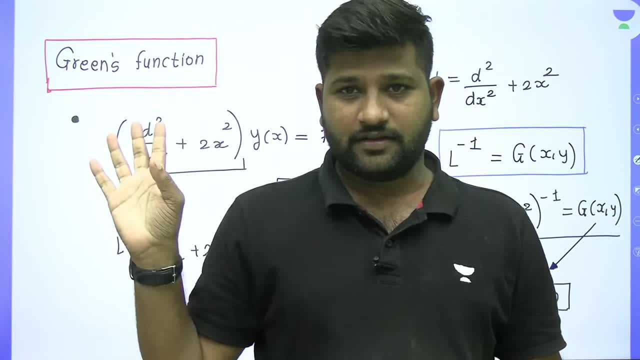 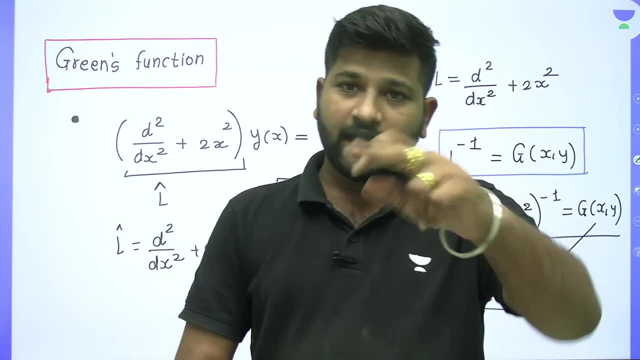 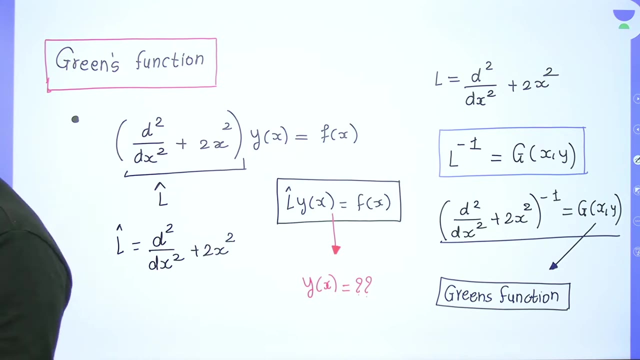 your Green's function has 5 marks. definitely 3 sessions. 1 hour, 3 sessions, only 3 sessions. this complete in this question with the help of all the PYQs previous year question, including this in this 5 marks question, definitely, you know now. 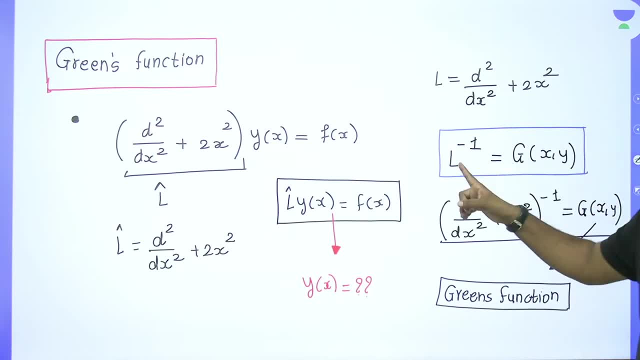 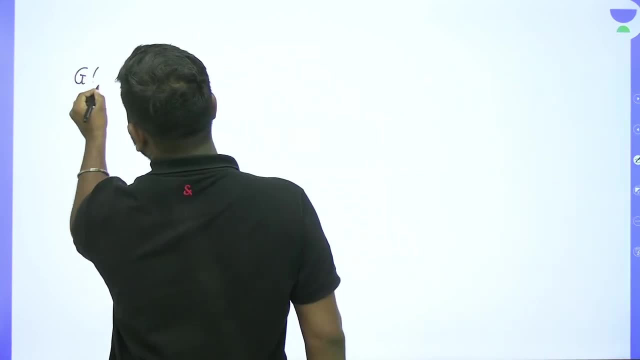 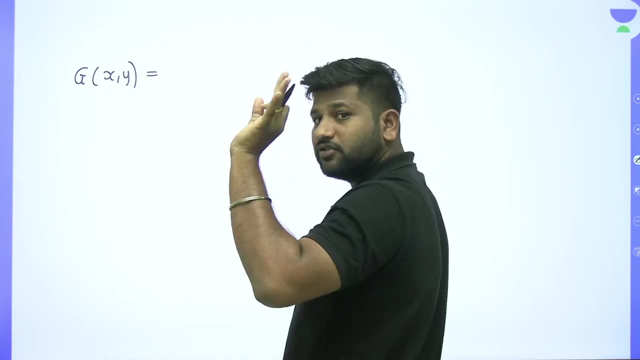 see here your Green's function. we took this, this Green's function. your Green's function is this: that means, if I write this Green's function like this, then g of x, y, this is your Green's function today. you will think that, sir, what is x? no, no, no. 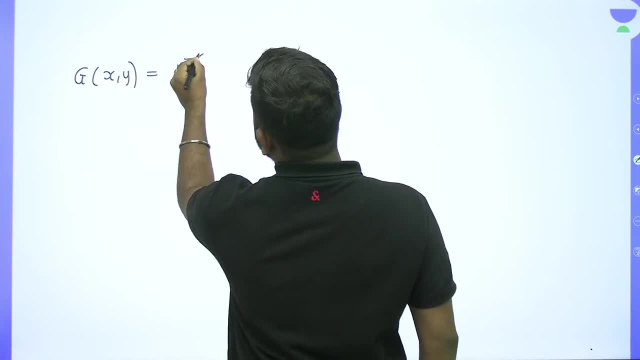 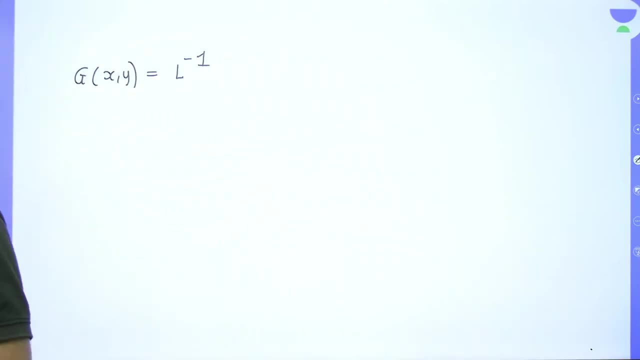 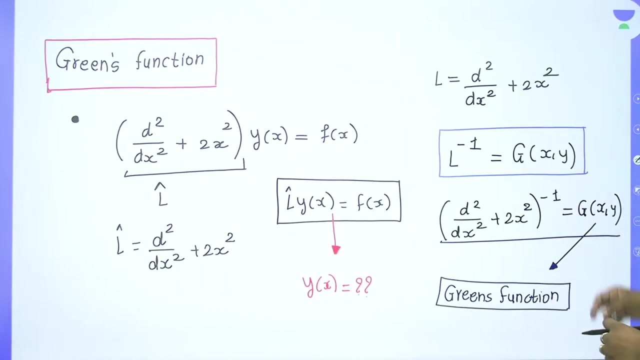 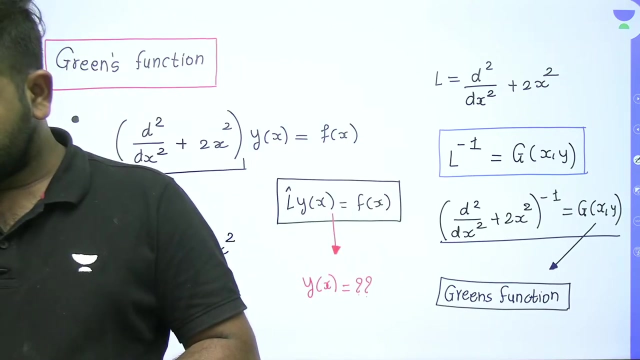 this y is different. what is wait? so this is your L inverse. now what we will do. this equation, this equation's both sides, ok, ok, this Green's function means this Green's function is also an operator, isn't it? this Green's function is also one of. 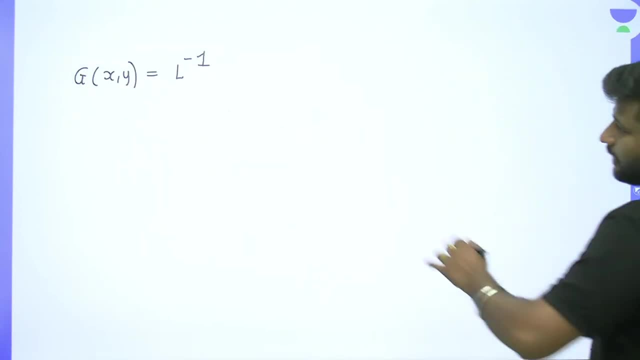 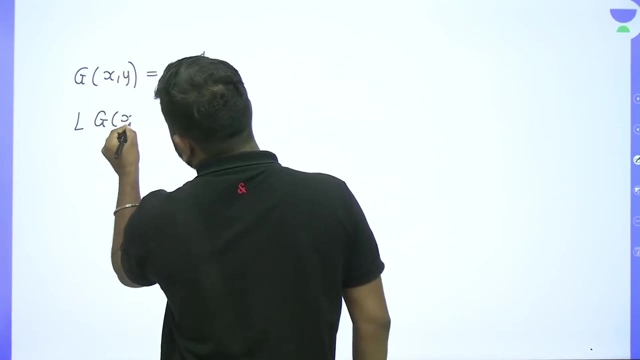 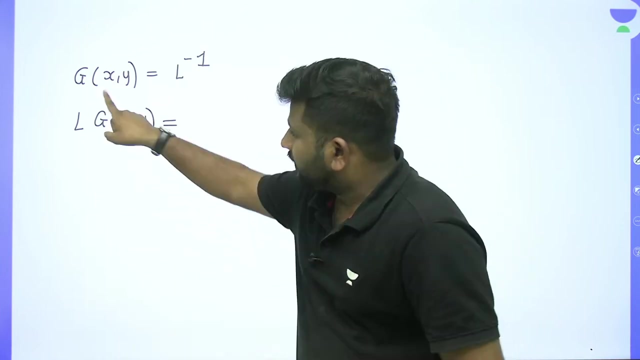 operator. now what we will do here, see, we will operate L on both sides. so what will happen by operating L? this is g of x. y is equal. to see now here: this is a property of Green's function. so here, what is this? this is a Green's function. 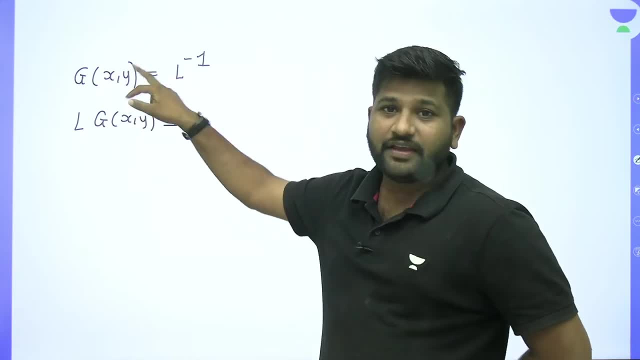 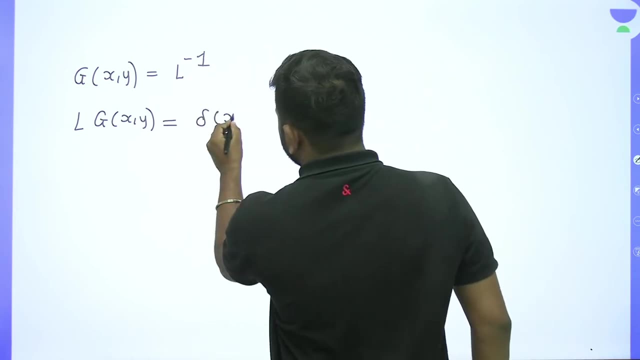 is nothing but the L inverse. ok, now what we did? we operated L on both sides. so here we operated L. so L into L inverse. this should be 1, but this is nothing but the L into L inverse. so this is the property of Green's function. 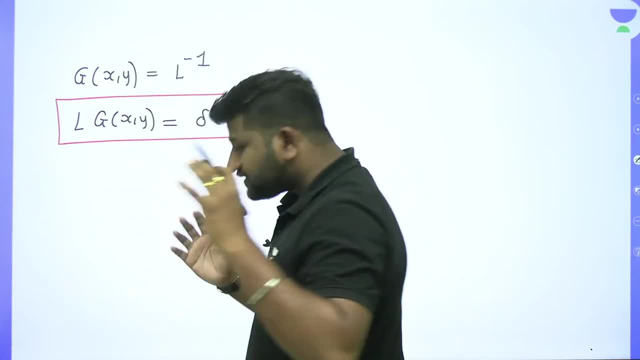 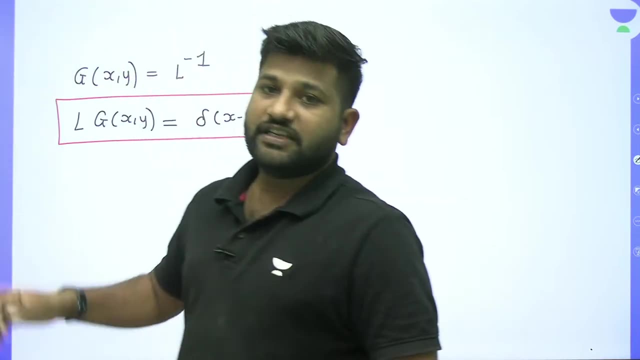 this is the property of Green's function, means this Green's function. we are defining that Green's function, this relation, this relation, what will it do here? it will satisfy. now. we will not take its derivation. it will take very long time and if you want their derivation, 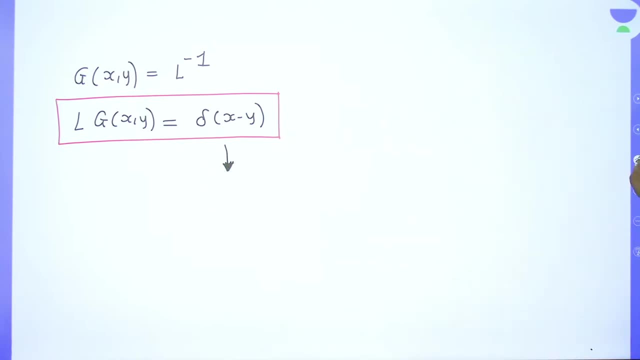 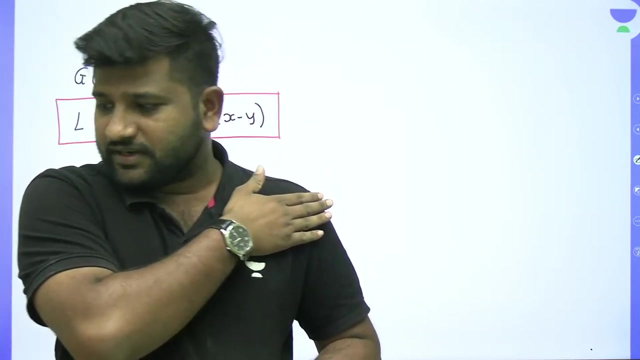 then RKN and Weber. you have read from that book- you will also get their derivation. ok, If you take L into L minus, then how does this direct delta x minus y come? that we are not going to do, okay, No, no, no, no, no. Green's function is totally different and Green's theorem is totally different. okay, 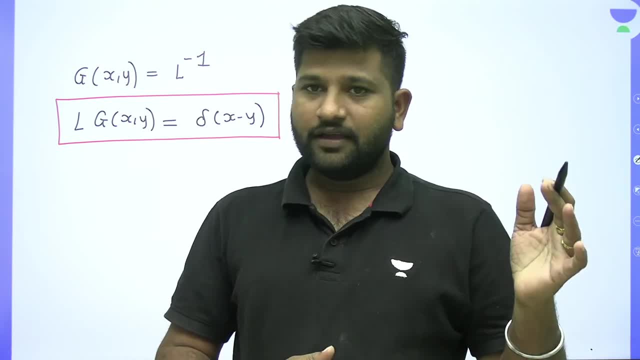 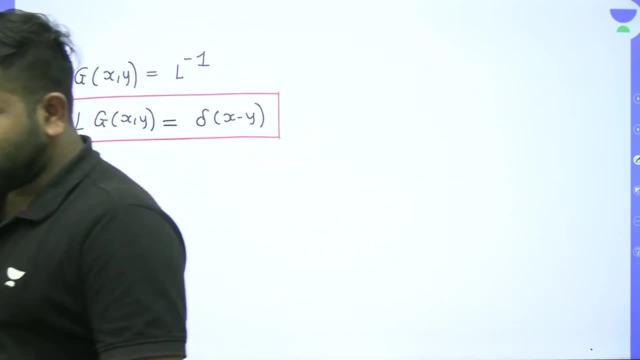 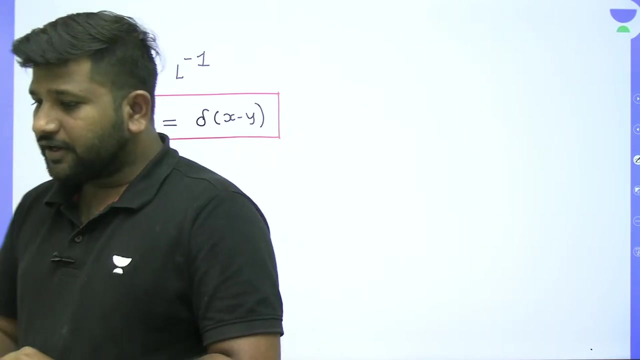 Green's theorem is different. okay, Green's theorem is nothing but the Stoke theorem. Stoke theorem in a plane is the Green's theorem. This is a different thing. okay, This is different. okay, I hope you understood this okay. 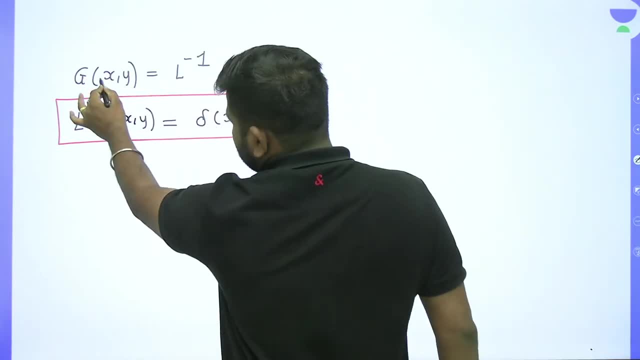 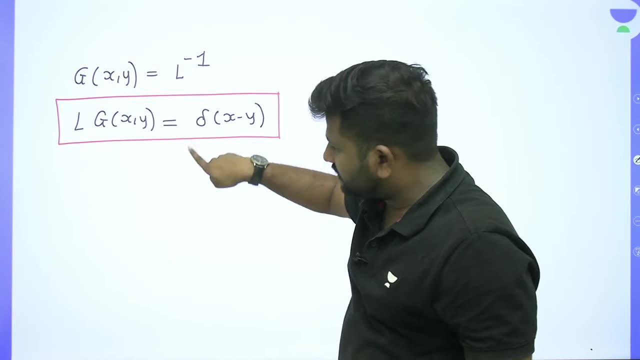 So this is your Green's function. If you operate L on both sides, then here Lg of x, y is equal to L into inverse is not 1, which is equal to direct delta x minus y. This is the property of Green's function. 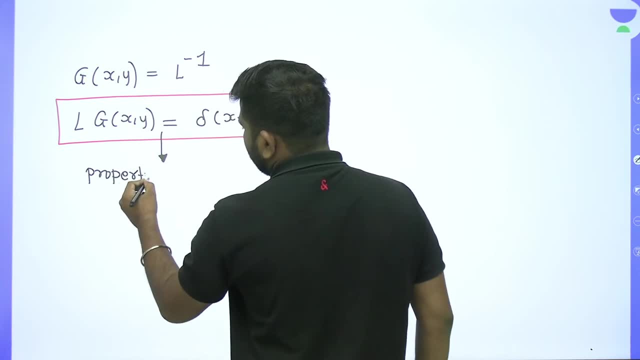 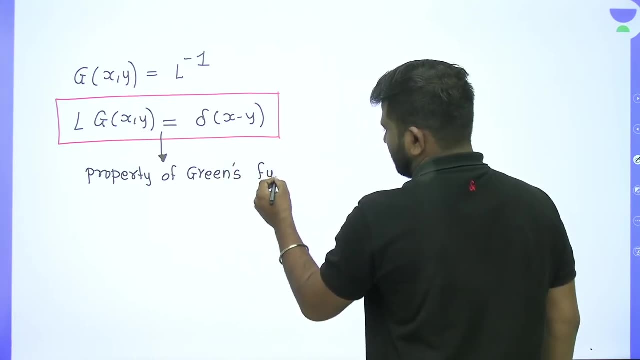 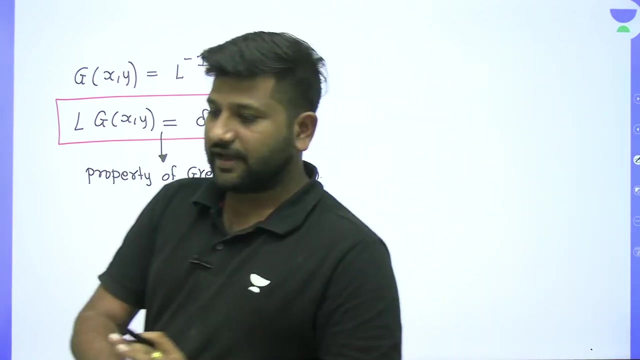 This is the property of Green's function. We are not going to do derivation because we don't have that much time, right? If you want, then you can see the book of Erbkahn and Weber in that very simple and simple language. I have given you the given, okay. 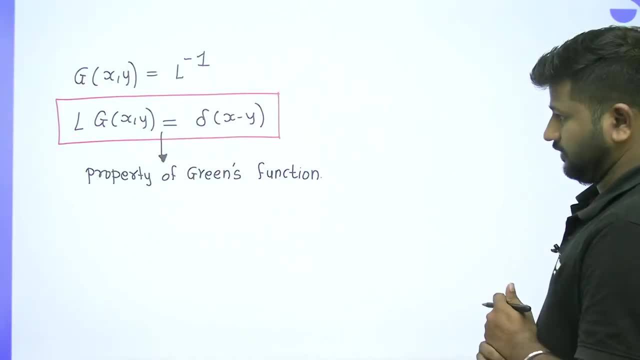 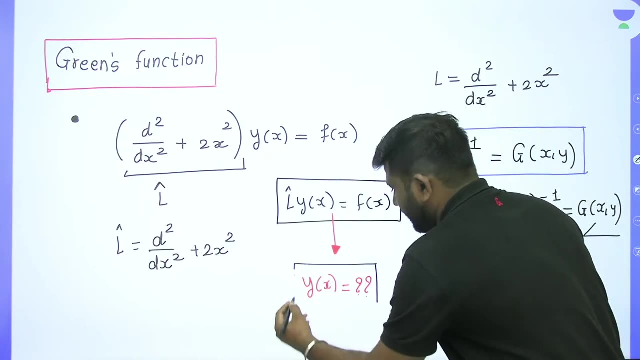 Now let's move ahead. So what is our aim, What we have to find out? finally, we have to find out the solution of this differential equation. Now the questions that will come from here will be of two types. First, you will get the given. 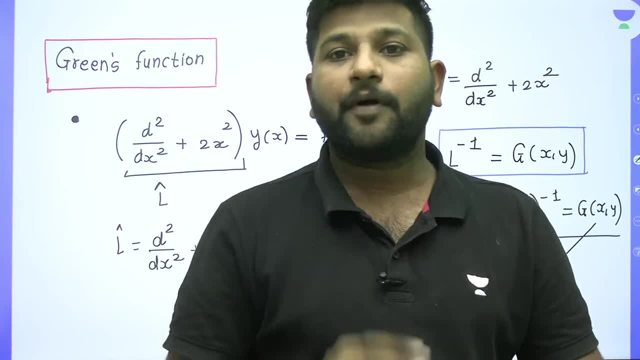 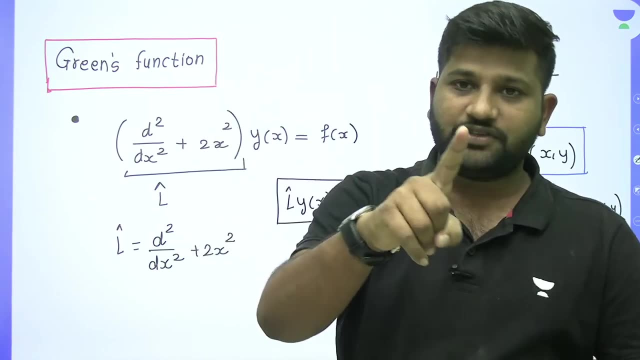 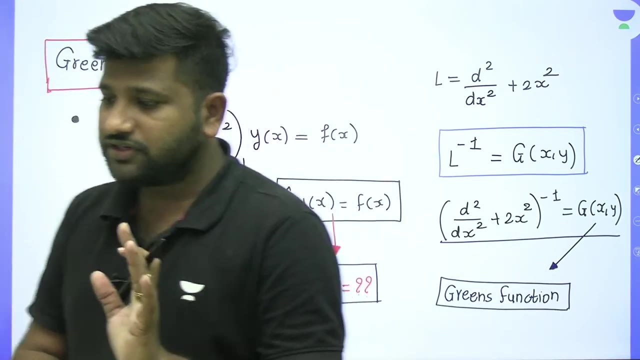 Second, you will get the given. If you want the solution of the given differential equation, then we will ask you to find out the Green's function for this differential equation. So, for this differential equation, we will ask you to find out the Green's function, or we will ask you the solution for it. 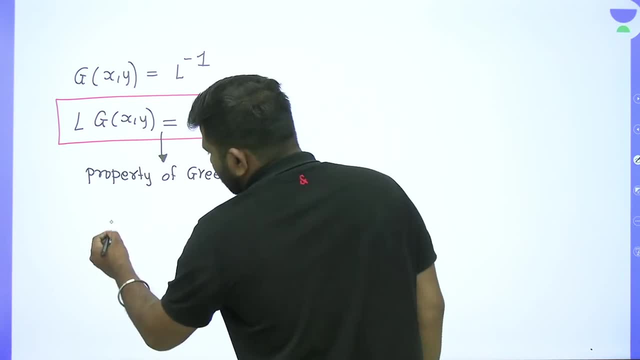 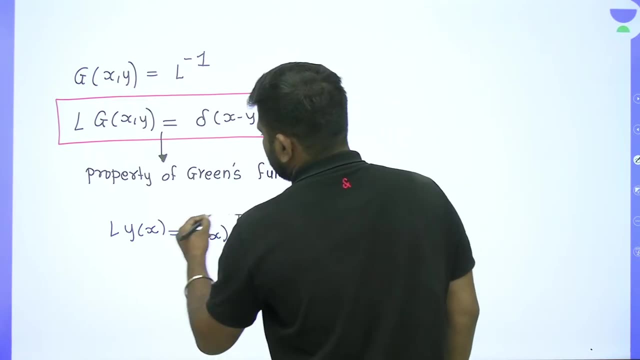 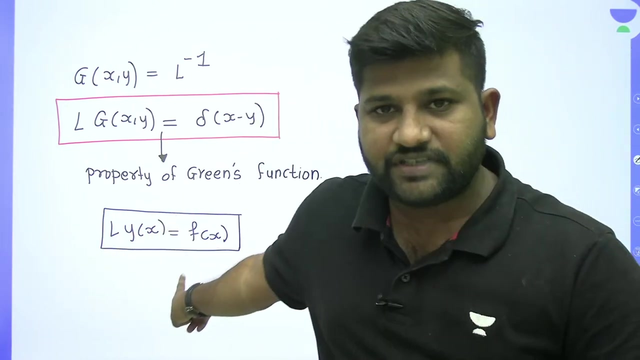 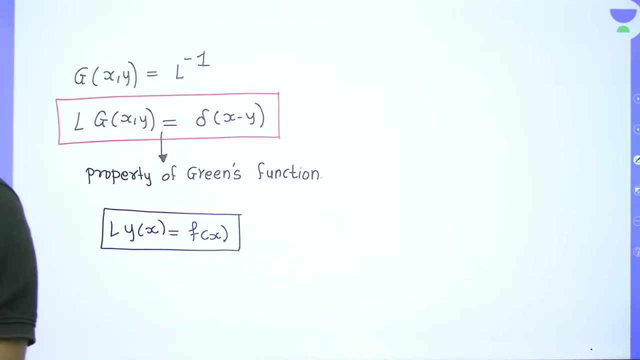 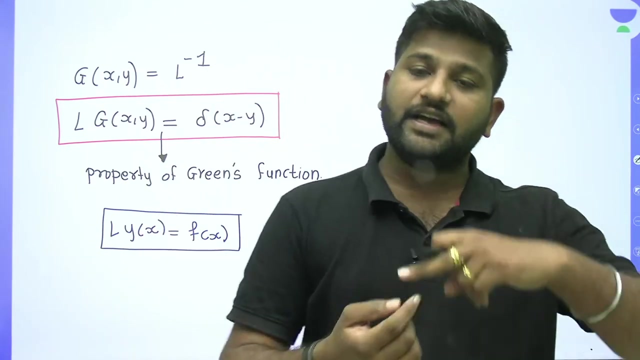 So here we have the relation that L y of x is equal to f of x. This is our given differential equation. This is our given differential equation. now, what will happen here? now this differential equation has a solution, we will assume that solution. what we are going to do, Ganesh Deshmukh ji, good evening, good evening, good evening. what we are going to do now, this differential equation, we will assume that I am assuming a solution here. what we are doing here, assume 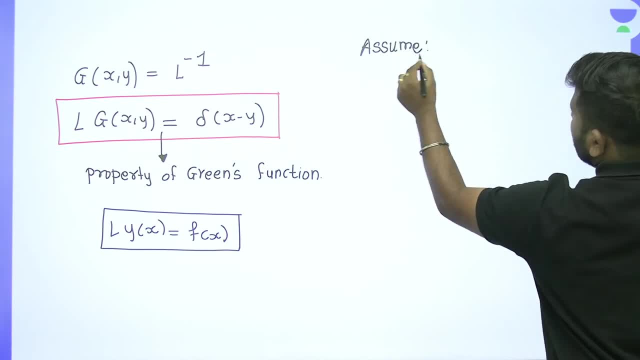 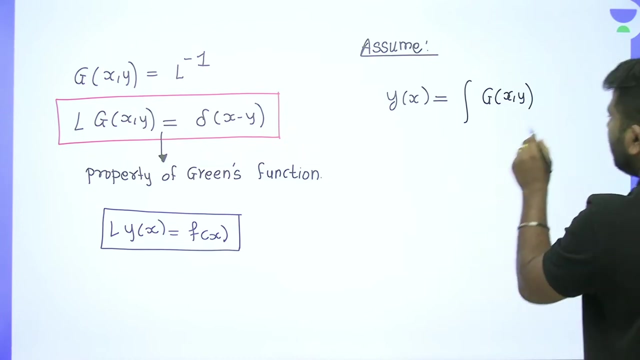 we are going to do this. see, we are assuming that this y of x is equal to what will happen. we are assuming this: this is integration g of xy. what is integration g of xy, f of y, dy. so this is your given differential equation. this is the solution we have assumed, like this: 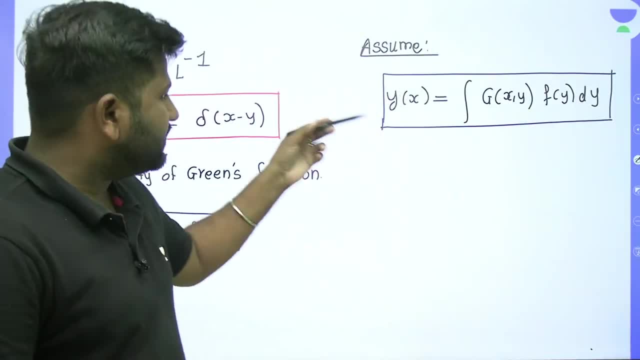 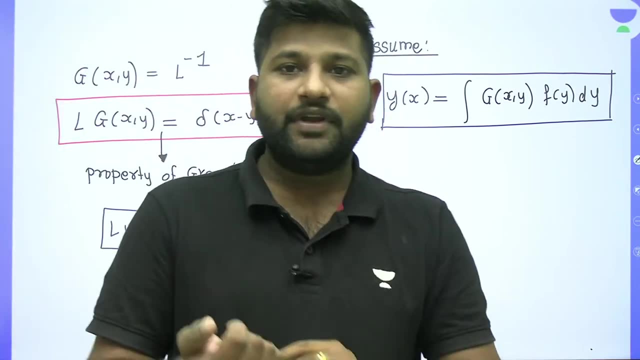 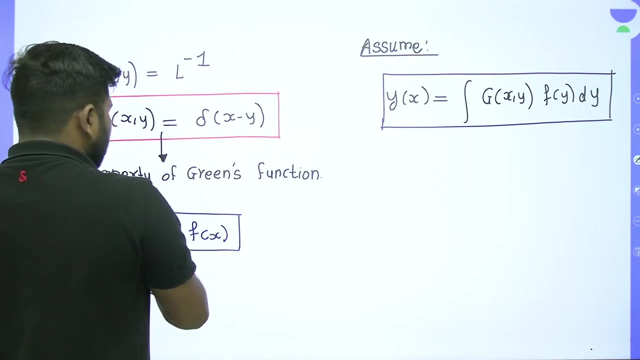 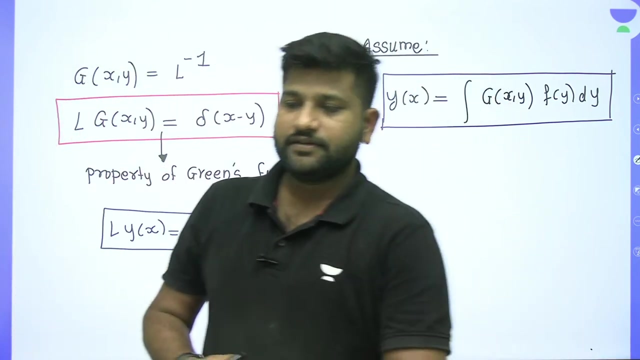 we just assume this. we have assumed that this differential equation, this differential equation, will have this solution. Poonam ji, good evening now here. we have assumed that this will be its solution. this means that if we put the value of y in this, if we put the value of y in this, then how much should its answer come? f of x? how much its answer should come. 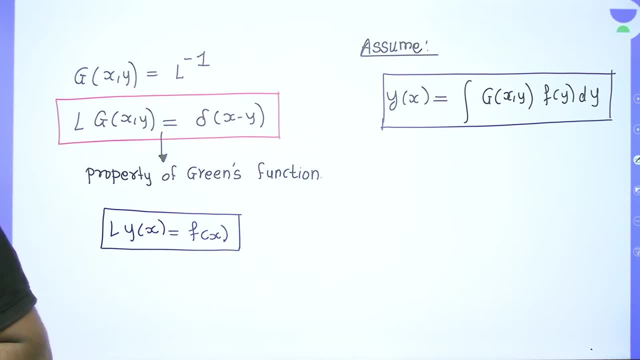 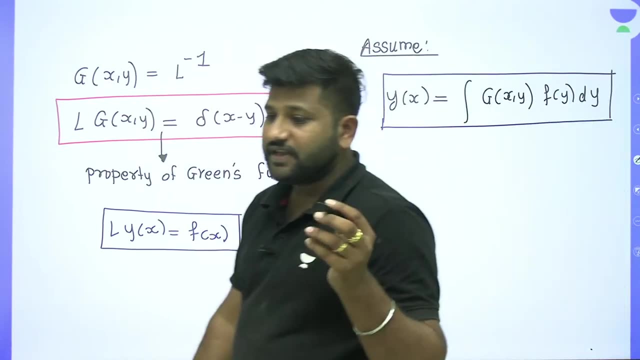 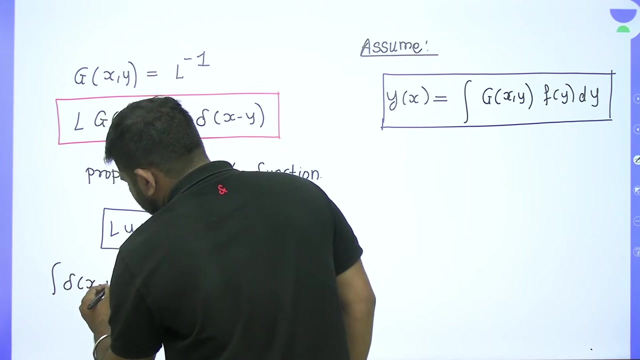 equal. if we assume this, then this answer should come to you. okay, so we know that. so you people know the properties of the direct delta function. it is important to know the properties. okay, that integration direct delta of x minus y. I had already discussed this property in a class, maybe. 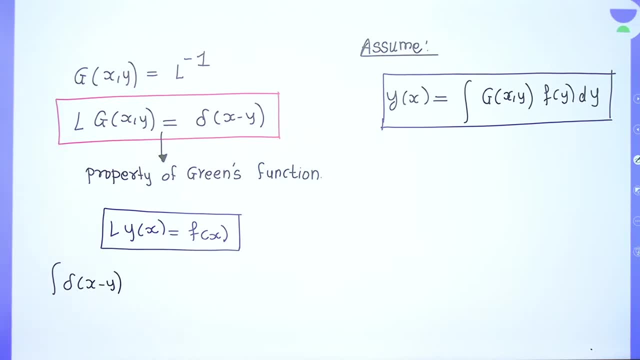 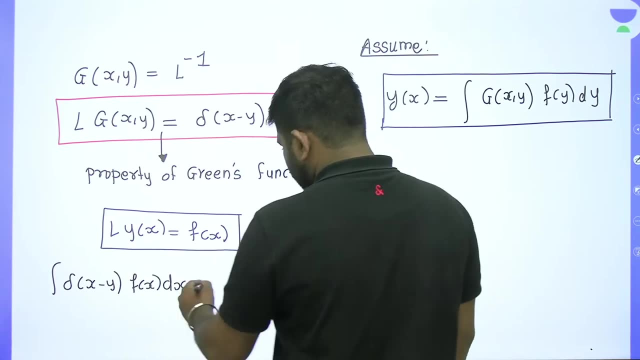 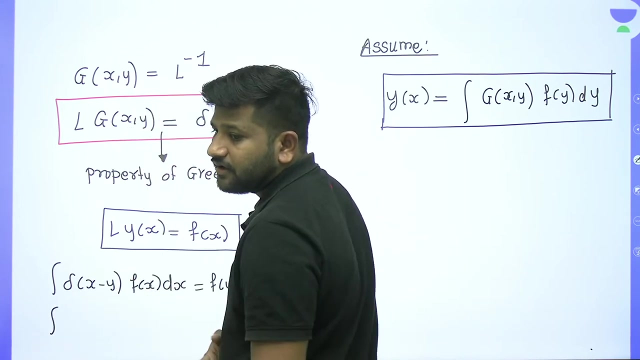 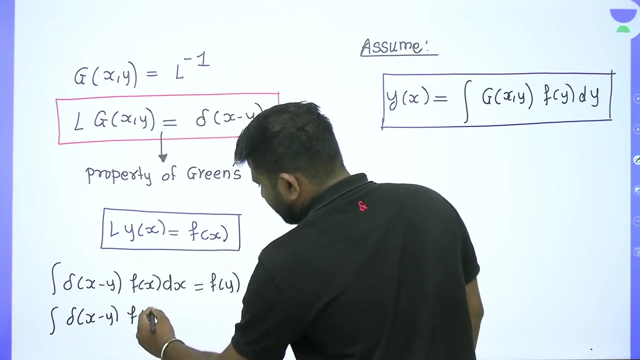 good evening, good evening, good evening, okay. so if you have this, this is f of x, dx. if this is, then what is the answer to this? f of y, how much is its answer? f of y and integration if here, instead of x, x minus y, f of y, dy, if this is then its answer, simply, how much is f of x? 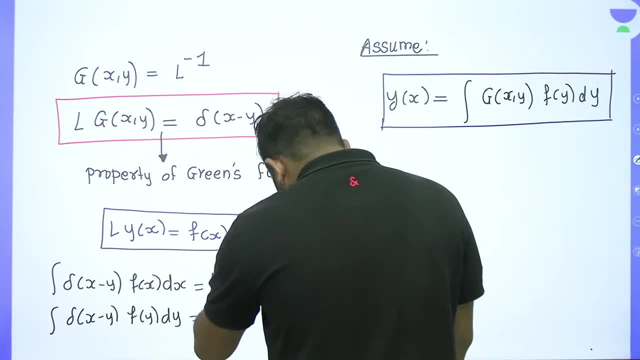 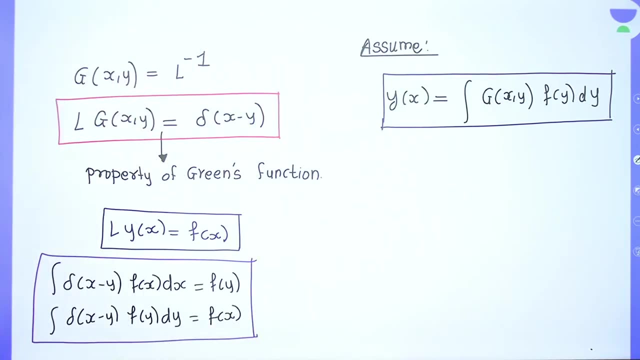 these are the properties of direct delta function. it is important that you know this. if you know this, these are the properties. if you don't know, then you write them down. okay, so these are the properties. this is the properties of direct delta function. so these are the properties of direct delta function, okay. 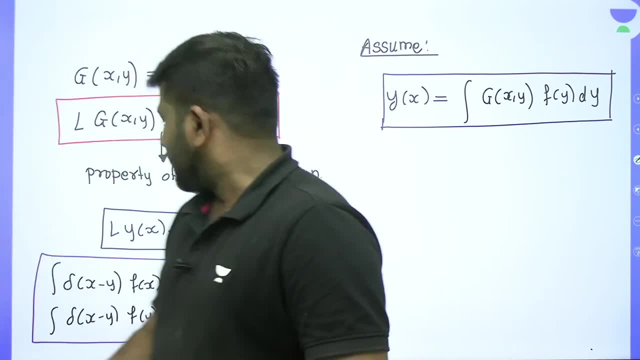 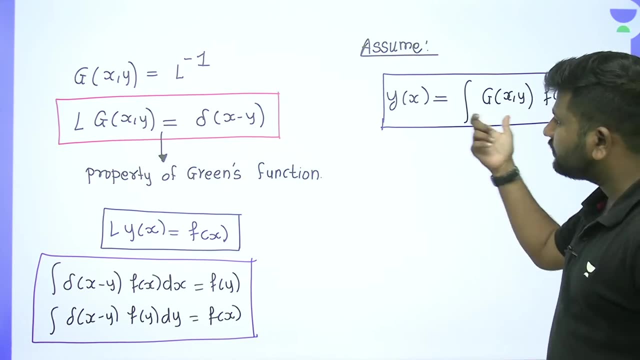 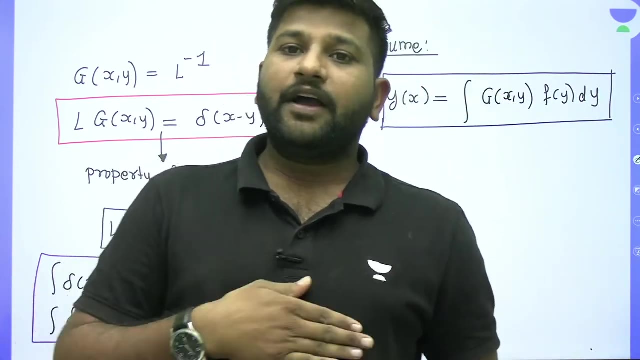 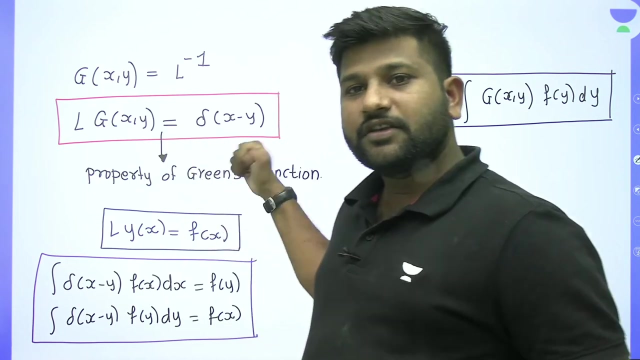 Now what we do is that we just check. we are just going to check that the solution we have assumed is it right or wrong? we don't know. we don't know if it is right or wrong we have assumed, so we should also check that what we are doing is right or wrong. so let's check it and see that our solution is right or wrong. 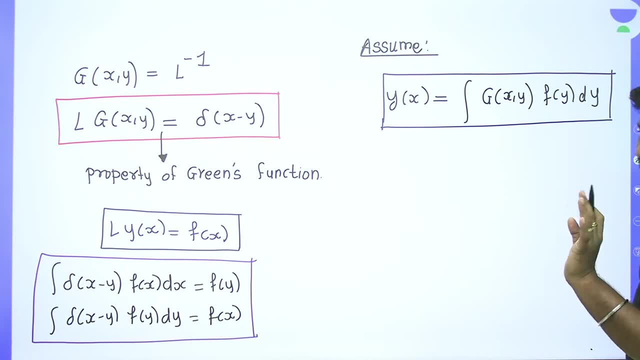 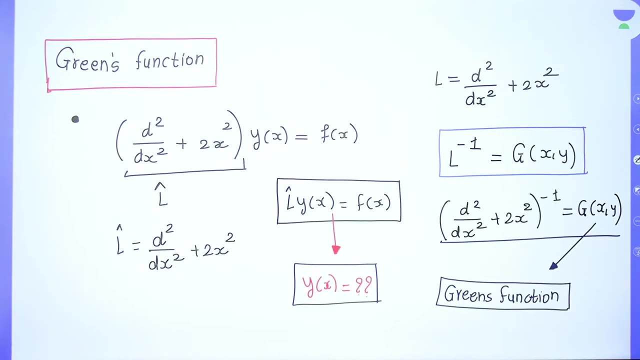 so what we do is that we operate L on both sides. so this is Y of X, is equal to L- into integration G of XY, F of Y, DY. now this L is the function of X, and here the differentiation with Y is there, so we can take it inside. 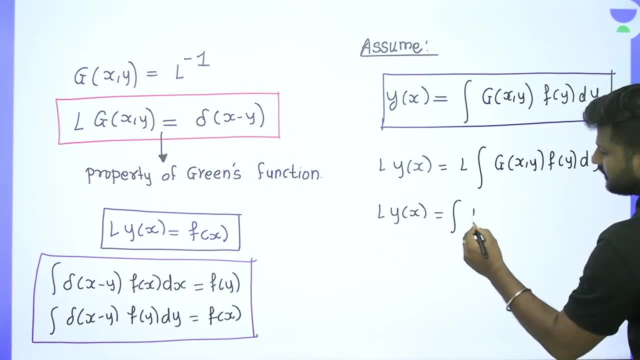 so it will be: L Y of X is equal to integration. L G of X, Y, F of Y, DY. can I write it like this? yes, absolutely, I can write it like this. yes, that means now here, you see, if you see here, then what is this? this is C. 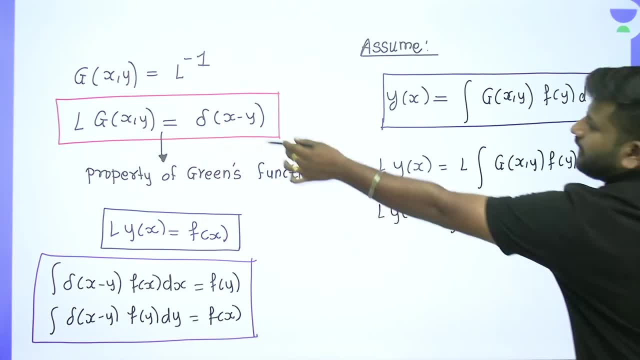 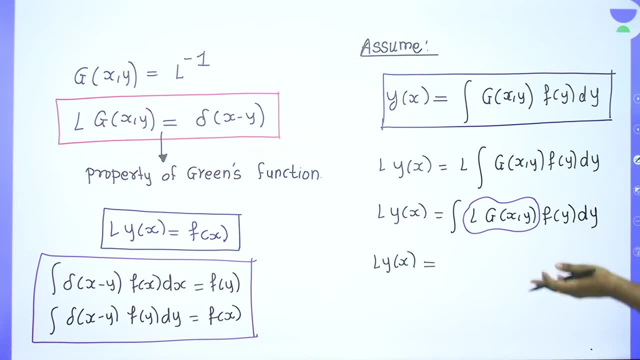 what you are seeing here, then this is not this, then put it in this. then this Y of X. see, let me tell you a little theory first, so that we can't take an example directly. keep some patience, we will also take an example, because all these things are an example for you. 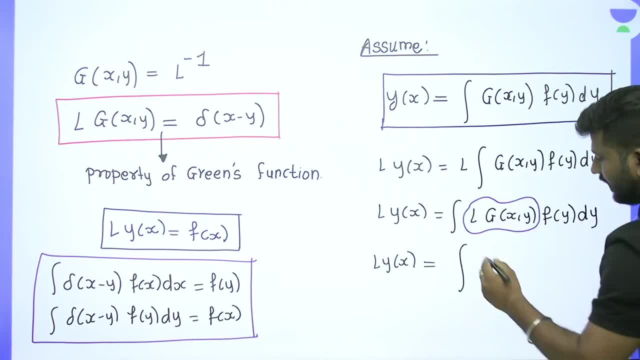 understand. well then L G of what is your Delta? X minus Y here will be F of Y, DY. okay, so use the properties of direct delta function, then use the properties of direct delta function. can you see the properties of direct delta function? substitute it, how much will you get? F of X, okay. 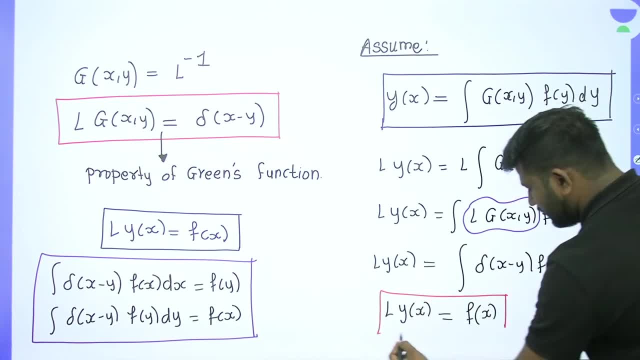 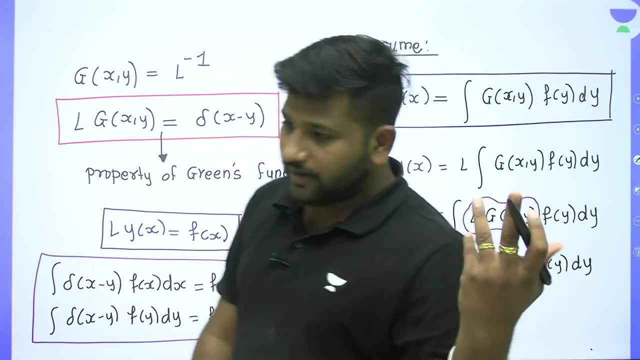 I mean what we got. did we get some interesting things or not? absolutely we got it. this is our function. If we take the solution, then we are getting the same function, which means that it is being satisfied here. so we have taken the solution. this is right. 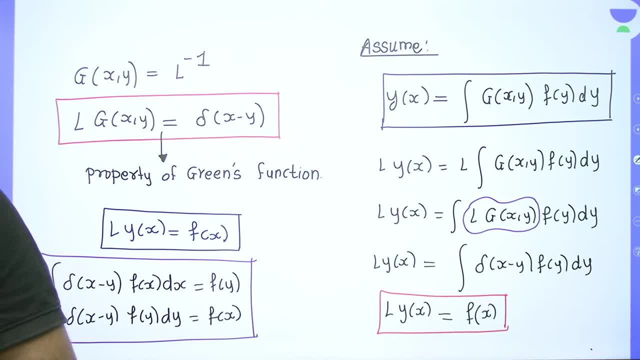 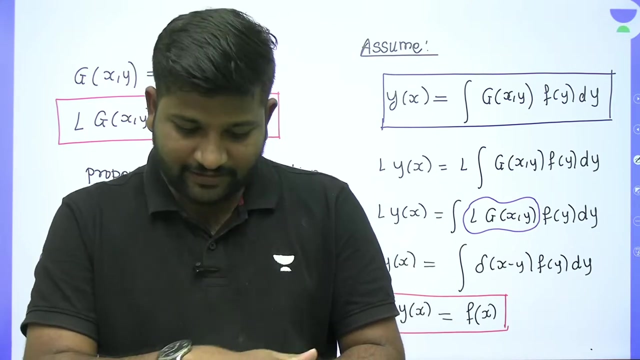 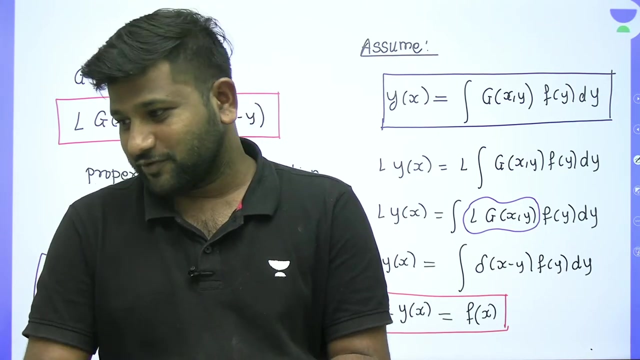 And not ahead. What we have taken here is: our solution is right, As simple as that. We have assumed here and solved after assuming. So this equation is being satisfied. Divya ji, do you not understand math? Oh my God, Math is the language of physics. If you do not understand math, then there are a lot of problems. 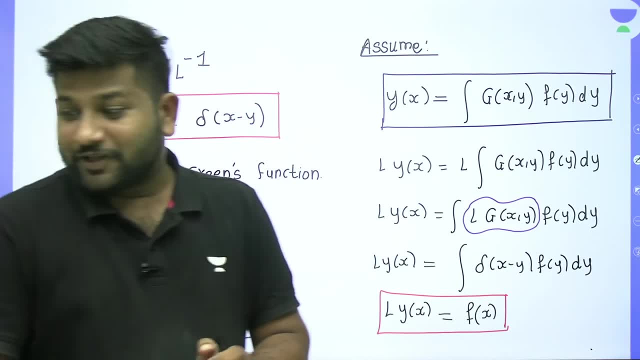 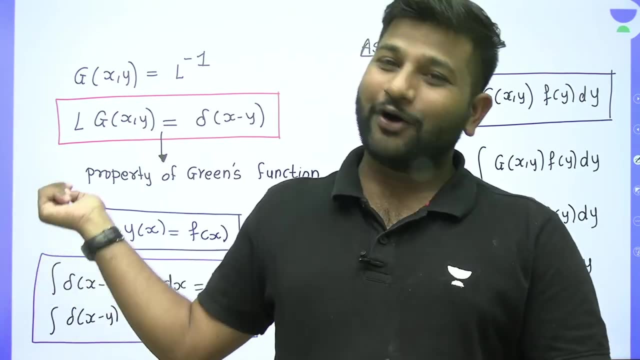 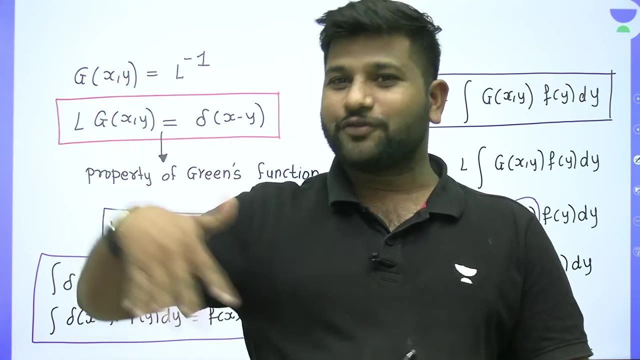 Isn't it How to assume the solution? This solution is not like this. we got up and assumed the solution. There are a lot of mathematicians behind this, This scientist. he took this first, Then after the other. He took this, He took this, He took this. 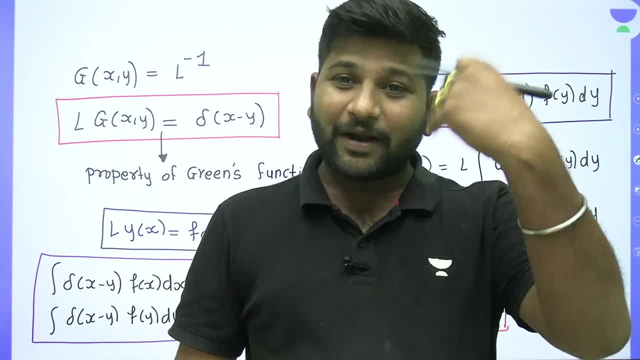 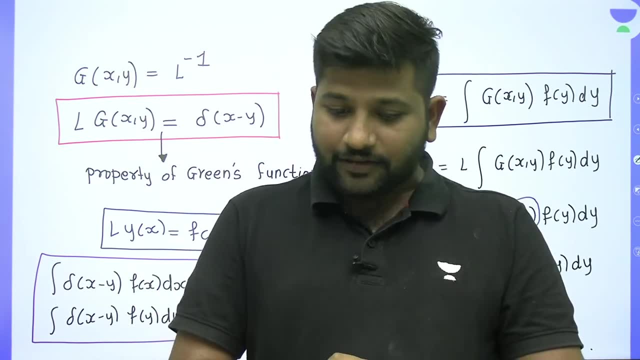 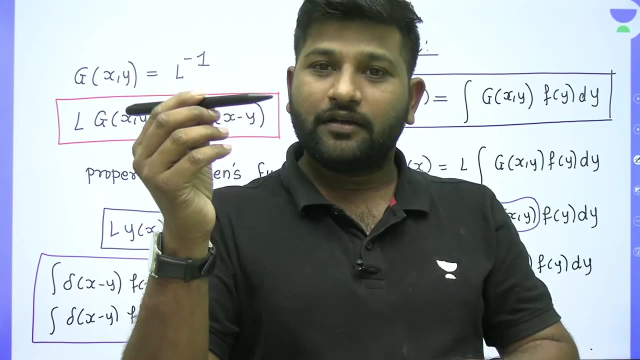 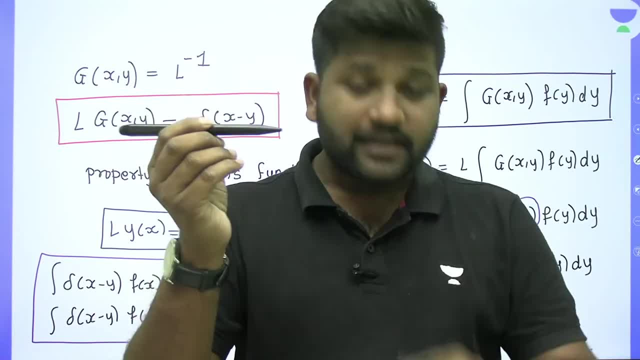 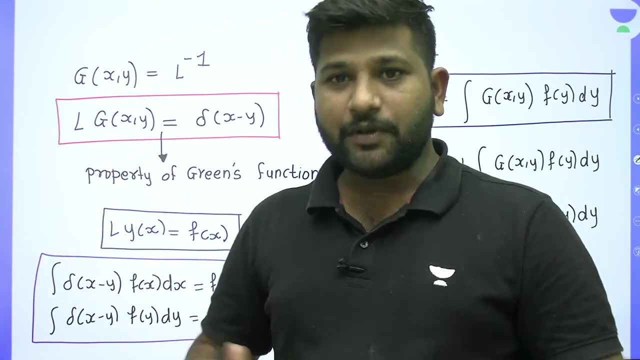 Now which one is fit in this? You will make the first choice, You will assume the second, You will do the third, You will try it many times. then you will have one or two feet. same thing happened here too. this is assumed means many assumptions were made. 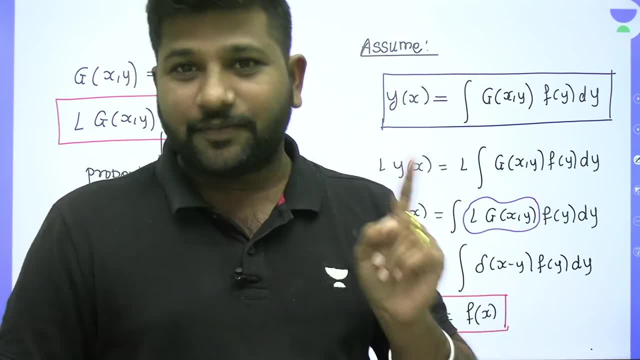 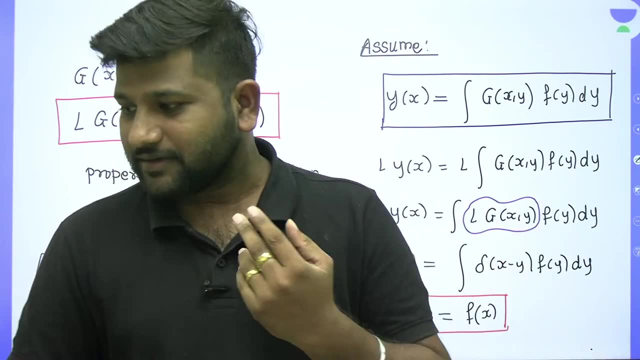 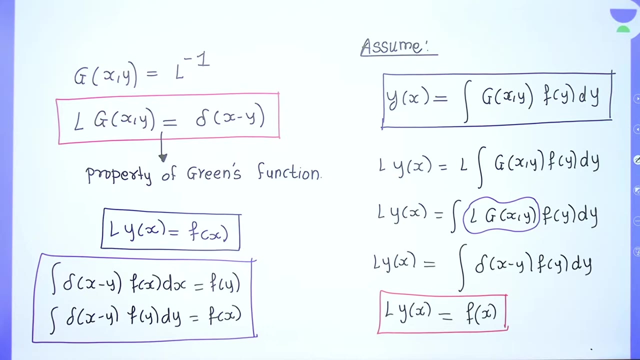 let's say, 1000 assumptions were made, so one of them was satisfying the whole differential equation and we are studying only one rest what we will do of 999? we will not keep checking it. understood my point, ok? I hope you understood this, ok. ok, let's move forward. 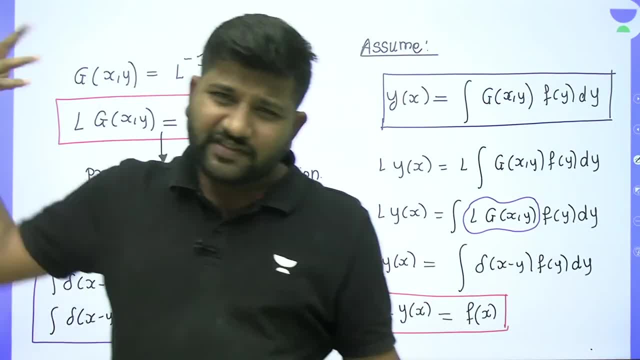 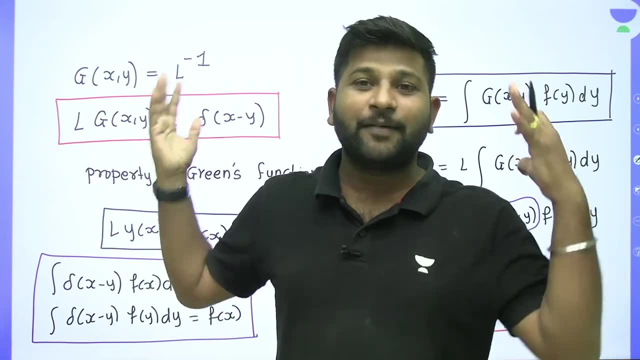 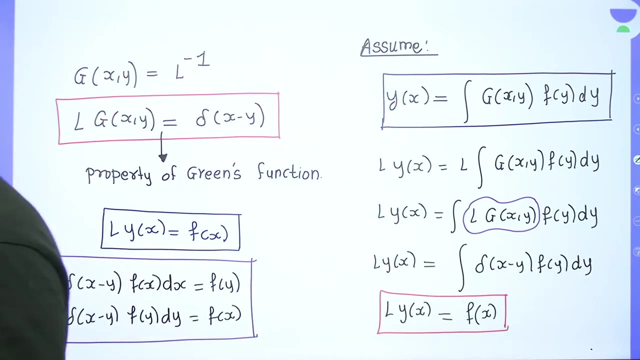 many assumptions were made. not only this much many assumptions were made, but this was satisfied. they were already great scientists, they have made everything for us, so they assumed: if this is satisfied, then we will take it. ok, ok, ok, they are great scientists, they have already worked hard in this. 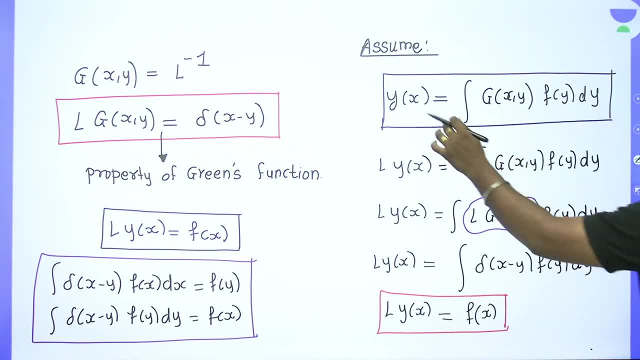 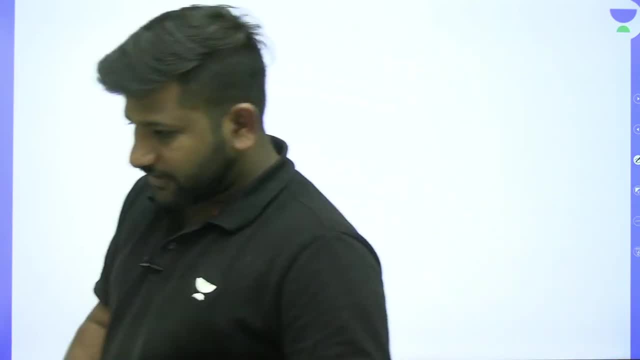 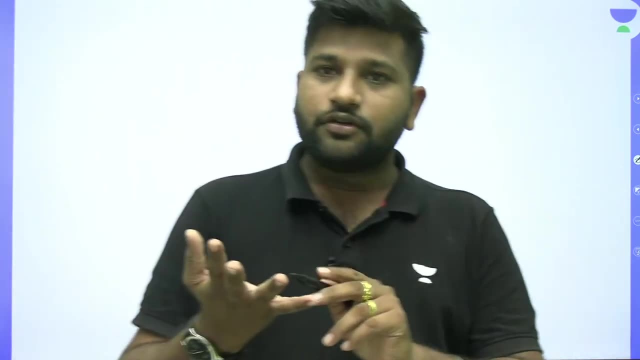 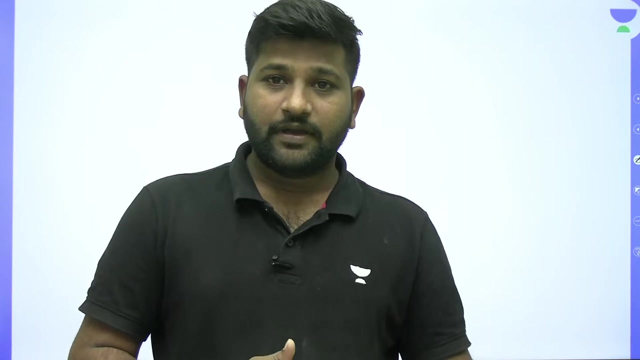 so this solution, this solution will be yours. ok, now let's move forward. you can get two types of questions. ok, now see here you will be asked solution or greens function in the exam. most probably they will ask you about greens function. that for given differential equation, design greens function. 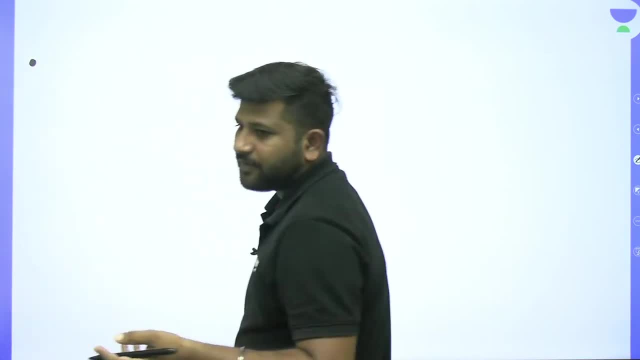 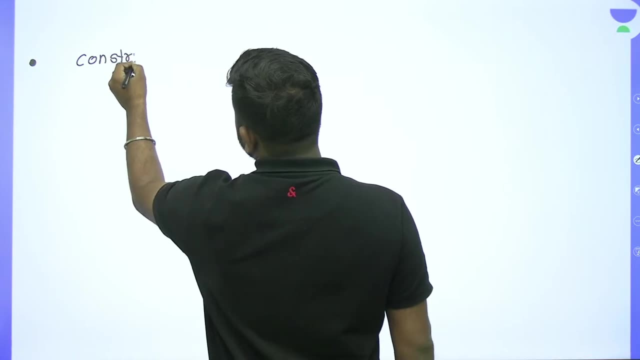 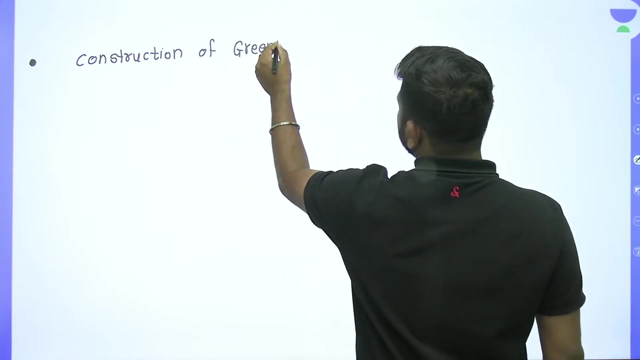 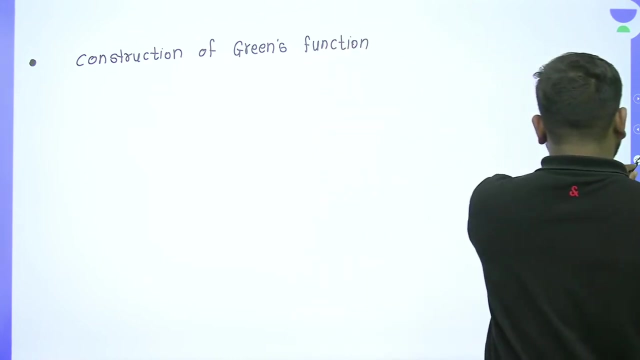 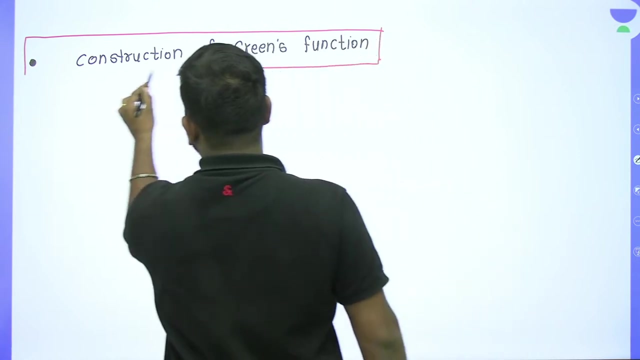 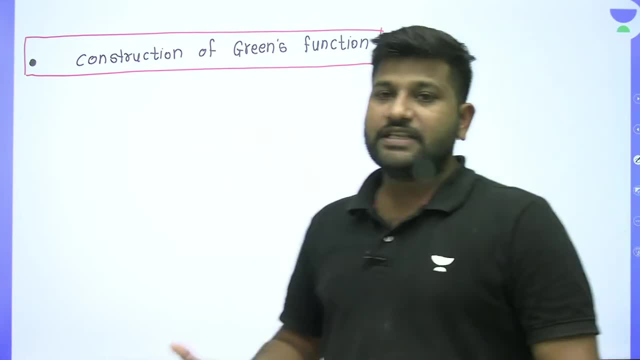 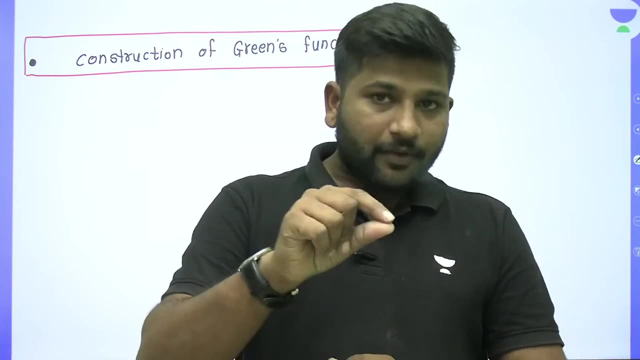 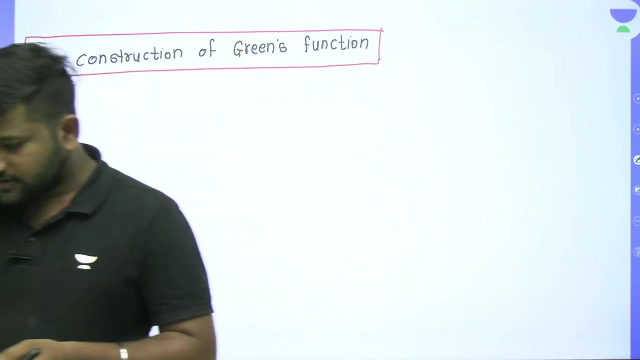 now, what is the need to explain both methods? because sometimes first method is used, sometimes second method is used. now here, first method means there is a little long procedure. second method means we can get the answer of the question with the help of question. ok, I hope you understand. 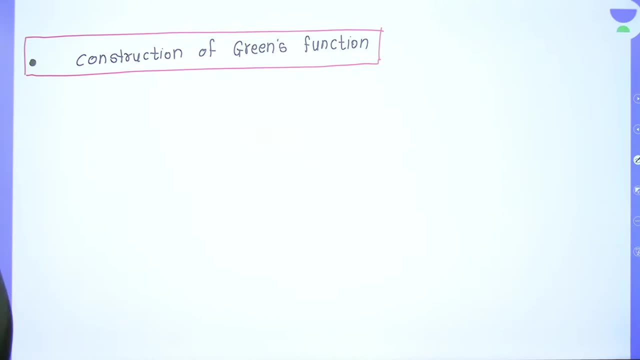 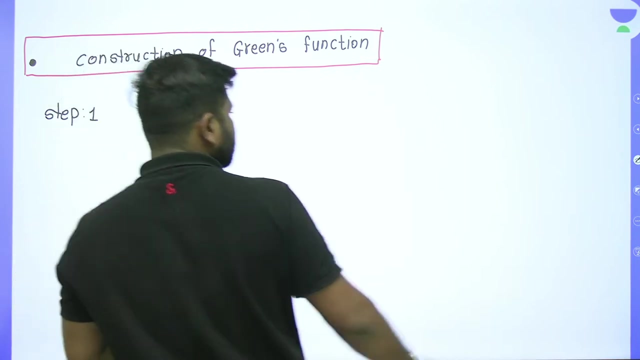 ok, I hope you understand. I hope you understand. I hope you understand. so, how we will construct here. so we will discuss about step number one and what should be your step number 1, and follow these steps and this step. see till when I wasn't taken an example. 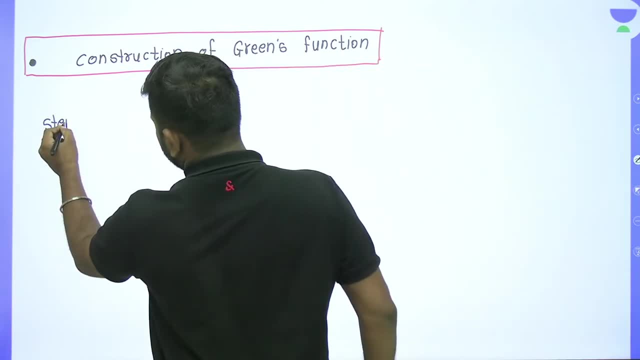 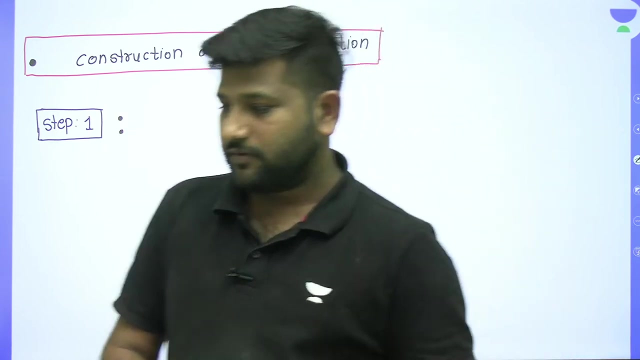 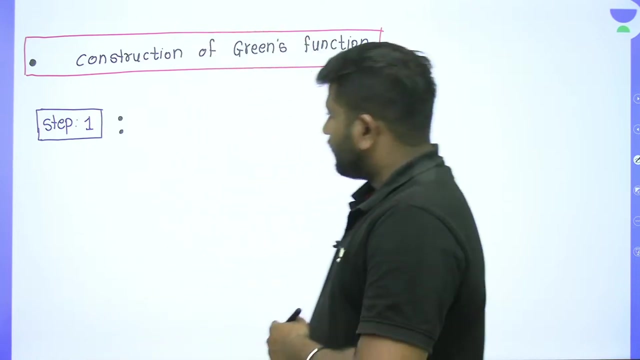 you remain in a little confusing state. you also think that why this condition of CSR? So if you want to be clear, then, till the example is done, be patient, I will discuss each and everything. So, step number one: what should be the step number one? okay, okay, let's go. so step. 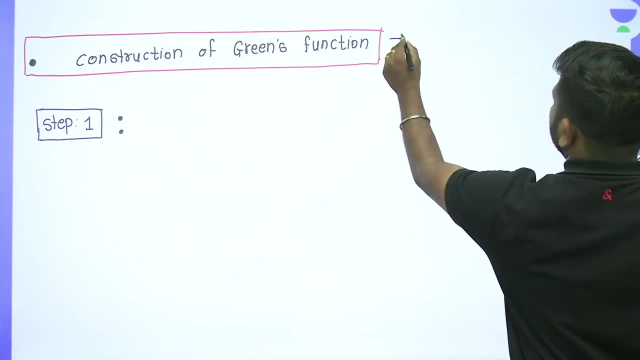 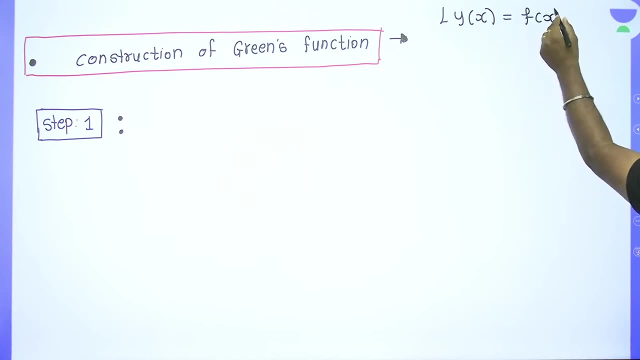 number one now, when we are going to design the Green's function here, then the differential equation will be given to us. that is, this will be given to you and along with this, you have a boundary condition in the differential equation, which is a boundary condition: you. 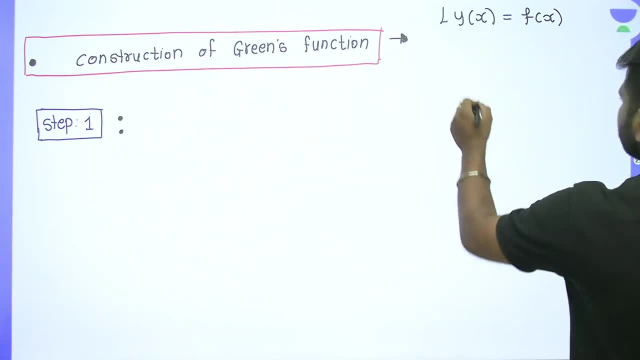 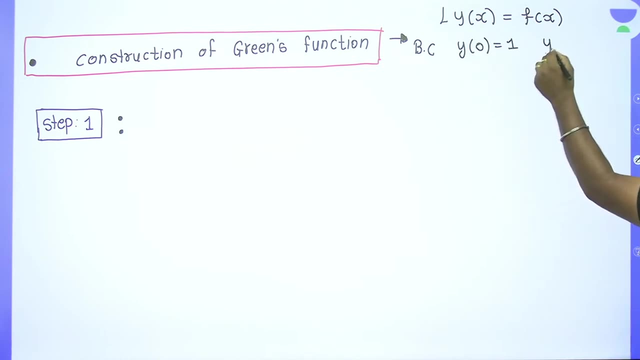 will be given. okay, so they will give you the boundary condition also. boundary conditions are also given. so let's say, y of 0 is equal to 1, y of, let's say, l is equal to 3, so this boundary condition, this boundary condition will be given to you in the example and for 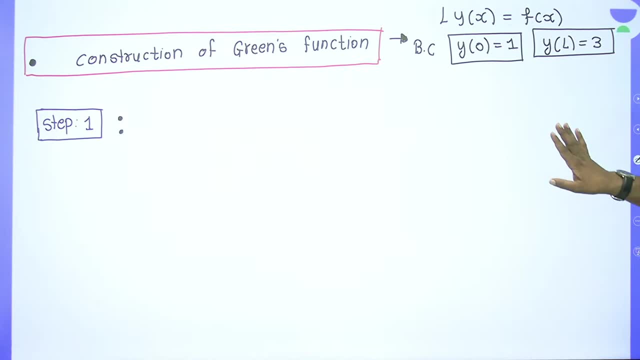 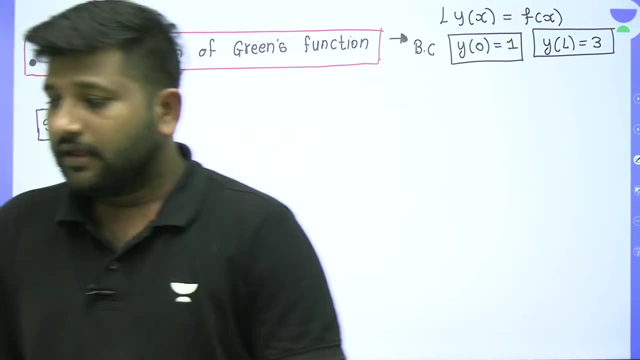 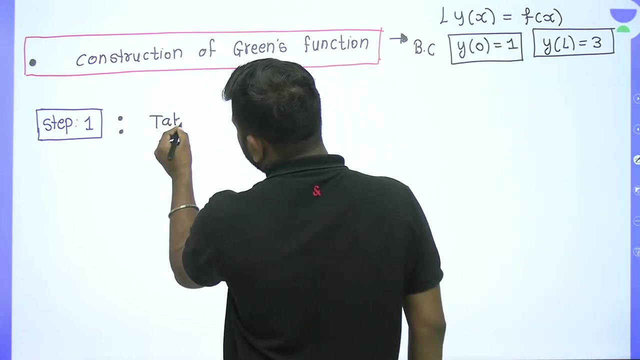 this boundary condition. this is not a new thing. this is a well-known thing to everyone, so this will be given to you in the example, you do not have to worry about it. okay, step number one. so what is step number one? take homogeneous equation. take homogeneous equation. 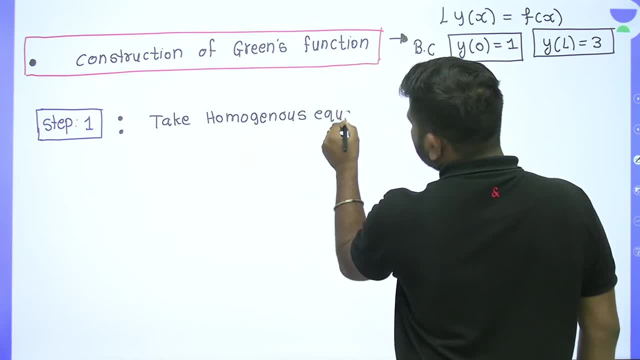 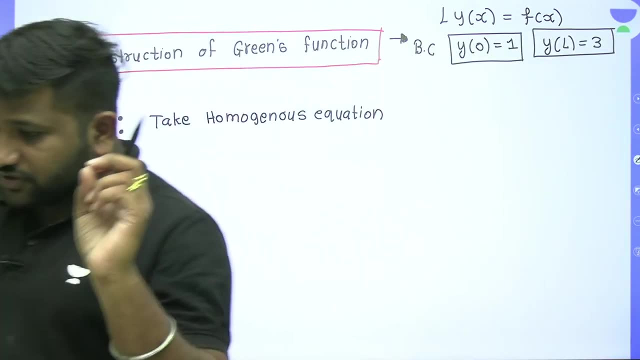 homogeneous equation, sir. what will happen if it is non-homogeneous? first let's discuss for homogeneous, let's discuss for non-homogeneous. So take homogeneous equation, then you have a homogeneous equation. okay, you are 13 years. 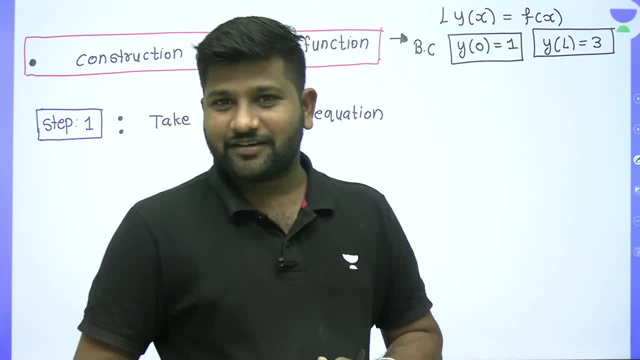 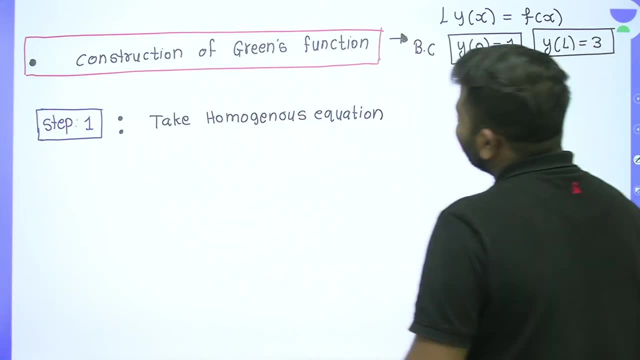 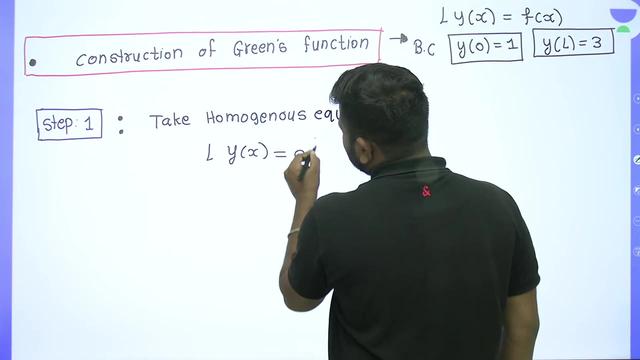 old, that means you are in 6th standard, 7th standard. then why are you looking at this class? you will not even understand anything. so y of x is equal to 0, this is a homogeneous equation. okay, this homogeneous equation. this homogeneous equation you will not understand. 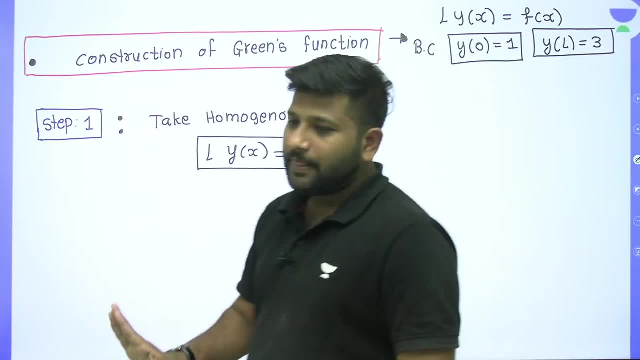 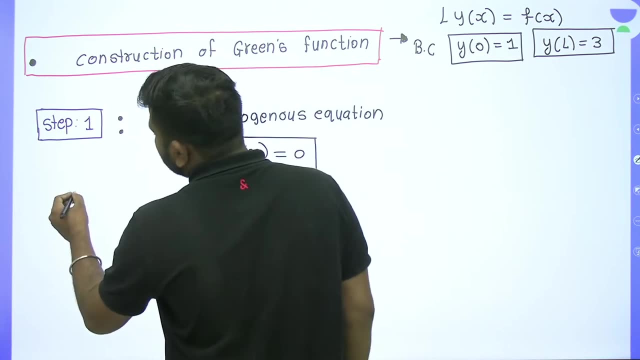 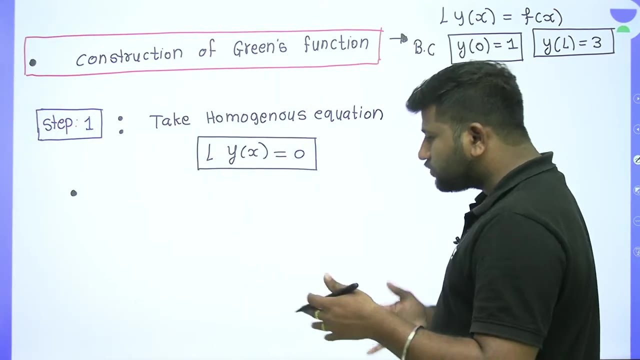 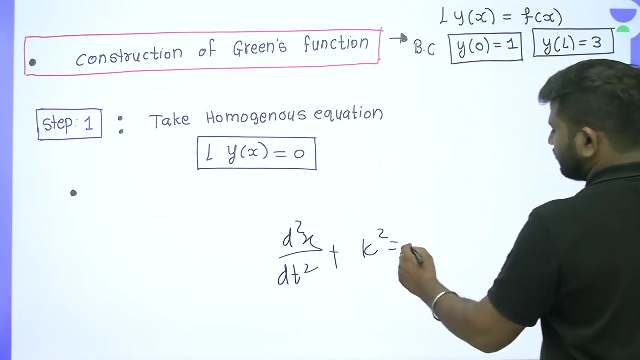 who knows that if now you are learning anylafya, then you will even learn these basic functions. then what I have to do now? then I will go further and say that you have to do this here, you have to learn about it. 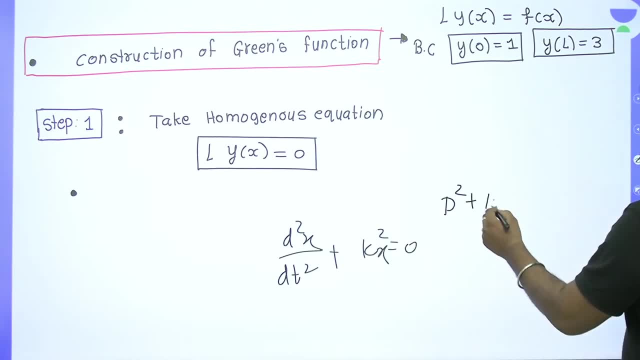 How to do there. you will know What I'll do next. then I'll explain you. you will not understand. Oh no, no, i won't. ok, i completed my prep in this already. so where is the function? can? square x is equal to zero. that means d square plus k square is equal to zero, so d is equal to. 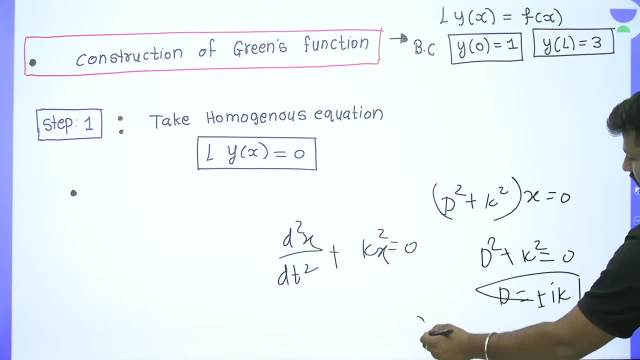 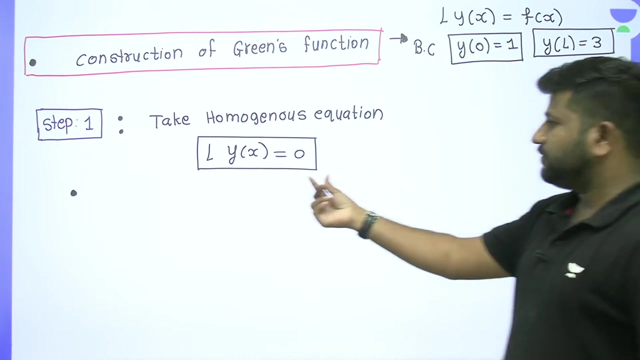 plus minus ik, and then its solution is solution a into exponential, something plus b into exponential, something so differential equation. you need to have some idea, because we have to find out the root of this equation. so what we have done here is that we have taken this homogeneous equation. 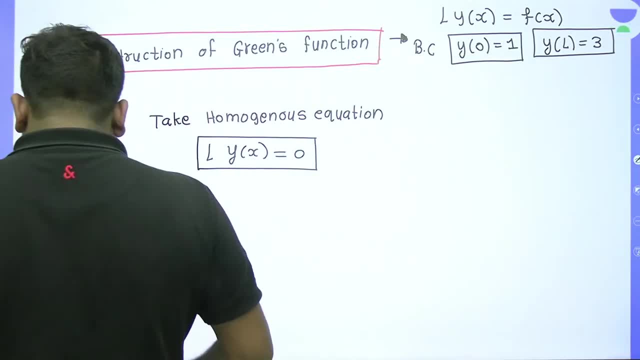 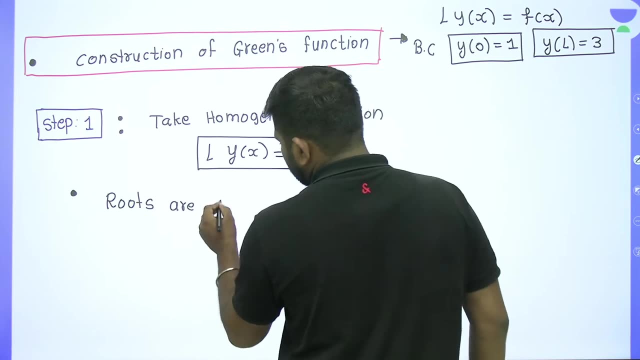 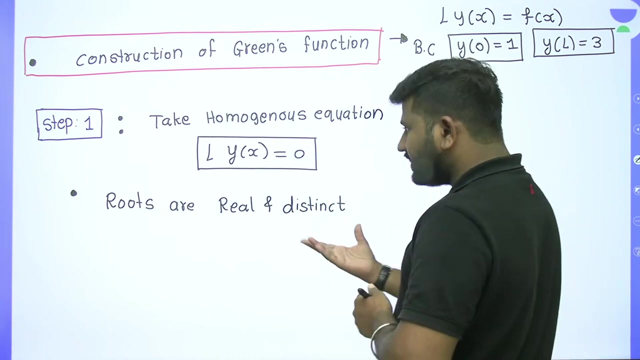 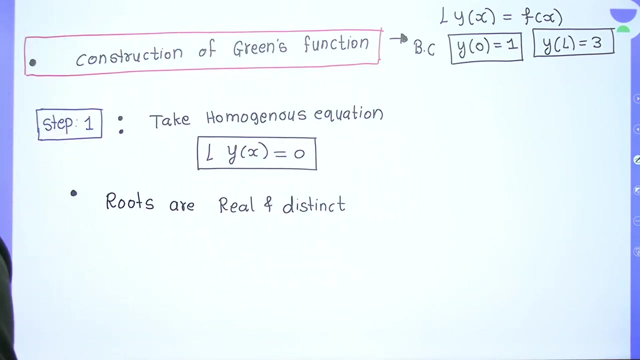 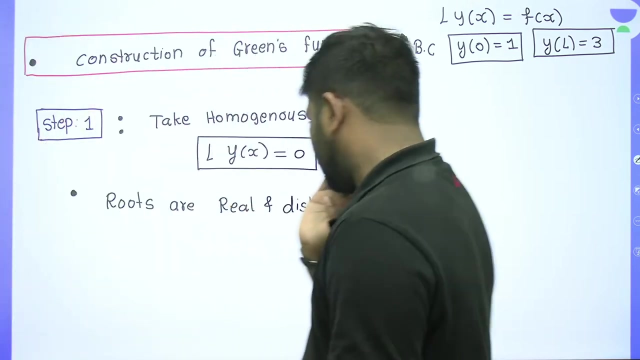 ok, then there are two types in this too. you know that roots are. roots are real and distinct. roots are real and distinct. if roots are real and distinct, then what is the solution to all this? we all have some idea about this right of differential equation right, and so roots. 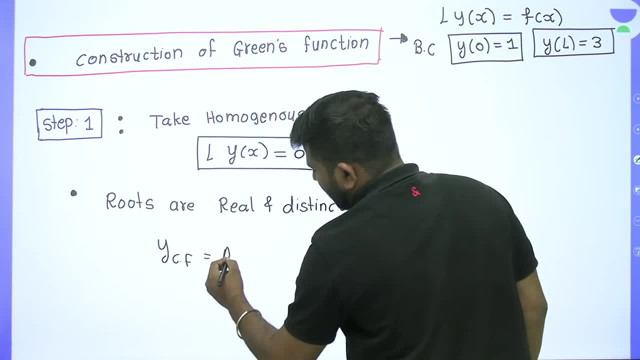 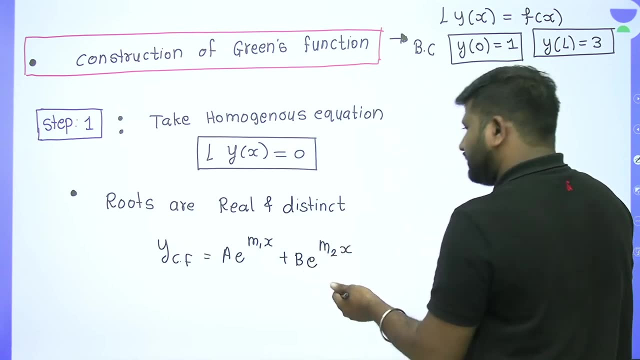 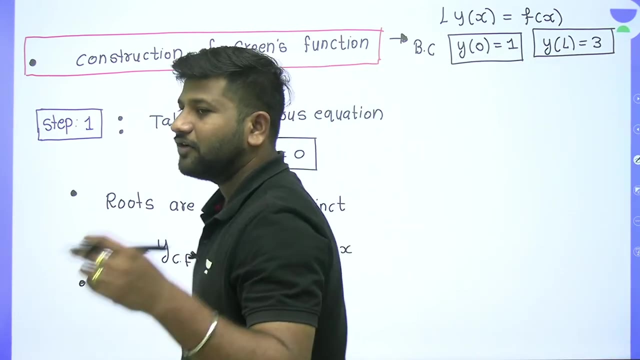 are equivalent to its Y complementary function. what is your a into exponential m1x plus b into exponential m2x? so these roots. you will have the idea about this right. and second is that if your root is complex, then its root will be very complex. if your root is complex, 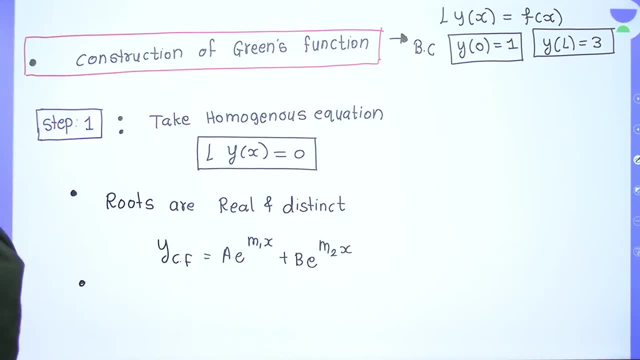 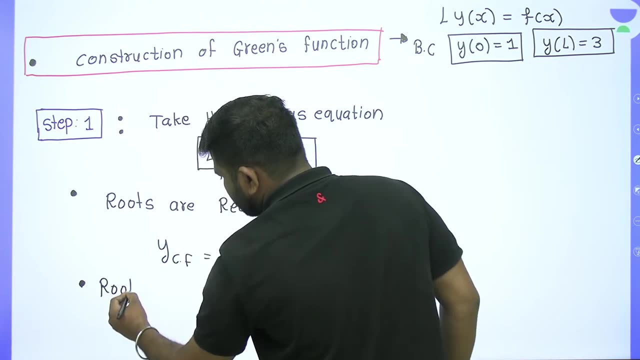 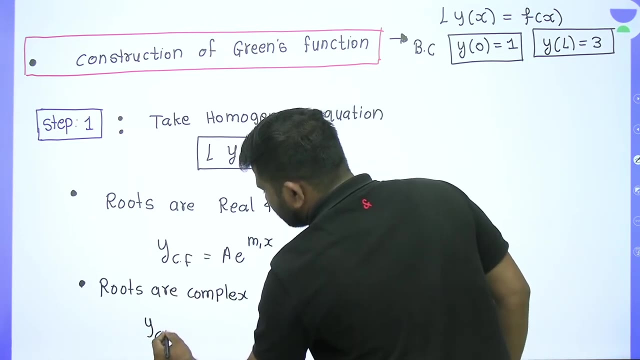 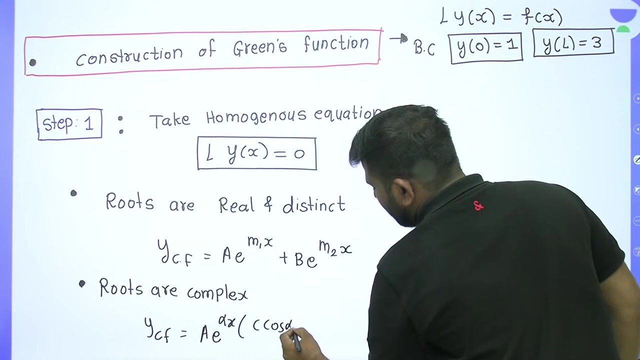 then what else is there to see in such a relationship? what is the root of here? since if roots are complex, if roots are complex, if roots are complex, then y complementary function is a into exponential alpha x, into c cos alpha x plus d sin alpha x. so this is the 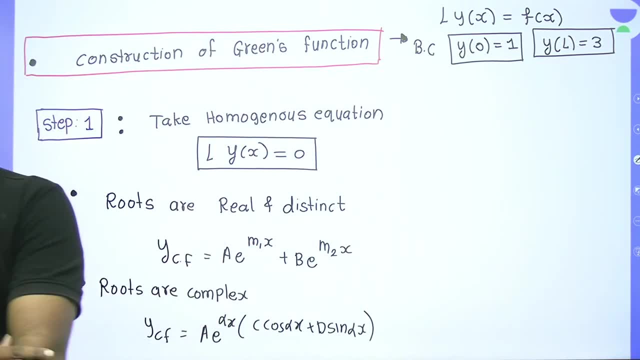 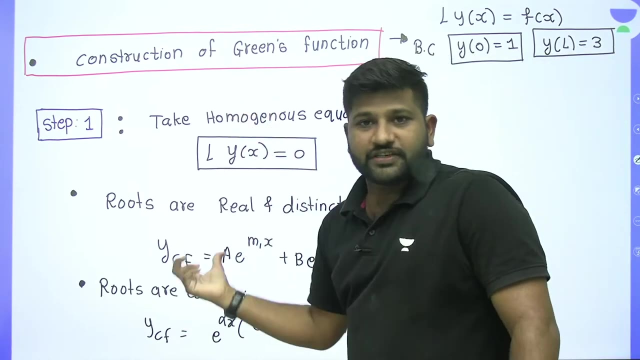 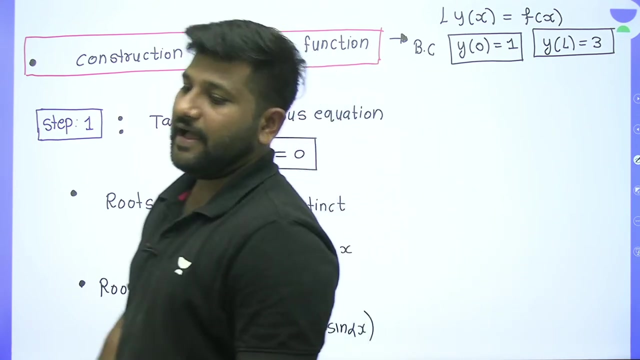 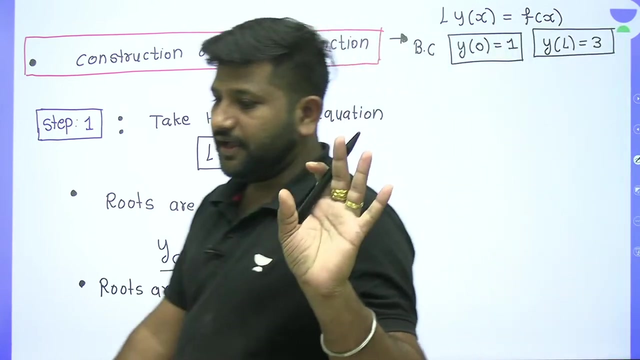 solution of homogeneous differential equation. ok, so this is the step number 1. so you have to take homogeneous differential equation, so you have to solve it. so roots will come, so complementary function you have to design now see here. now what is the step number 3? see: 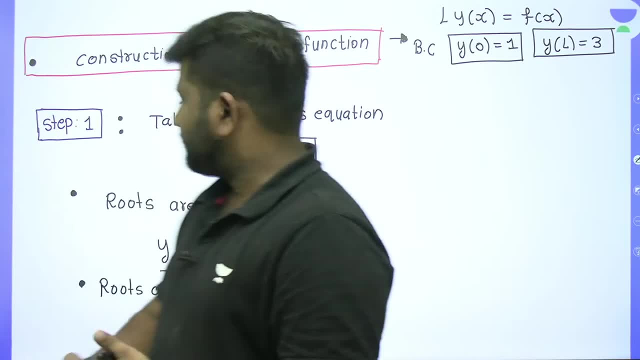 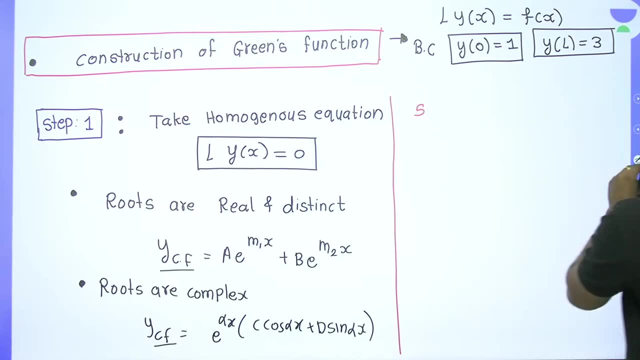 now step number: step number 2. step number 2. what is here? see carefully. this is step number 1. now what is step number 2? step number 2. these are the steps that you have to follow, step number 2. so step 2 will be this. 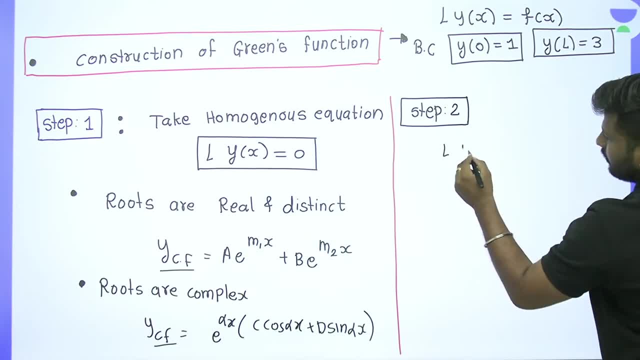 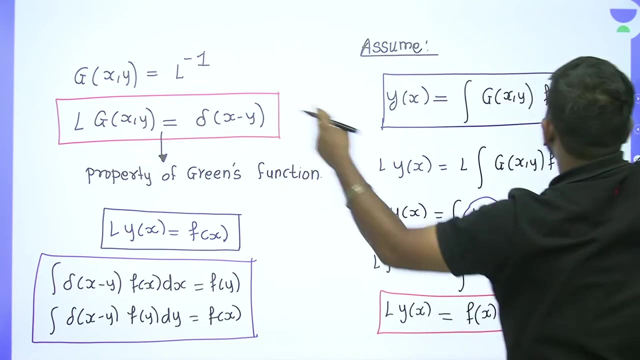 see, this is: l y of x is equal to what you have, f of x. this is you have, ok. ok, that means, if we see, here we have written l g of x, y, so which is equal to delta. so l g of x, y is equal to: 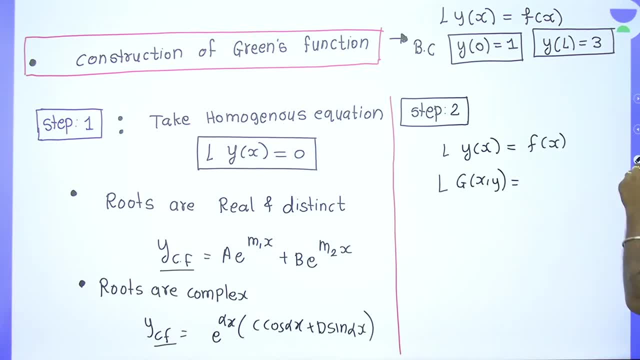 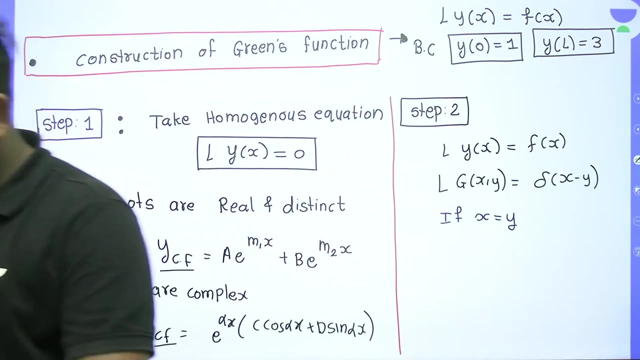 g. this is direct delta x minus y. ok, so you all, if I take if, if x is equal to y, if x is equal to y, then what will happen? if x is equal to y, then what will happen if x is equal to y, if x is equal to y? 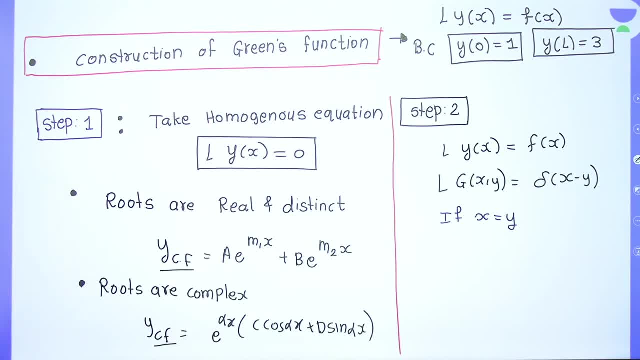 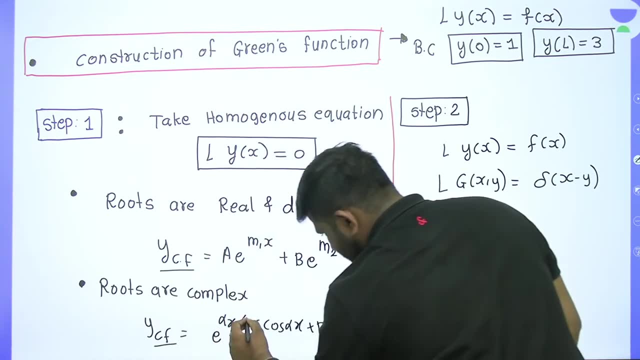 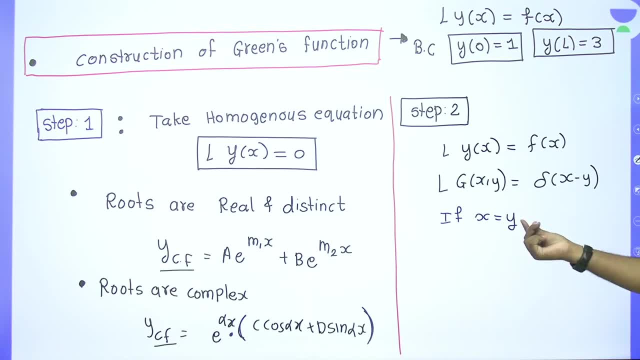 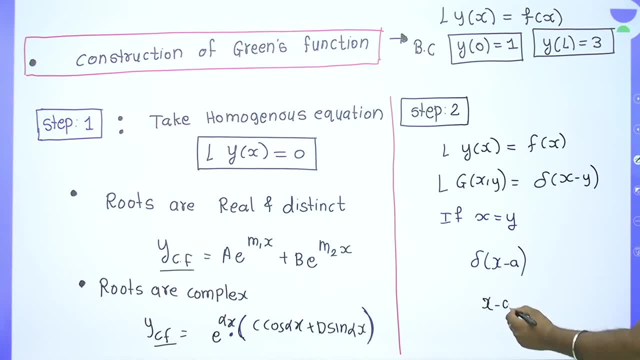 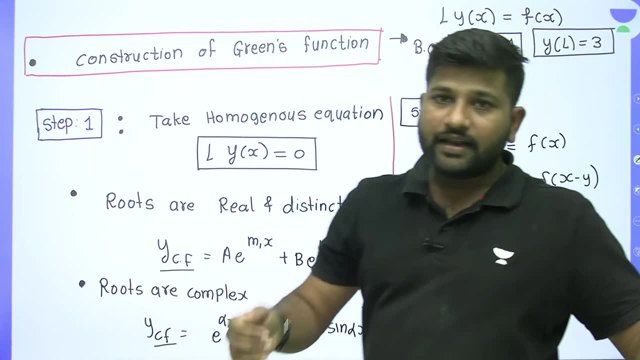 then what will happen? if x is equal to y, then what will happen? if x is equal to y, then what will happen if x is equal to y? on x is equal to a, the peak of direct delta will be there. the peak of direct delta will be there. the infinite value will be there. 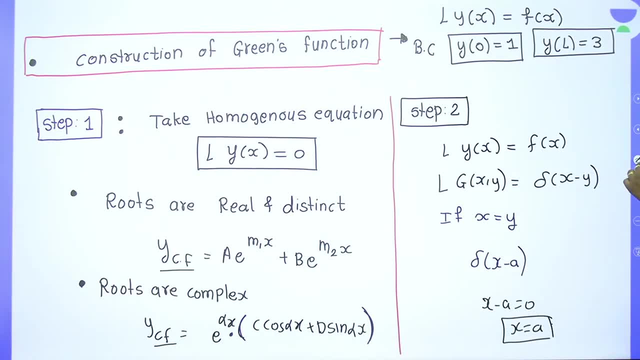 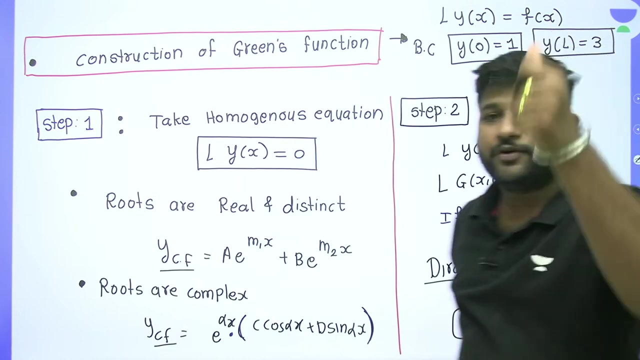 so similarly, that means if we take one thing in our quantum mechanism, if you remember, then see this direct delta function. in the quantum mechanism we see the direct delta function that if x is equal to a, If there is a peak, then how much potential was there? how much potential was there? infinite potential was Non-dimensional. 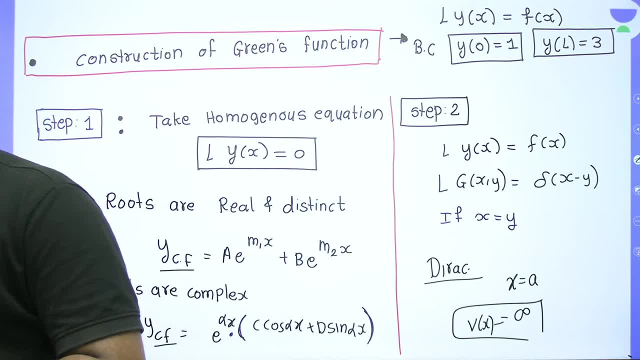 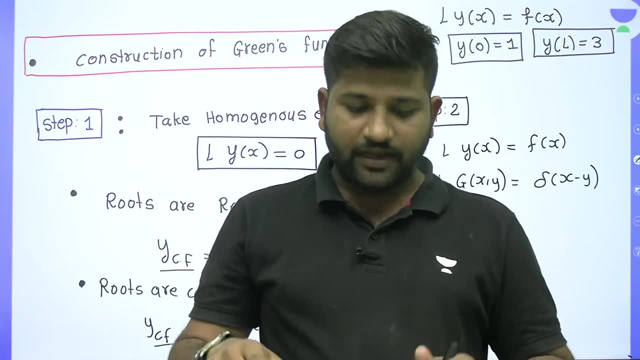 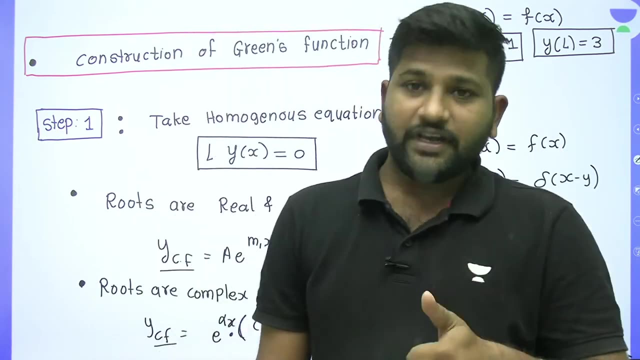 direct delta function. direct delta function: if you have non-dimensional direct delta function in quantum mechanism, then there is peak and the value of the potential on the peak is now infinite. then, where the peak is, the value of the potential on peak is infinite. so there is infinite potential. so itsment is square. 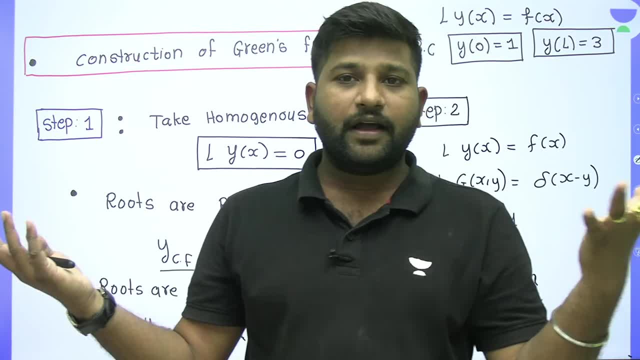 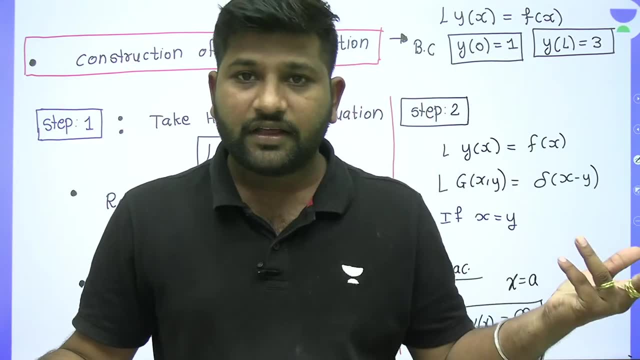 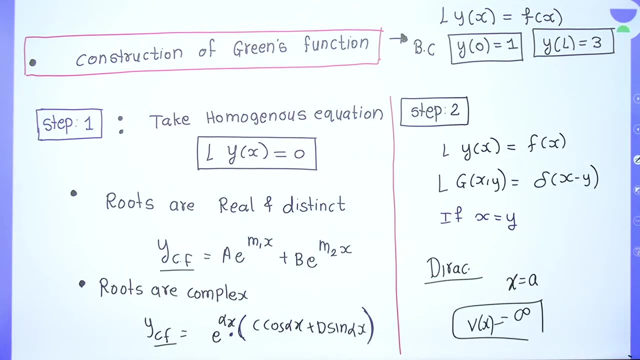 Tradition must apply to infinite potential. so great numéro 9. Is it not simple to simplify the equation of Scrodinger? Even Scrodinger did not know how to solve. the equation of Scrodinger on infinite potential, Everyone is coming to know. So here the same thing is happening. that at x is equal to y. what is its value? 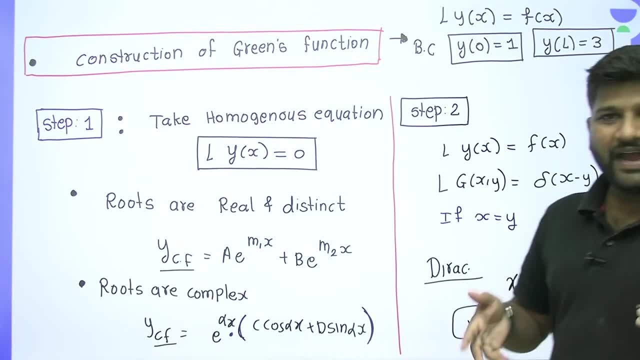 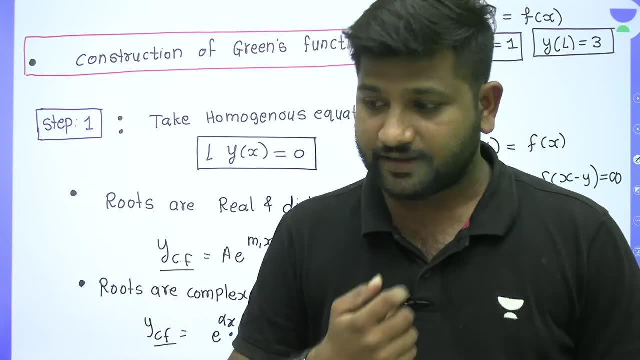 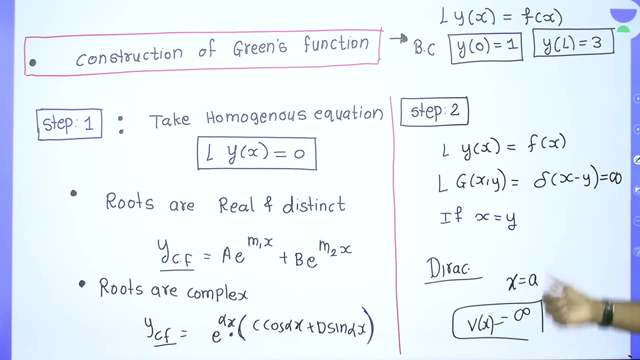 Here its value will be infinite. It is not infinite, but very large. That means at x is equal to y. we cannot define the solution. Do you understand? Here at x is equal to y. where is the peak of direct delta? At x is equal to y. 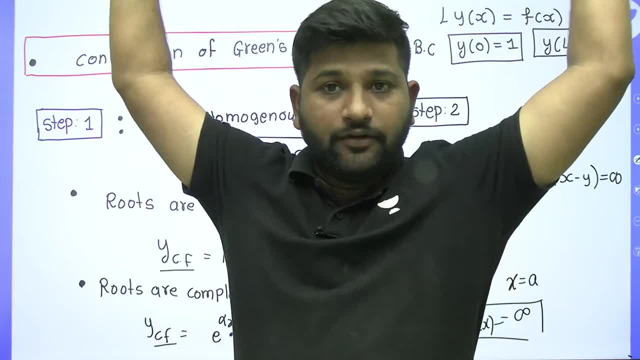 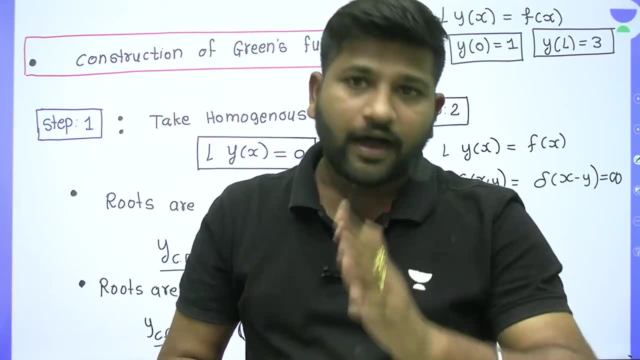 And at x is equal to y. peak means infinite value. Infinite value means very large value, So it is a very large value. How can we define the solution there? We cannot define the solution. That is why what happens here is that we approach y. 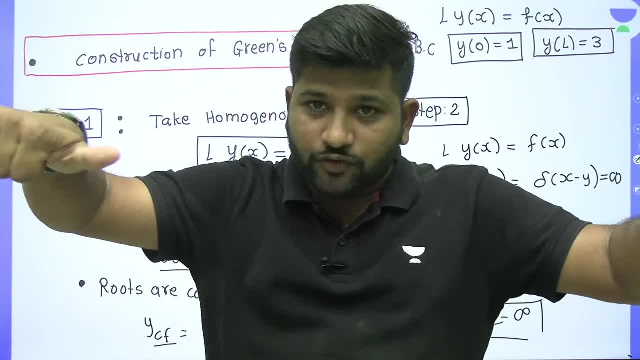 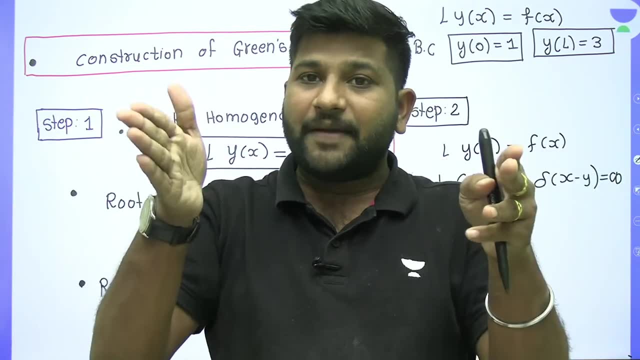 As we did in direct delta function, we approach towards that peak. We will approach that peak And as we approach that means we are taking epsilon here and epsilon here, So epsilon tends to zero. We will take this limit and find its value. 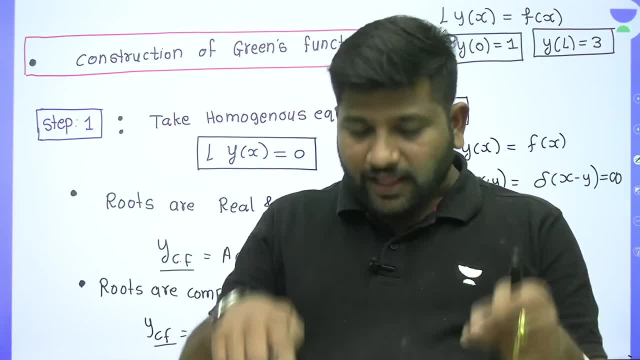 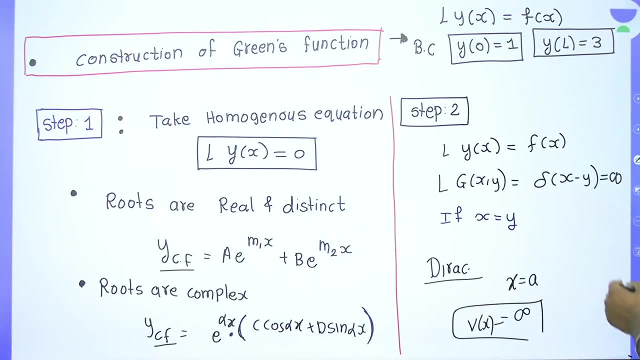 And that value will be that where the peak is, there will be so much value. Do you understand what I am saying? Okay, That means here also: at x is equal to y. the solution will not be defined here. Okay, Let me draw a line here. 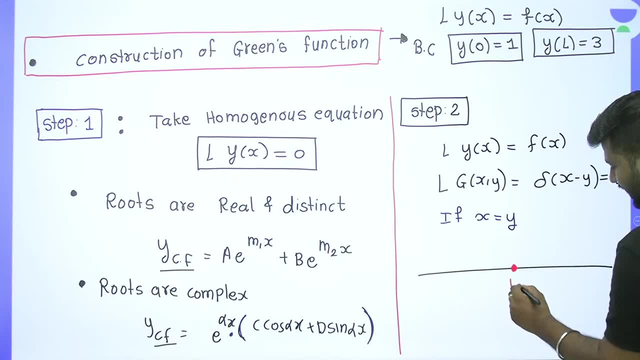 And if I take here, this is y. So if I take here, this is y. Do you understand? Let's say, if I take this y And if you see here what will happen in this, What is the solution here? 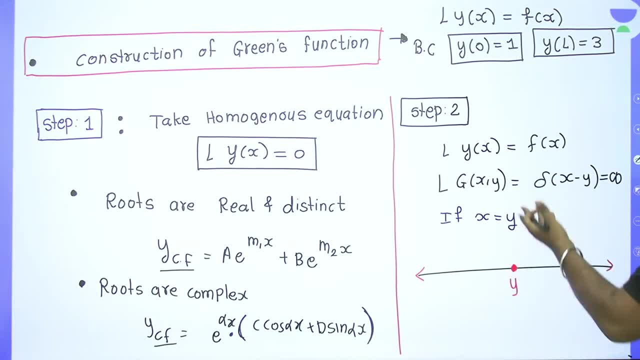 So here we cannot find the solution because it is an infinite value. So what will happen here? So this will be one side. We will find the solution on this side And we will find the solution on this side. That is why it has two parts. 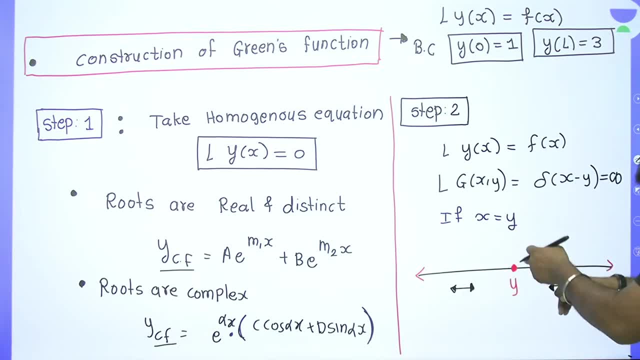 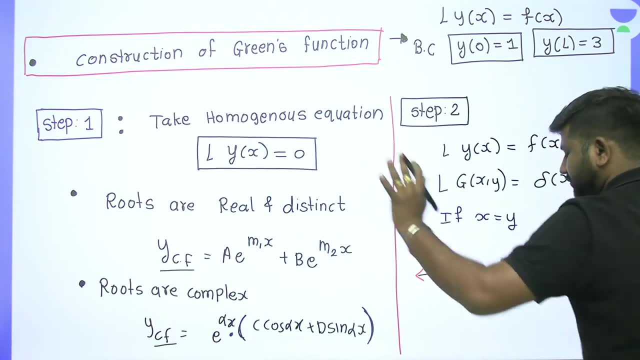 One is this part and the other is this part, Because there is an infinite value here. That is why we are not going to solve that. We cannot solve there. Do you understand? Now, this is y, So what will happen here? This is: x is less than y. 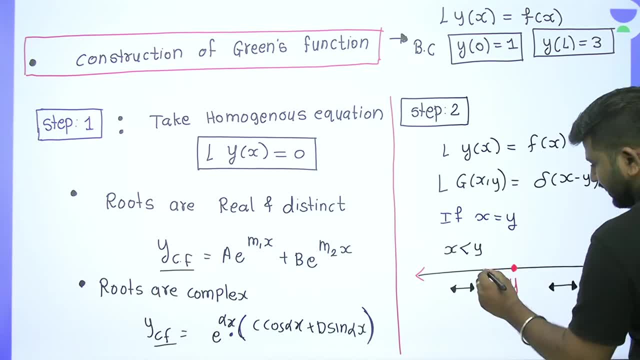 That means, if I take this point here, So if I take this point, then this point is less than y. So this will be one region And here will be one region That I took any point here That is greater than y. 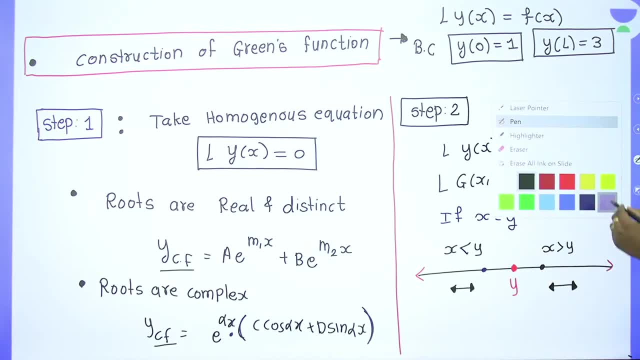 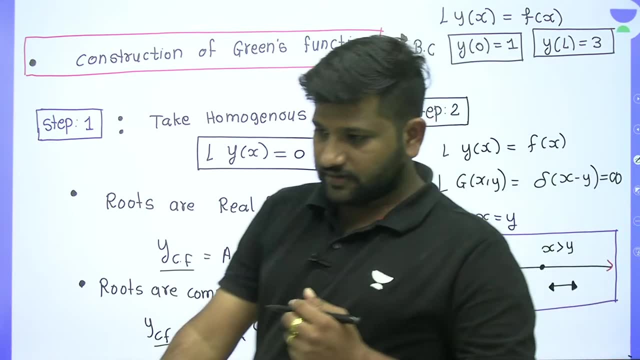 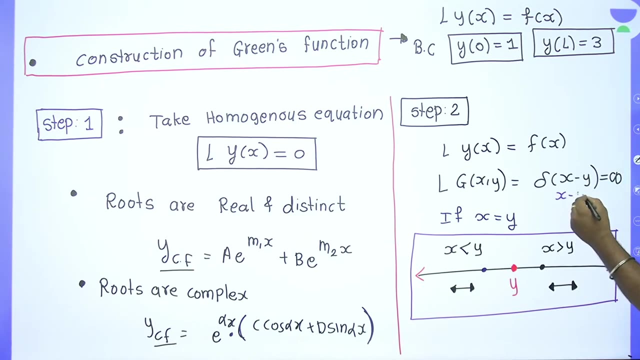 That means x is greater than y. So we got these two regions, And in these two regions we have to find out the solution. Okay, Yes, x is equal to a peak, But here y is there. This is x minus y. 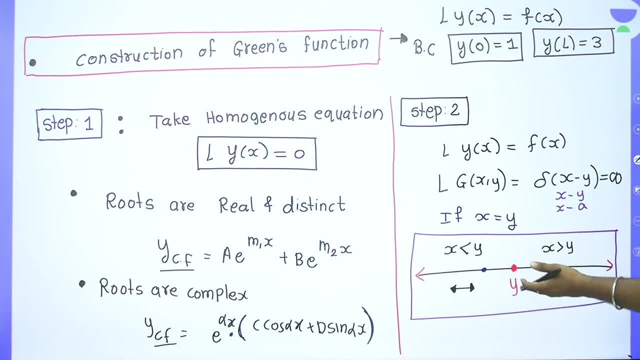 Let's say we replace y with a. That is simple. So here y is there. That is why we took y here. If here was a, then we would have written a here. Okay, So these are the two regions. Now, if you have given the question of CSR. 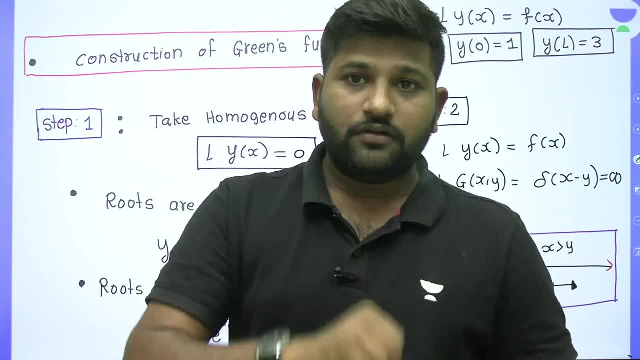 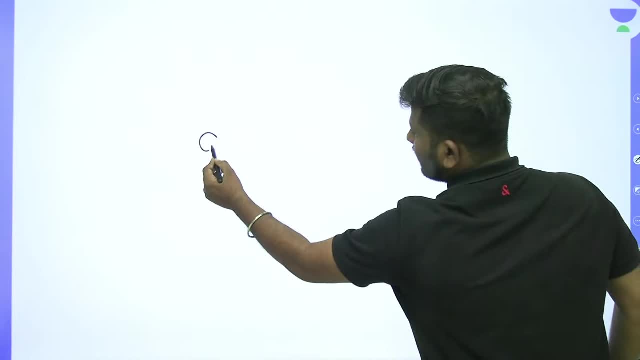 If you have given the question of CSR, Then in the greens function two solutions are given to you. Two greens functions are given to you, Right? If you have seen the previous year question, Then you will have this: That G of x, y. 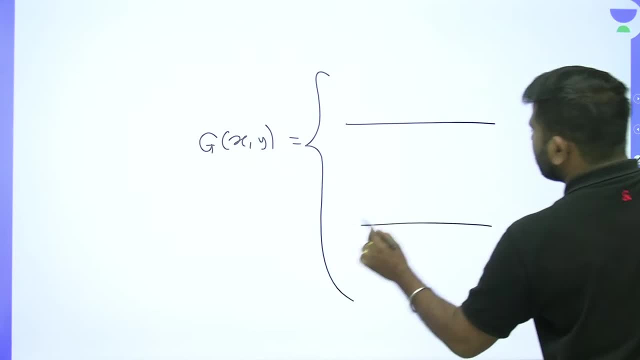 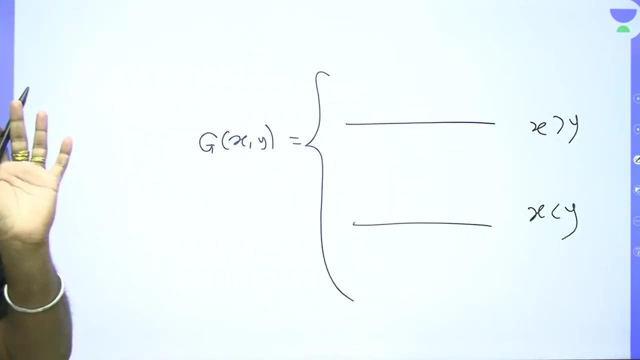 And this will remain to you. Here is one answer, Here is one answer. And here it is written that x is greater than y And x is less than y. Why does this remain? This is its region, Right? Okay, Shivankar ji, we are not talking about direct delta. 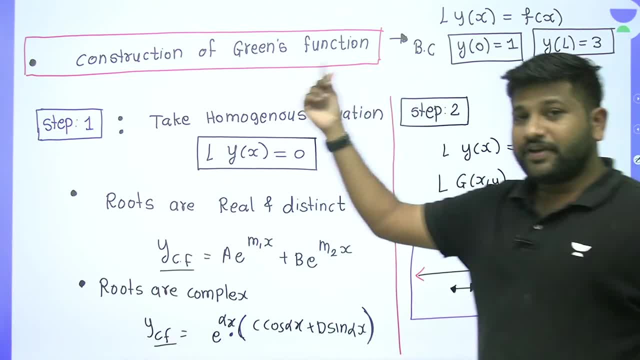 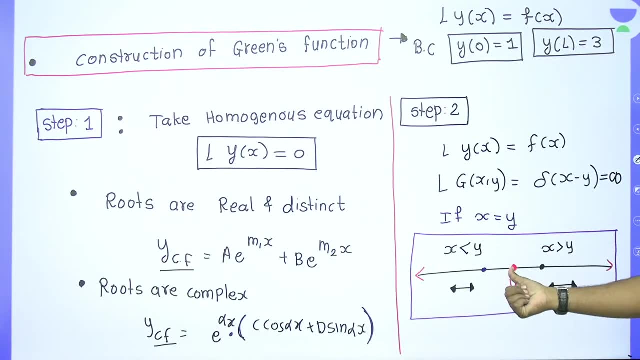 We are talking about the solution of differential equation. Right Here, direct delta is not defined. Okay, We are talking about the solution here. What will be the solution on this side? What will be the solution on this side? We are talking about the solution of differential equation. 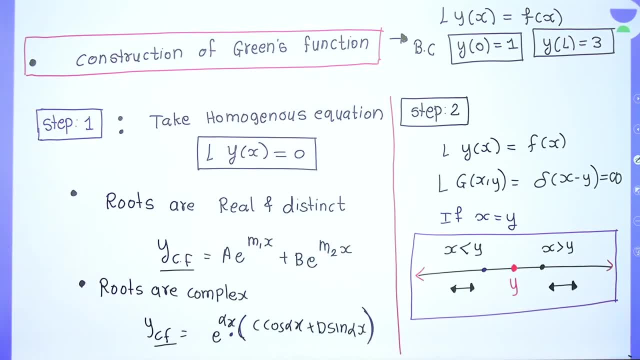 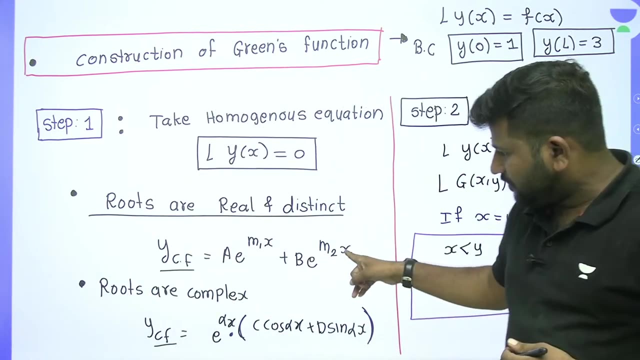 Okay, So this is your second step, Do you understand? Okay, Then what will you do here? This is So here, Let's say, I assume that we have taken the complementary function And in the complementary function. So the solution of this is this. 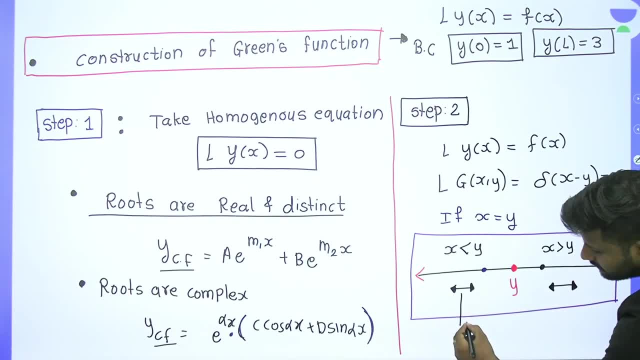 So how will you write in this region? Can you see this or not? I don't know. Can you see this much below? Let me check. Hmm, I can see. Right, I can see a little below. So what will happen in this solution here? 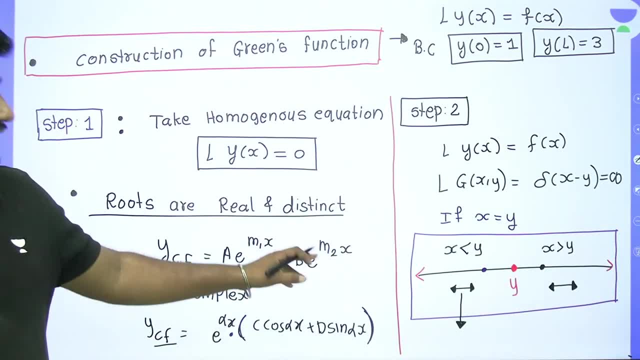 So this solution. See, This is the solution Now here in both regions. I want to write the solution. Okay, So what will we do in this In both sides? So this solution. We will write the solution on this side. 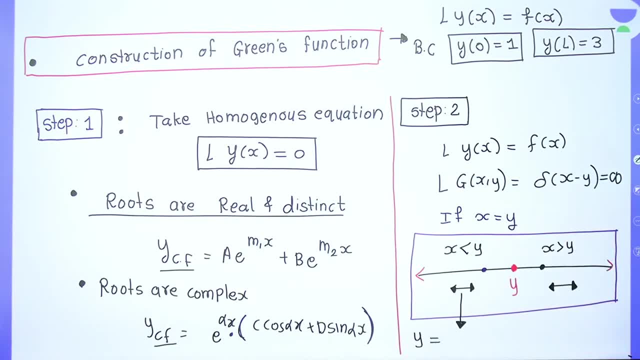 Y is equal to Now. here The form will remain the same Because your differential equation is the same. The form will remain the same. That means I am writing here What will happen? A Exponential M1x Plus. 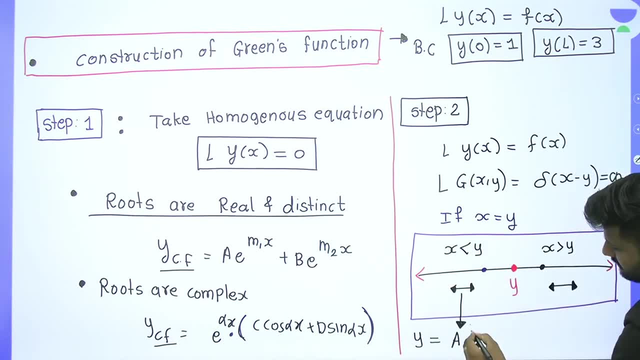 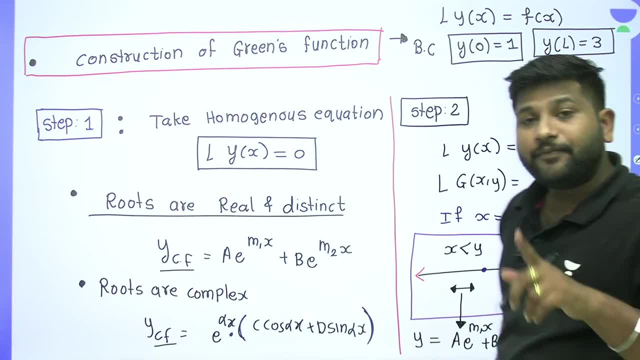 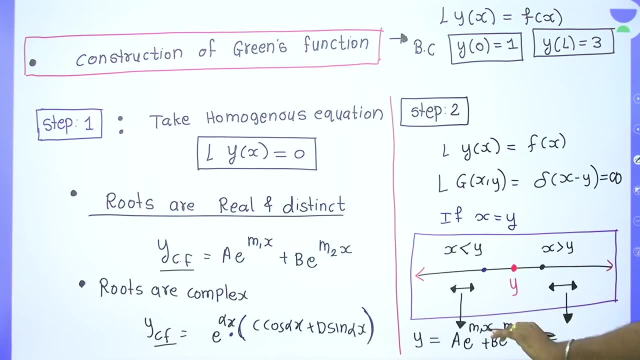 For this region, the format of the equation will be the same. Now, that is not the final solution. That's why we follow the steps. So here this will be: Y is equal to Now. everything will remain the same here. Only you have to do constant change. 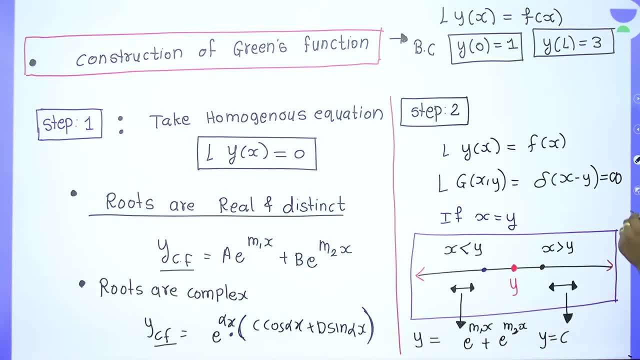 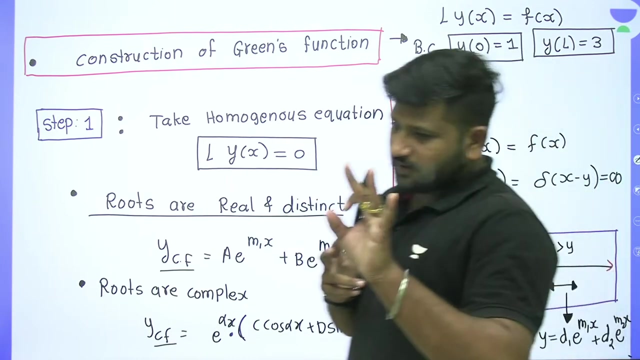 Uh, otherwise I would have changed a little constant: C1, C2, Md1D2, This would be c1- c2. so this is a d1 exponential m1 x plus d2, d2- exponential m2 x. okay, so this is here. we have changed the constant. its form will remain the same. 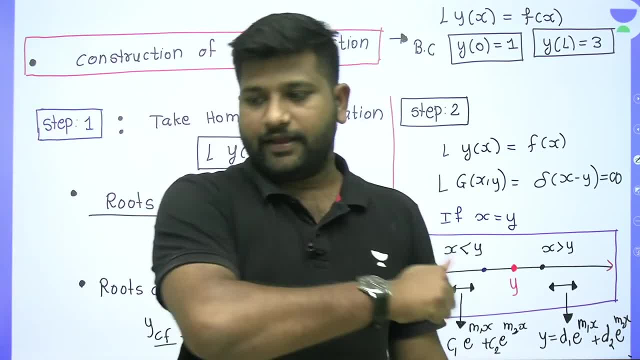 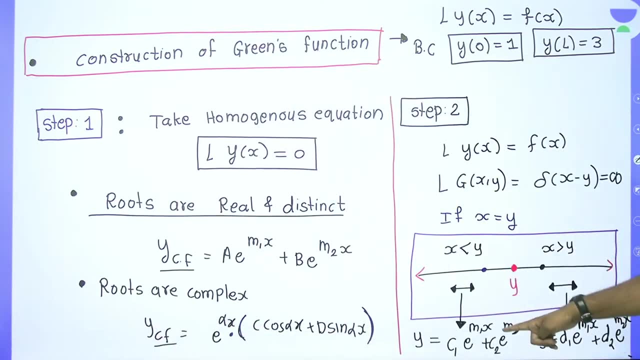 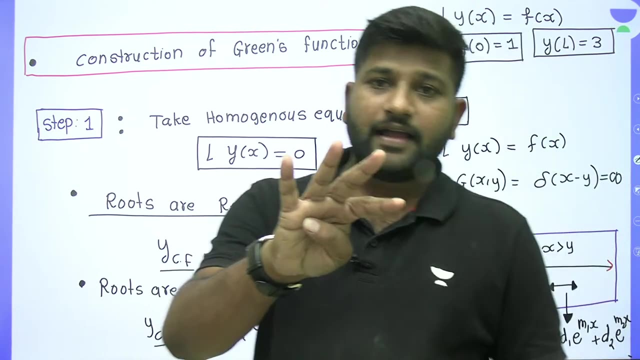 I am just telling you the steps here. if we take an example, then everything will be clear. I hope everything will be clear. you can see on left side solution and solution. on right side solution ends with c2, c1. let us take some unknowns. four unknowns are there. 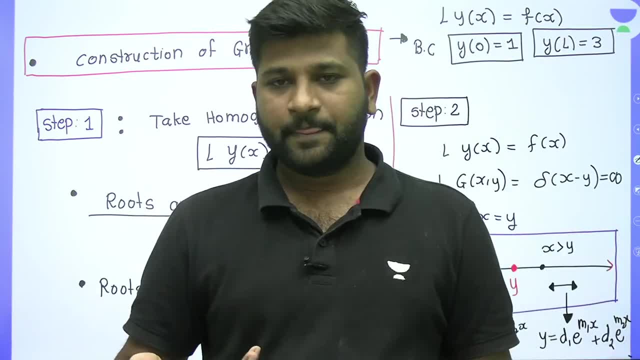 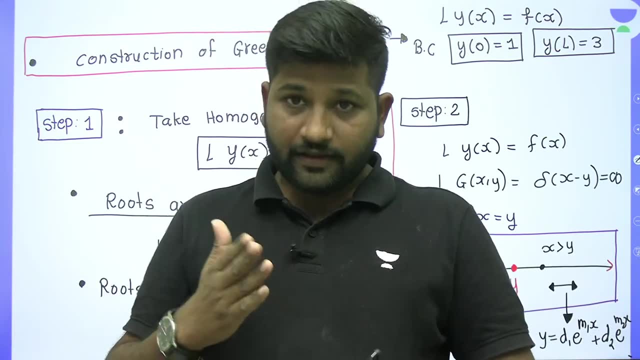 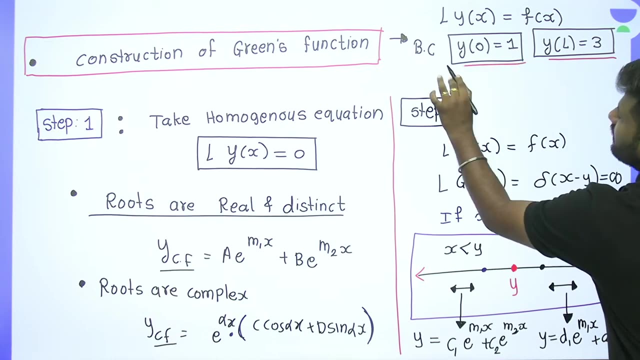 we have to find out. these are unknowns and these unknowns we have to find out. do you understand? shape is normal. a rectangle looks like this. we have to find it out. so, to find out this unknown, this boundary condition, this boundary condition will be useful to you. 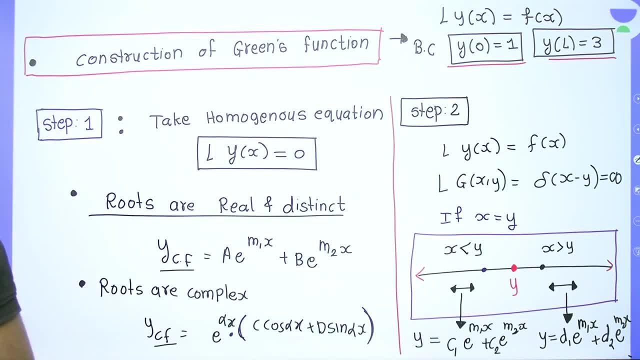 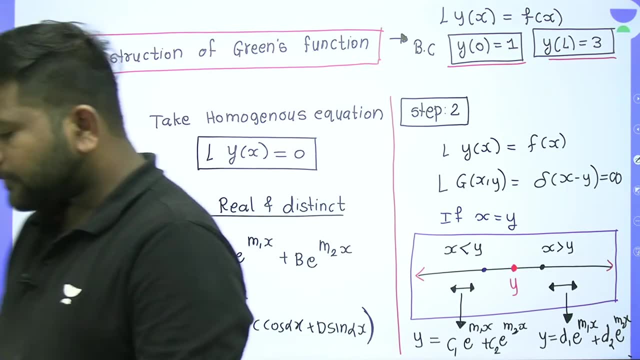 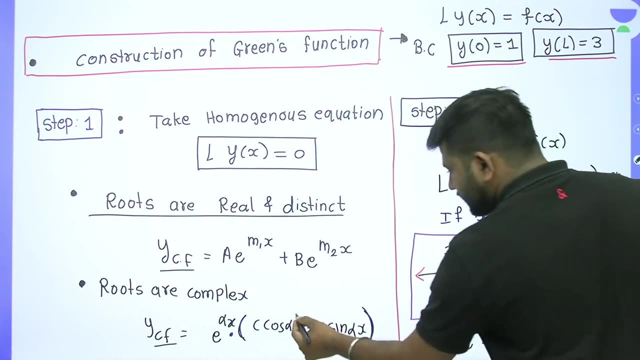 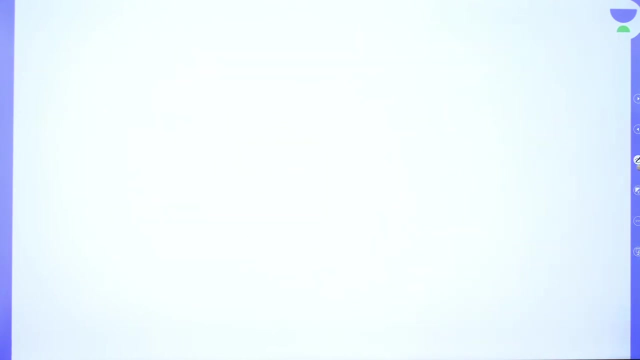 ok, this boundary condition will be useful to you, ok, ok, oh, correct, correct, this is beta, because i took real party. sorry, sorry, this is beta, beta, beta. yeah, so y is equal to alpha plus i beta. thank you, i hope you understood this. so here you have 4 unknowns. 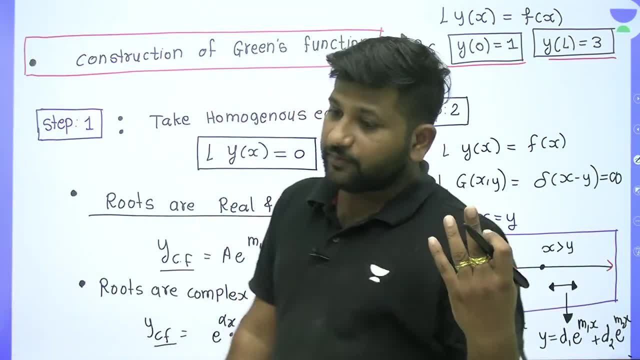 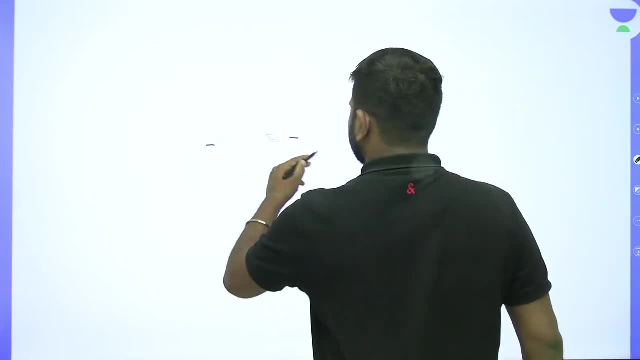 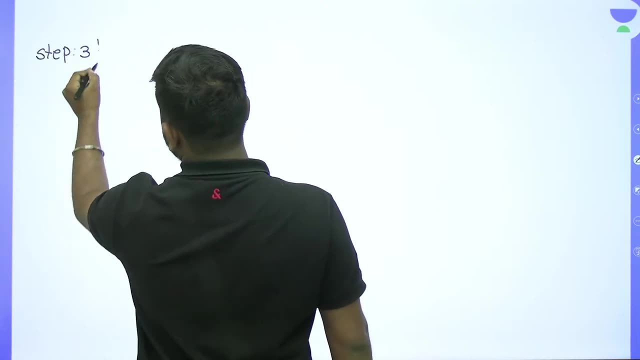 we have 4 unknowns now and we have to find out these unknowns, so you have to follow the next step. that is step number 3, step number 3. what is step 3 now? this step 3, this step 3, is that we have to find out this unknown. 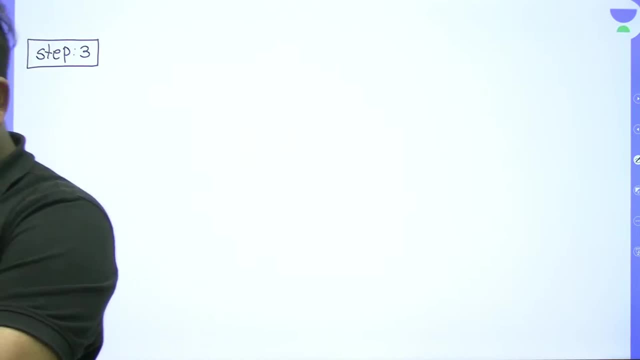 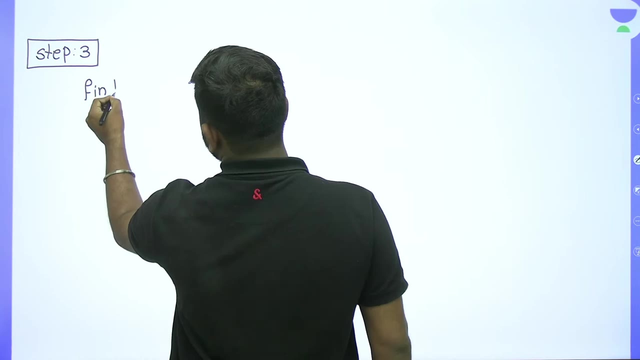 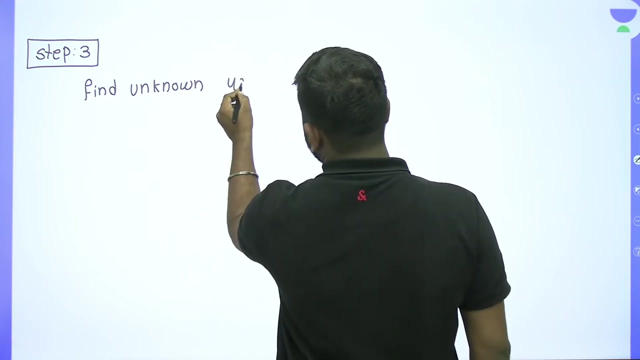 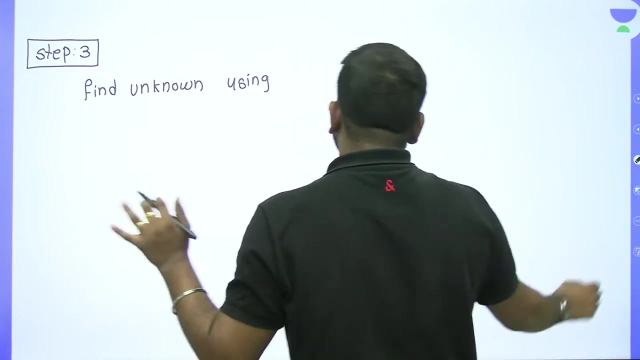 ok. so by using using the boundary conditions, find the unknown, find unknowns. now how to find out? lets discuss with an example: find unknowns using boundary conditions, using using now these boundary conditions. these boundary conditions can't take anything anywhere. this is not your simple differential equation. 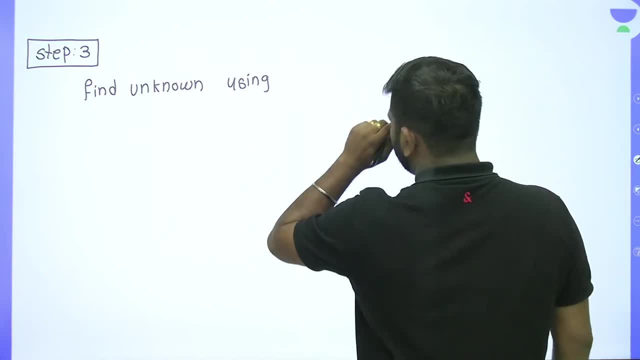 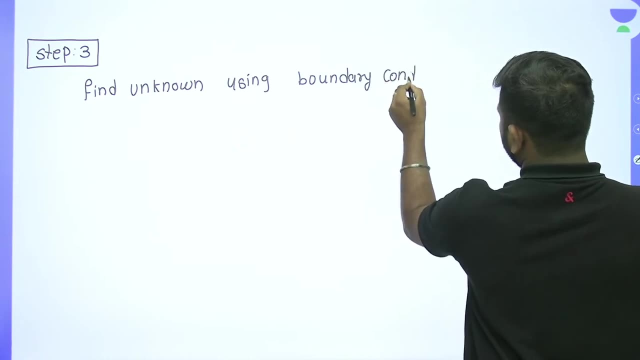 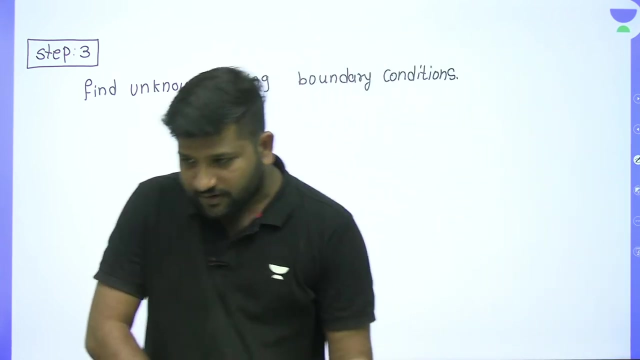 here some different things have to be done. pay attention, find unknowns using boundary conditions. using boundary conditions, so the unknowns from boundary conditions. you have to find out these unknowns. ok, now how to find them out, we will discuss. ok, this is your step number 3. 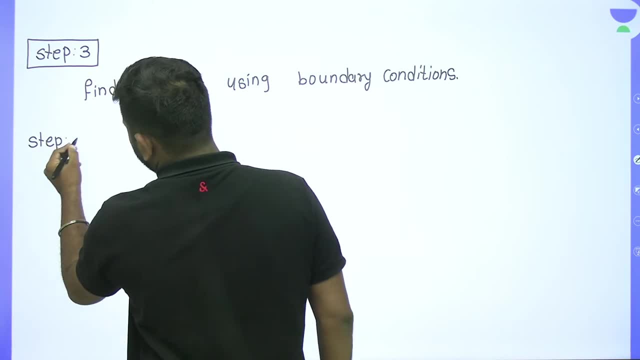 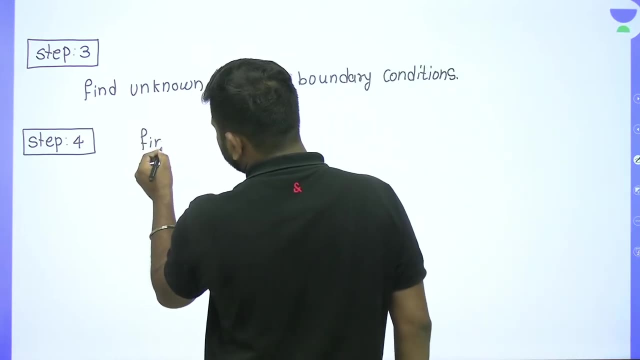 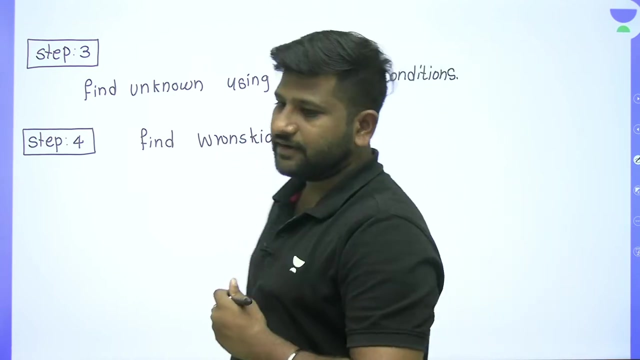 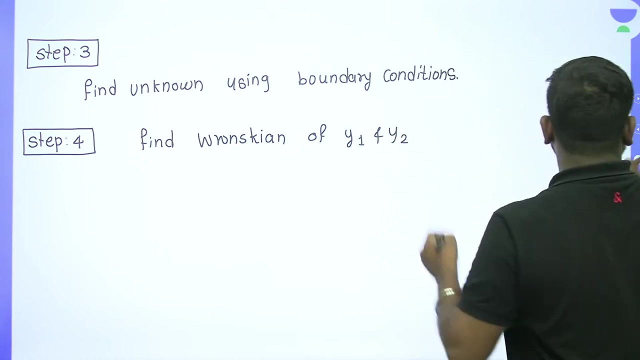 step number 3. step number 4. step number 4: find wrong skin. what is step number 4? find wrong skin. find wrong skin. whose wrong skin we have to find out? find wrong skin of y1 and y2. now, this y1 and y2 means this: 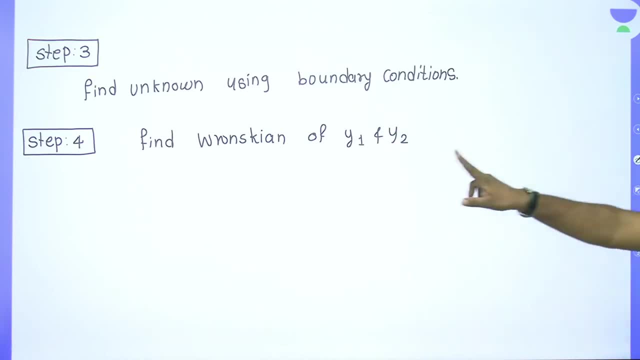 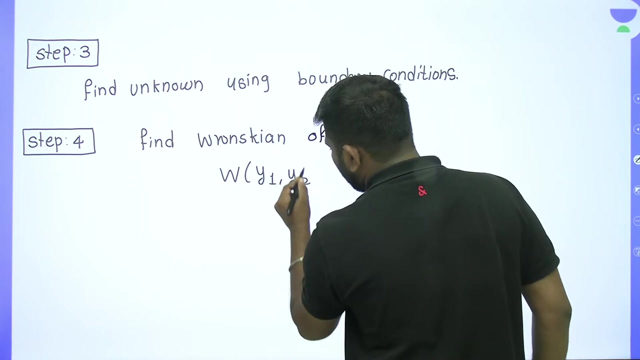 this is called y1, this is called y2, this is called y1 and y2, and you have to find the wrong skin of the same. so you have to find out the wrong skin of the same and you have to call the wrongness. now you tell which one is: the y1 and y2. 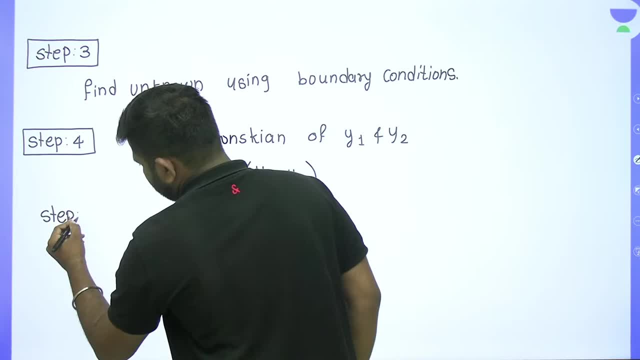 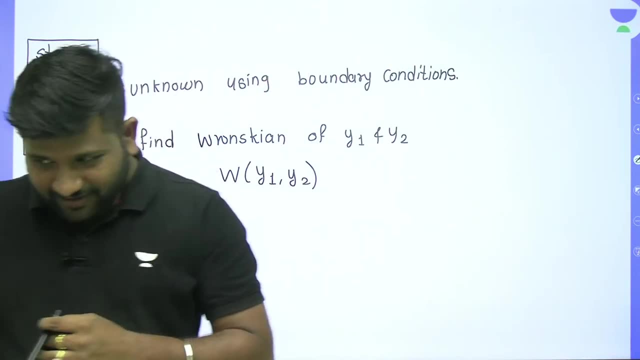 yeah, and last step. that means step number 5. I know many are confused. how to find out the wrong skin, how to find out wrong skin. maybe you don't know, but don't take tension. wrong skin is not a big thing, it is very simple. 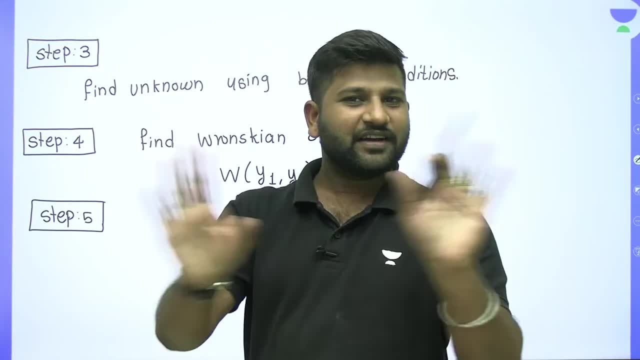 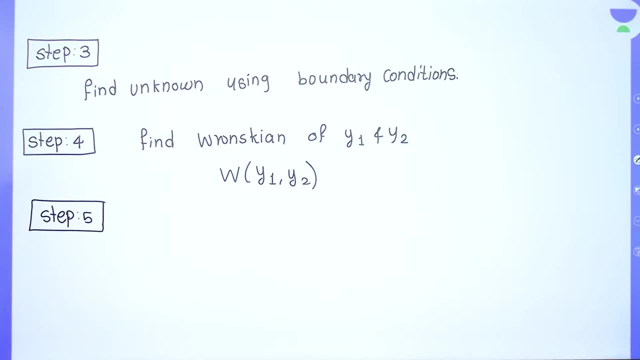 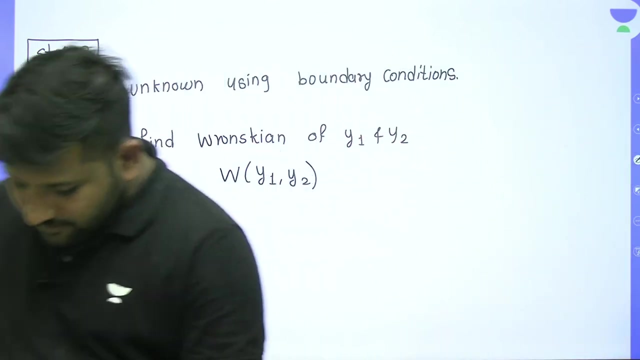 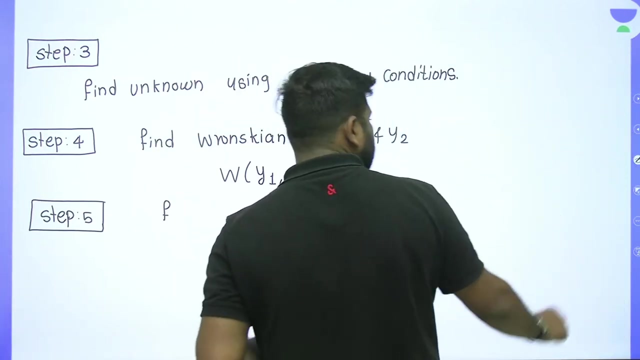 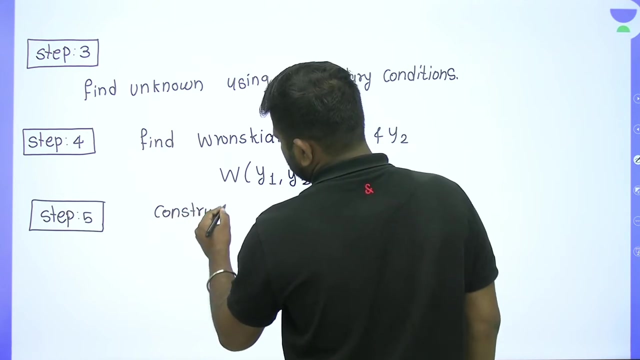 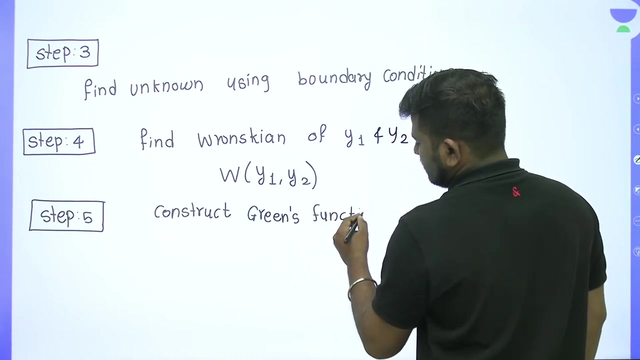 wrong skin is very easy: just determine and find out. there is nothing else in it, right? so after finding out the wrong skin, finally you can construct the greens function here and then finally construct the greens function, finally construct the greens function. these are the steps. once you understand these steps, 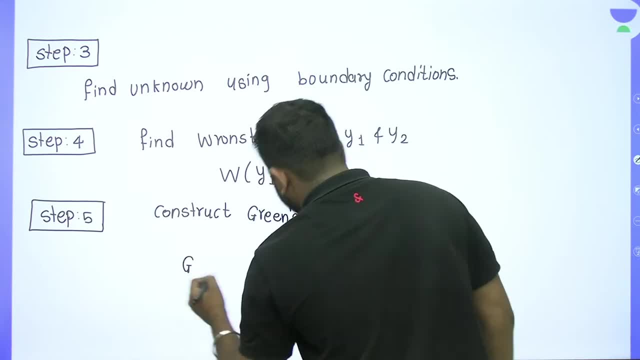 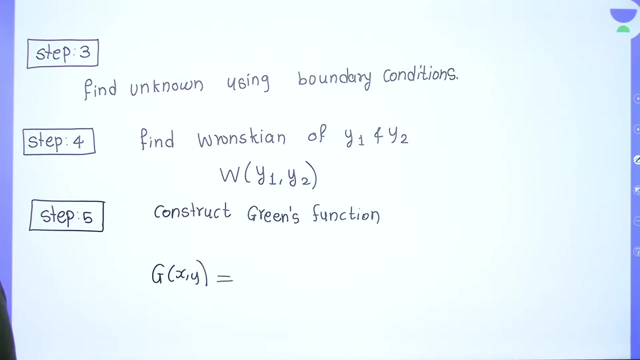 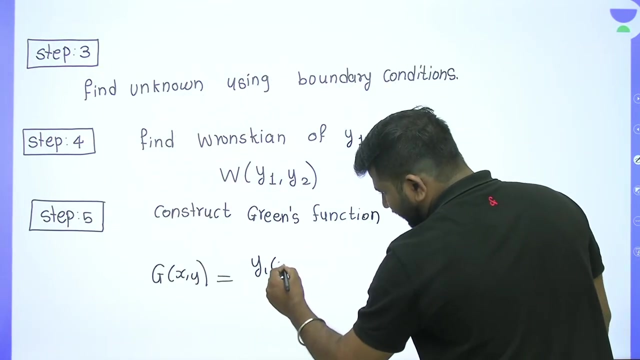 it is very easy. ok, now the greens function that you have to construct, then this functions will be g. this is the greens function, which is equal to here я paycje. it's a game of 5 minutes, why it needs just one lecture, is it? 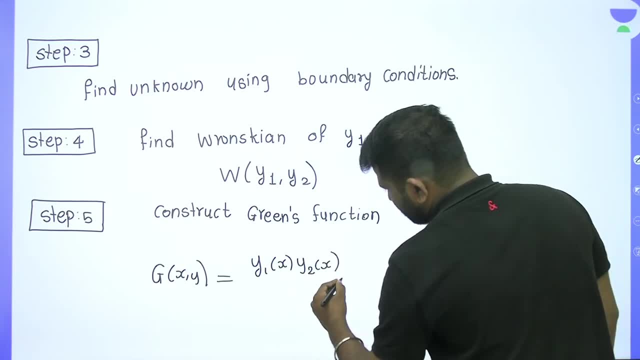 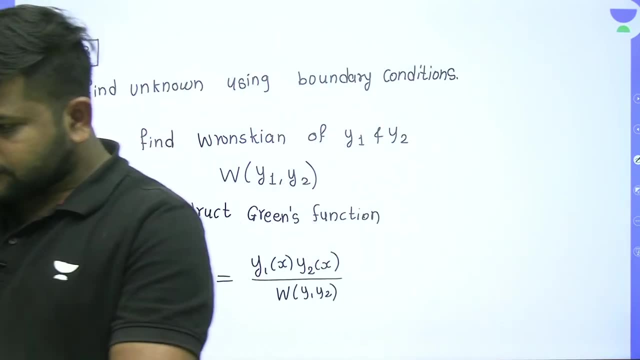 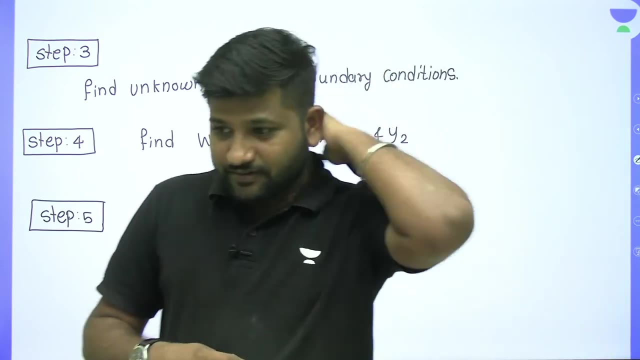 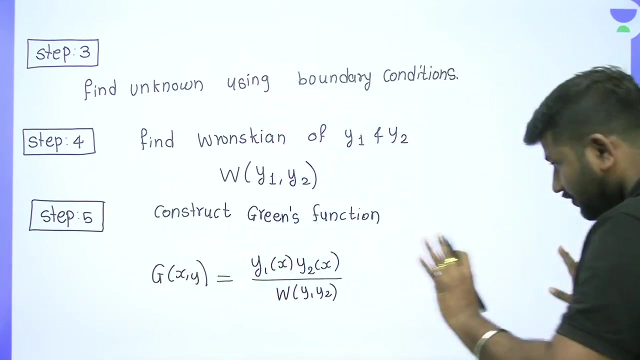 Y2 of X, Divided by Wrong scale, This is wrong scale. Ok, And Sir, this is wrong scale, but for what? For which region This is wrong scale? For what? So here This is wrong scale And here Another wrong scale, Because you have two regions here. 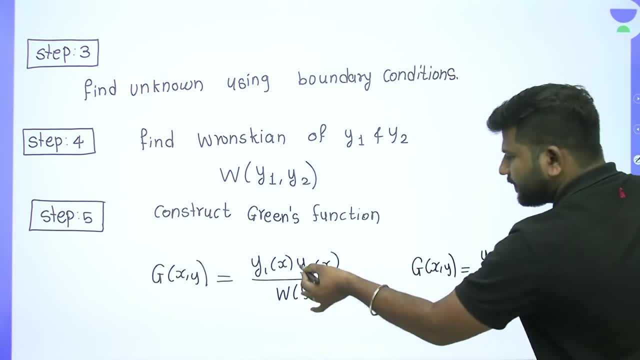 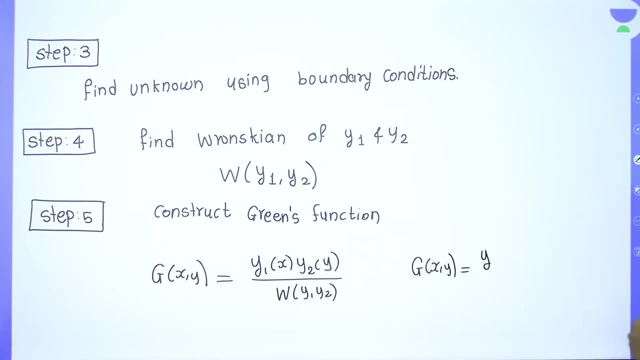 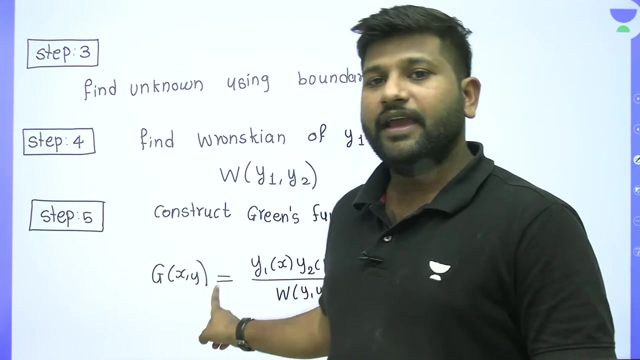 So this will be Y1 of X. Y2 of Y. This is Y- Y. This is the Y1 of Y, Y2 of X, Divided by wrong scale of Y1- Y2. So this will be your Green's function And this is asked in exam. 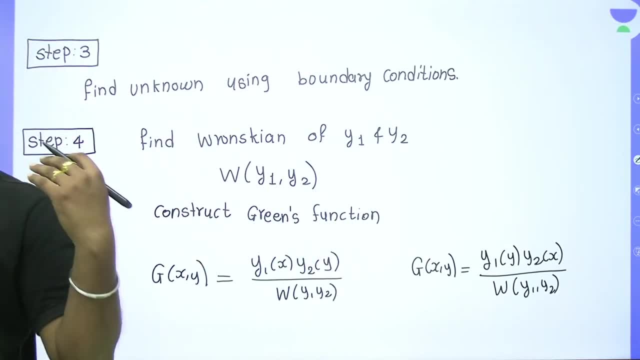 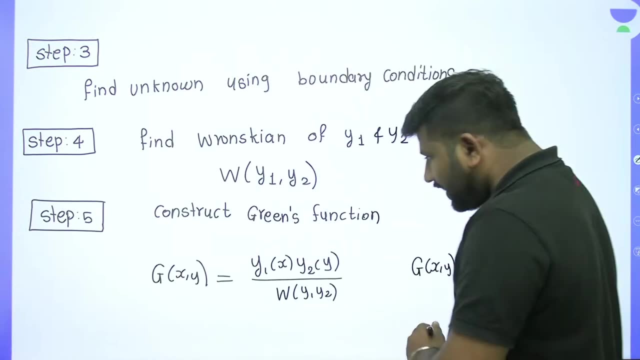 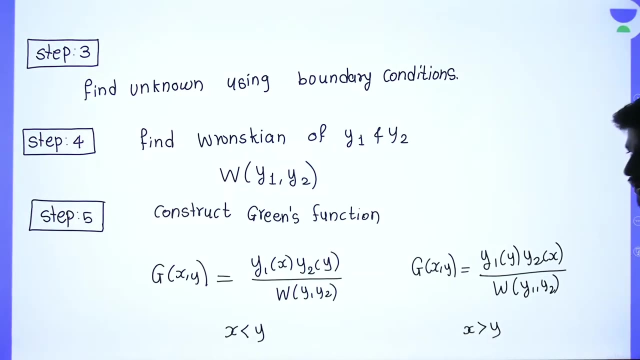 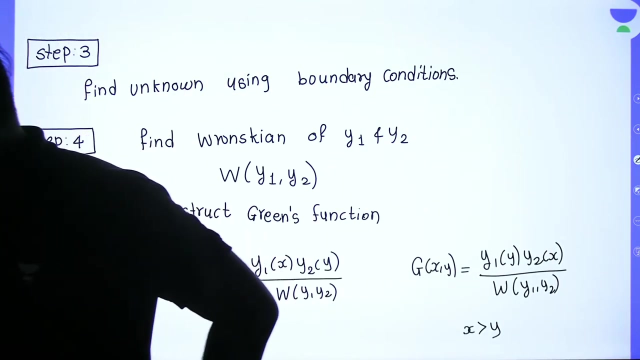 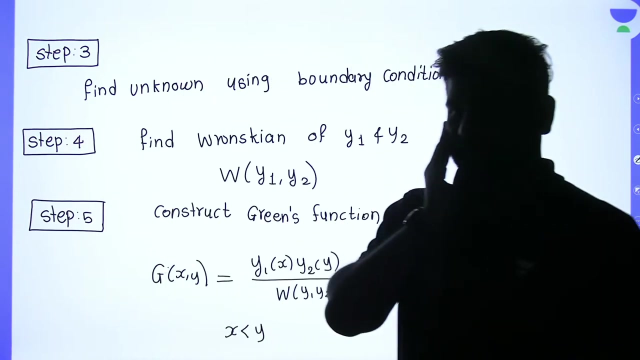 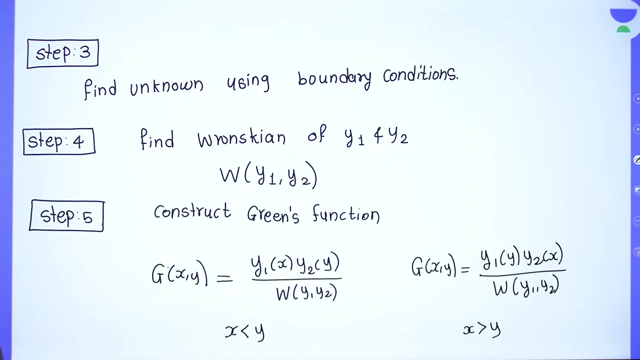 Construct the Green's function For the Given differential equation. Ok, Now, This one is for X less than Y And this one is for X greater than 1. So Light went. You can see the board. Ok, Hmm, You can see the board Now. Now it is completely black and blue. 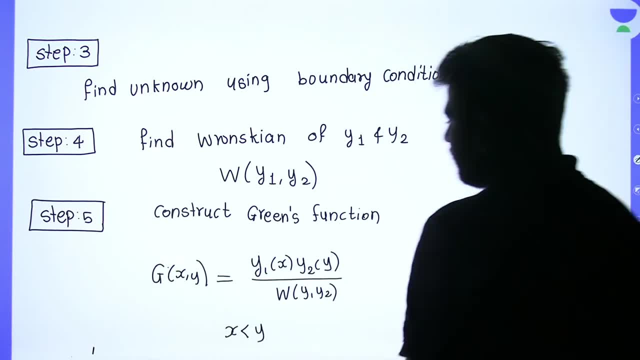 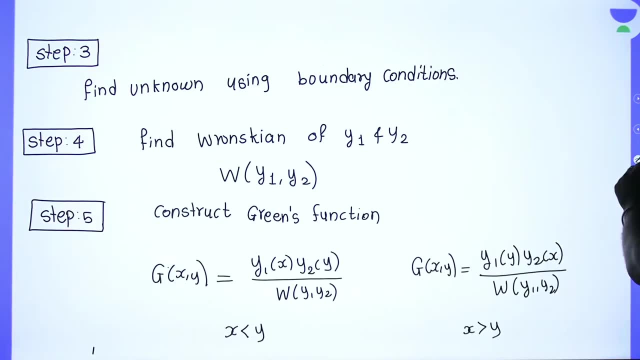 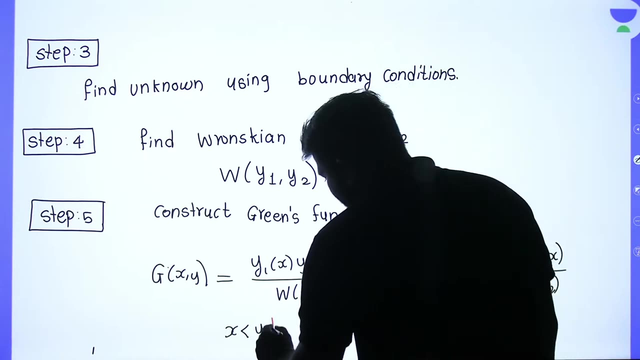 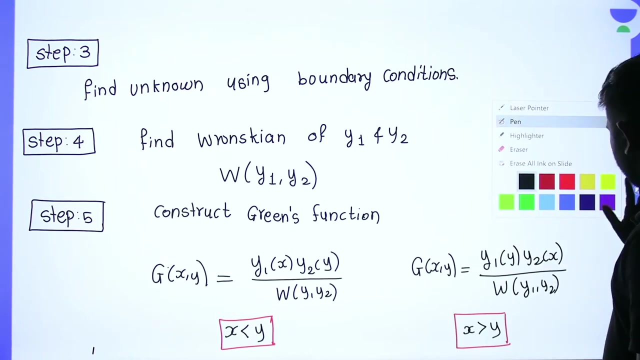 Light has gone. Ok, So this is your Wrong scale. This will be wrong scale, And this wrong scale is Now. you see here That You write this: So this will be X less than Y. This will be X greater than Y, For So you see from here That How can we remember this? 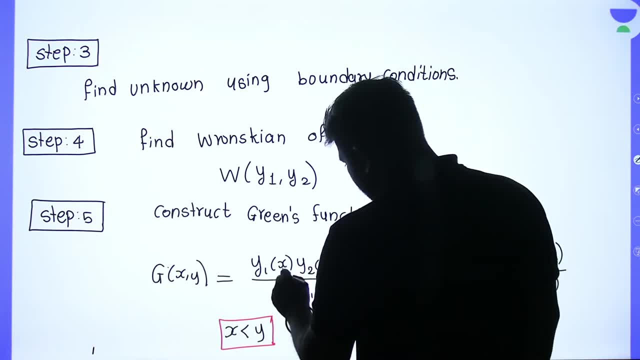 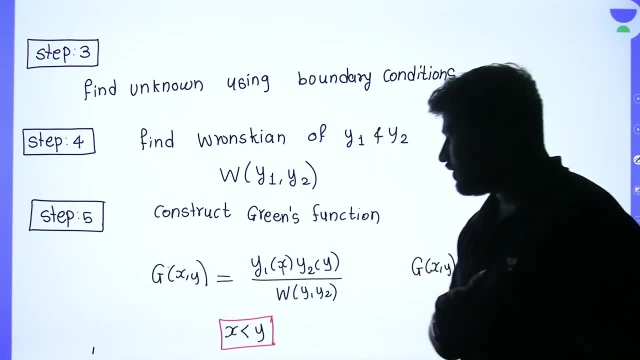 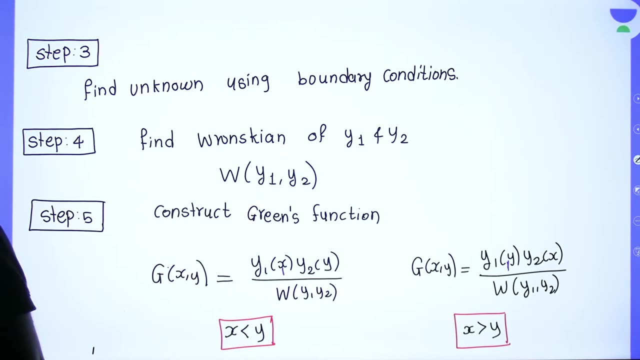 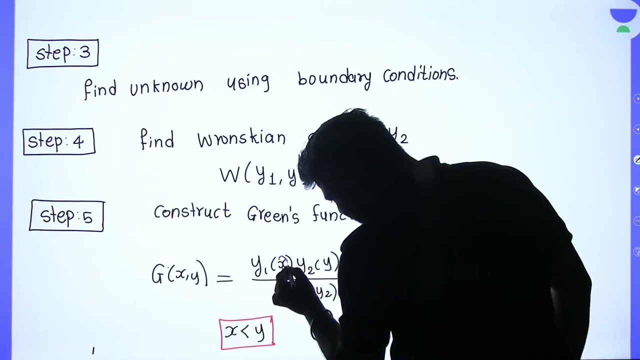 See Here, What is Here, What is If? First, If In Y1, What is It will be small. Here, What is It will be small. That's it, Ok, Ok, Ok, Ok, Ok, Ok, Ok. This is How can we remember this? What will happen in this? Right, Let's say you: 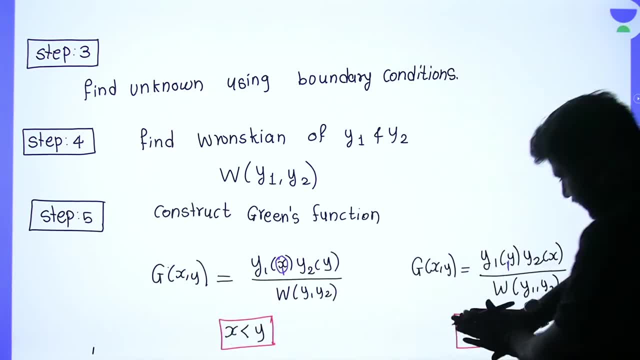 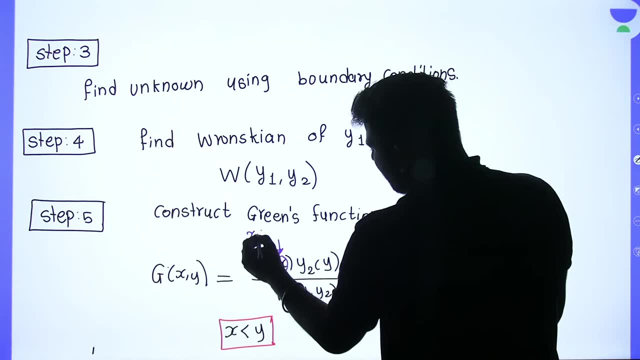 For whose reason is this? I don't know. For what reason is this? For what reason You don't know? So this will be Here When you write this. So this will be small, So it will be small Means It should be here, This one. What is inside it? 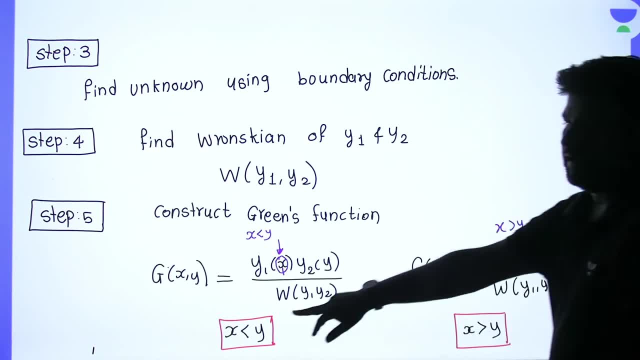 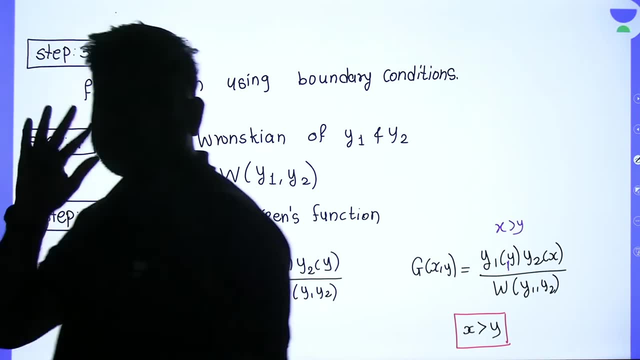 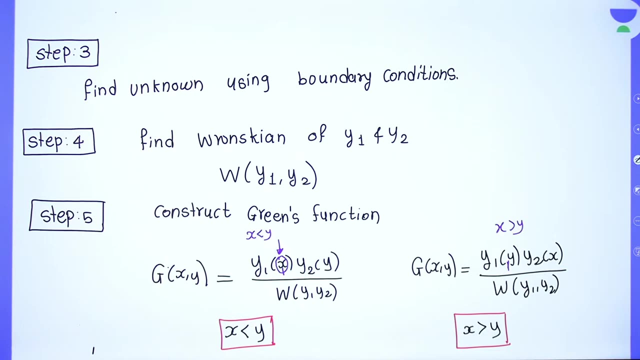 It should be small. It should be small Means. It's done. You can remember them in this way. What can you do? Ok, So I think We'll stop here, Because There is no electricity And It's not Feeling good. Wait a little. Wait for Wait, Wait for, Wait for.